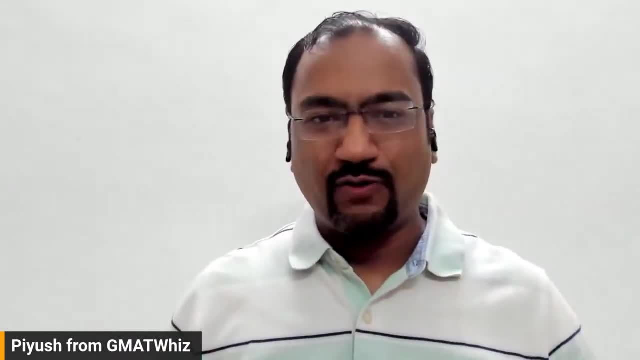 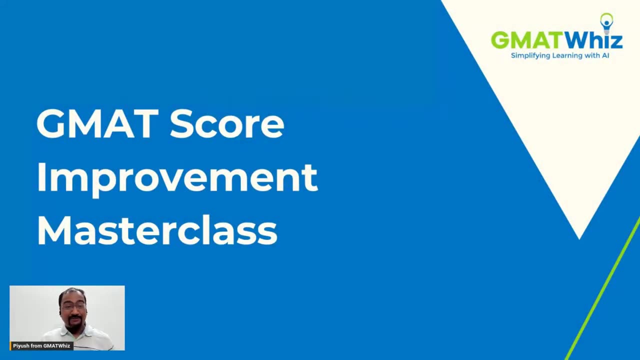 please make sure that you keep the session interactive. Ask as many questions as you want, because I love to answer your questions. So please feel free to ask me any questions and do let me know about your questions. So let's get into the GMAT score improvement masterclass today. Okay, so I told you my name. 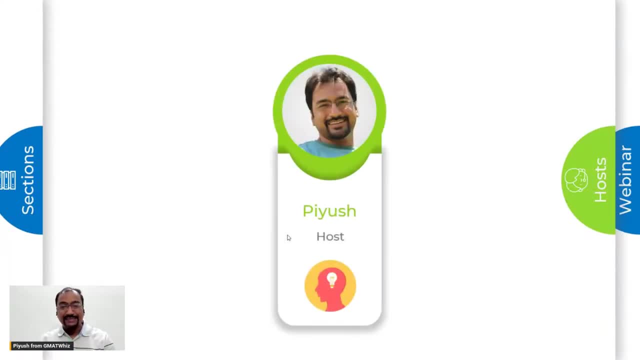 is Piyush Viriwala. Just a quick introduction. I'm a strategy consultant at GMAT, where I have taken the GMAT myself. I've prepared for the GMAT myself and I was one of the people who actually got stuck in GMAT for a long time, So I was not one of those people who were like brilliant from. 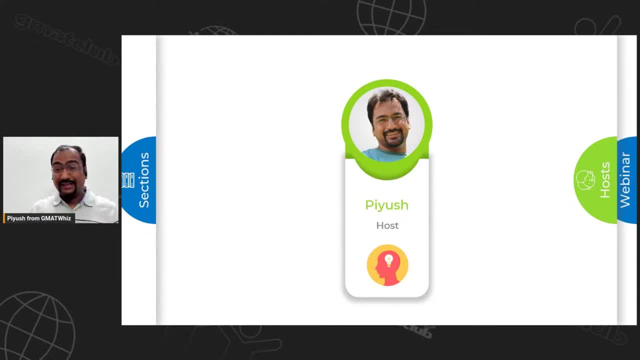 the get-go who were able to get a very good score in the first, like I, got a very good score in the first attempt. I scored a 740 in the first attempt, but my mock scores were really, really bad, even after preparing for six months. I scored a verbal 13 in my very first mock, So I was not someone who 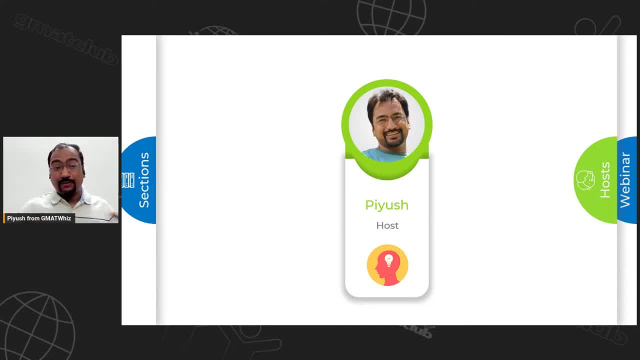 was very good in verbal initially and I had to fight my way to kind of get to a dream score of 740 on the GMAT in my first attempt. So I have close to 10 years of experience now. I have helped multiple people ace the GMAT myself through GMATWiz and we have helped people get into all 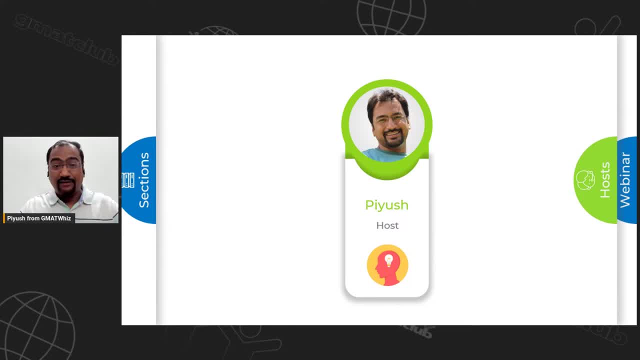 these schools that we can think of, like where is it? Harvard, Wharton, Stanford, INSEAD- You name a school. we have sent people into those schools, not just through GMAT, but also with their B-School applications. So we have been in this journey for a long, long time now. So I'm going. 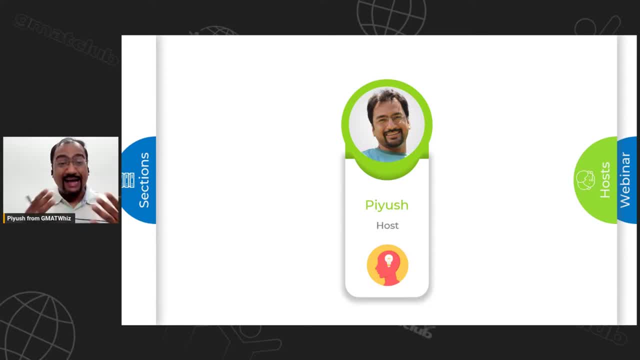 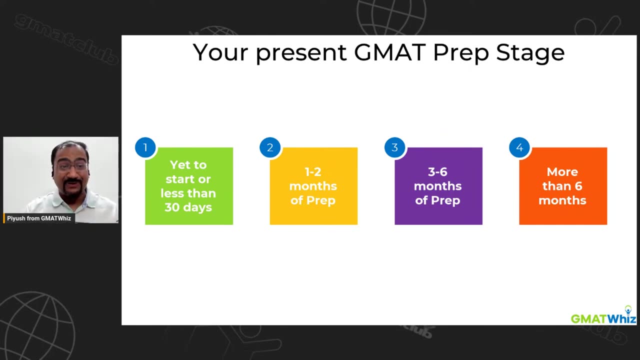 to share a lot of those unique experiences with you to help you understand how you can boost your GMAT score. So that's a quick intro about myself. If anyone of you wants to talk to me, I'll share more about you guys because, again, the session is about you, right? The session is about your score. 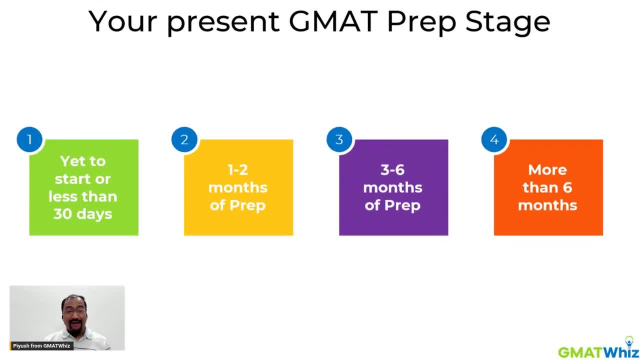 improvement. So I would love to know more about you. So I have given four categories. I want to understand what stage of GMAT preparation are you currently, So I can actually face the session in that way. I want to understand overall what is the sample size that you are looking at today? 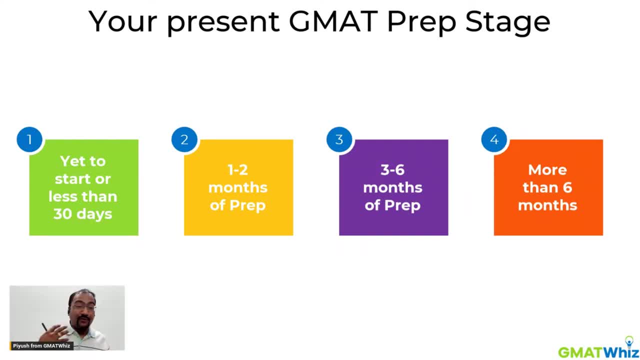 What are like? What is the distribution of people? How many of you are new to GMAT? If you are in category one that you're just started your preparation or you're you're prepared for less than 30 days, just mention one. that will be enough. if you are in the second category, where you have 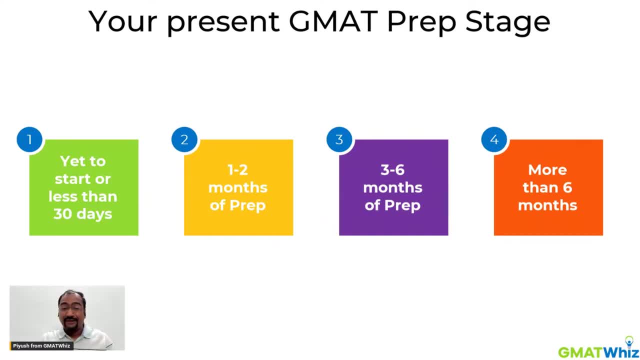 done one to two months of breath, mention two in your thought like message. if it is three to six months, then mention three and so on. so just put up your thoughts so, uh. so mr says i am someone who has been preparing for more than six months. okay, uh, so i'm. i'm understanding, so, mr, that you are. 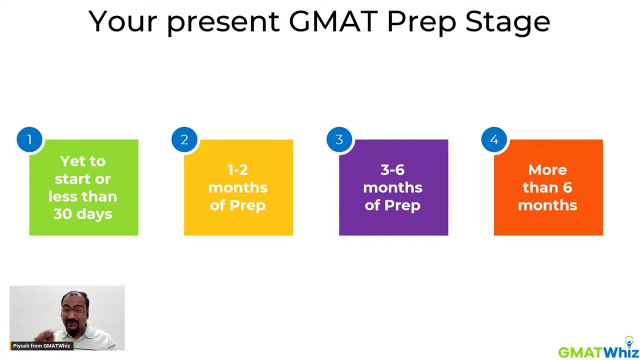 having some issues with your verbal, like gmat score improvement, so don't worry, you're in the right place. we're gonna talk about what kind of leads to score plateaus and how do you overcome those four plateaus in gmat. basically, isaac says i'm at category two, doodler is also in category. 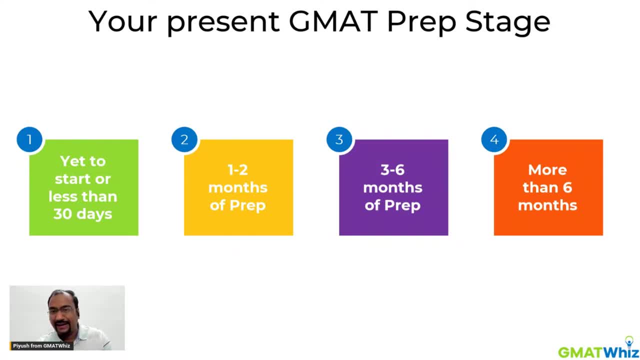 two. so one to two months of preparation, and there are a lot of people in category one. right, i see, uh, dewey, nelson, shireen and barish in category one. so you have yet to start again for who? for those of you who are yet to start as well, you will learn a lot about. 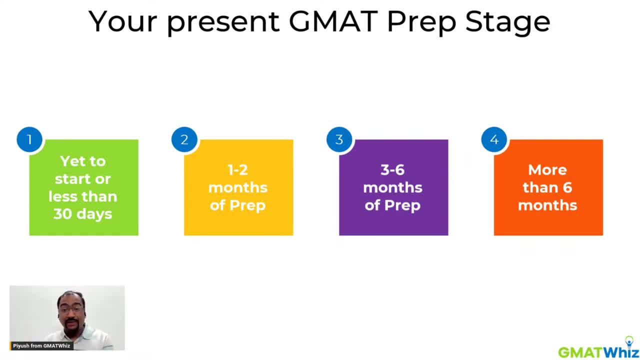 how to start your preparation also, and what are the mistakes that you have to make in order to be able to start your preparation, and what are the mistakes that people make because of which they get stuck at a particular score, and how do you avoid those mistakes? and i only see one person, gargi, who says: i am in category three. i have three to six months of. 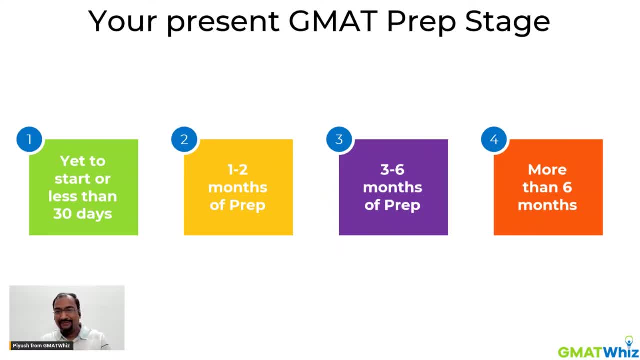 gmat prep experience. okay, so most of you i see in category one, which is uh there, uh like, which is the case with like. generally most of the sessions i see a lot of people who are in the beginning phases of the preparation. but even if you are in any of these categories, you're going to learn a. 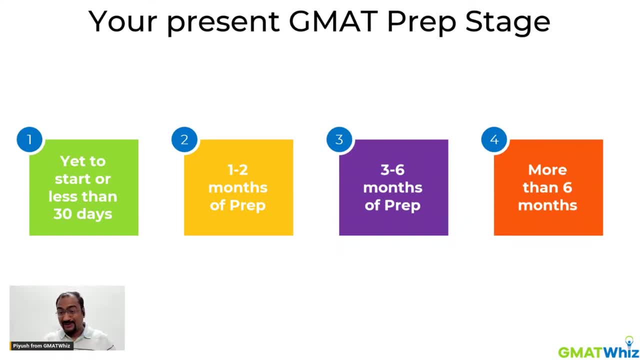 lot about how to improve your gmat score and take it to the next level. okay, so mr says i'm also in category three. the gargi is not alone. okay, that's great to know. okay, so let's get started. so what i usually do is i present an overview of the entire session to start with, so that you have an idea. 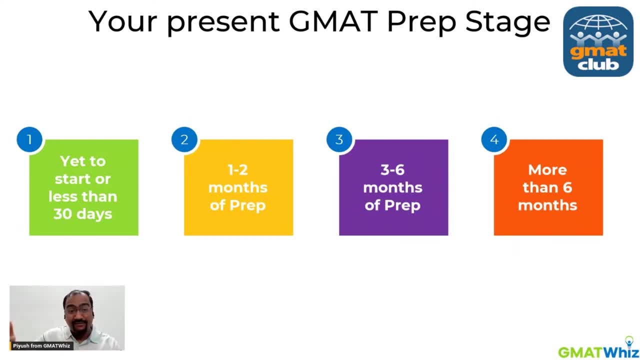 about how the session is going to be structured and then we deep dive into each of the areas, basically for for that. so julie had a question. she was saying: what is the average time required to ace a good gmat score? so, julie again, a good gmat score is a very subjective thing for someone. 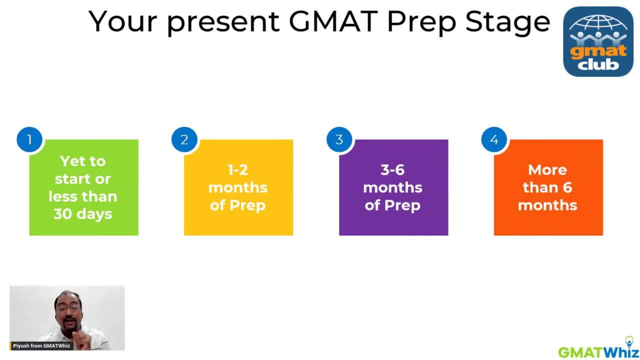 650 is good, for someone 670 is good, or someone has 700 is good. so i'll say, if you want to get a 700 plus on gmat, an average time for the average student would be about two to three months, basically okay. now we have had students who have prepared for gmat for 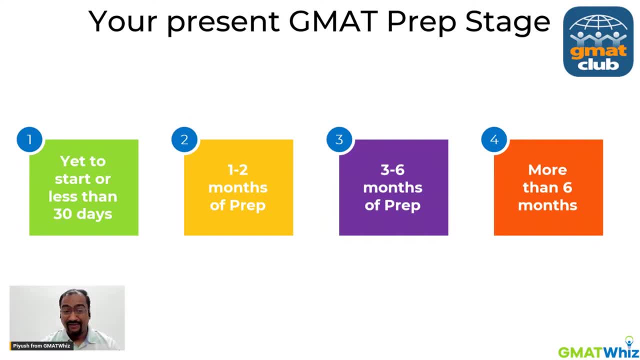 just a couple of months and scored a 770 in their first attempt as well. so we have students like those also, and in case you want to uh watch the uh detailed interview of that student, i'm just sharing the link here in the chat so you can go to it, julie, and check it out. so this is the link. 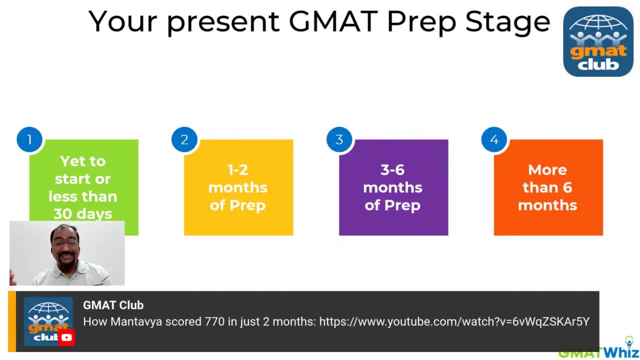 this guy's name is mantha. there he did an amazing job and was able to get a 700 plus on gmat score, to crack 770 in just two months, okay. so again, those cases also exist, but if you're an average student, approximately two to three months will be required for 700 plus, okay. so if you want more, 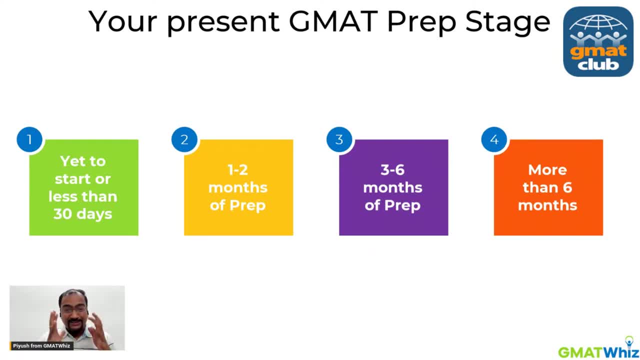 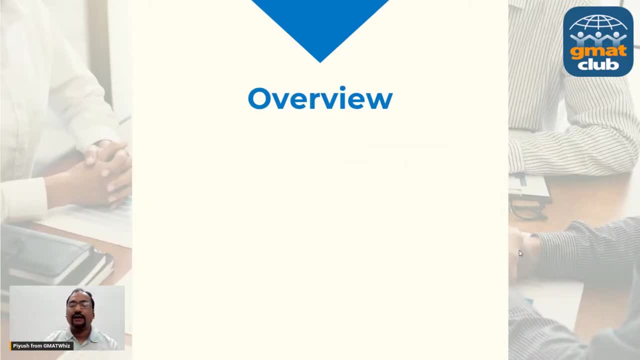 tips. you can always go to mantha's interview and check it out. all right, so let's get going with the session. i'll help you understand how i have structured the session, so what, what we are going to cover and the most important tip: like to help you improve your gmat score. 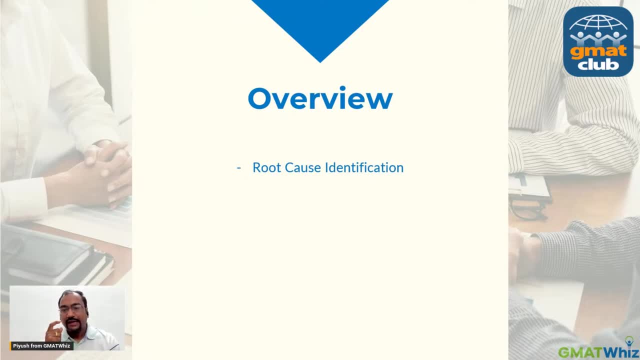 is basically to identify the right root cause, because when i actually speak to students- and just to give you an idea, guys- i speak to at least five to six new students every single day. so you can think about, i guess, thousands of students every single year, right? so in my career i've spoken to tens of thousands of people till now. when i speak to them, 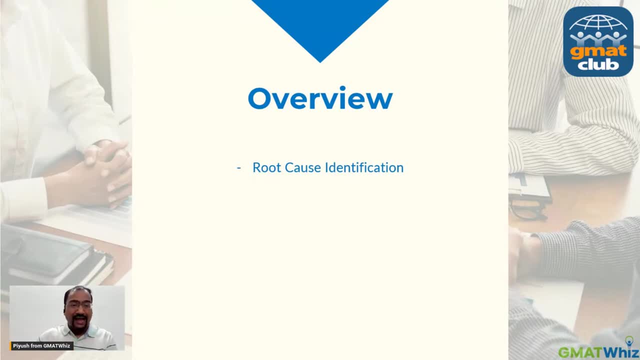 i understand from them that they don't even know what is the root cause to their actual problem. most of them think that it is timing: they are not able to solve questions in the right amount of time. many of them think that it is specific to specific areas. because of that, 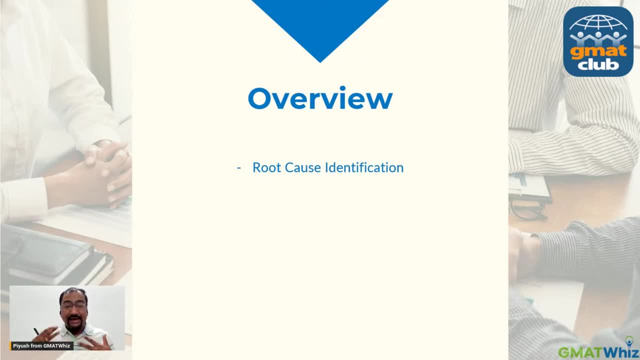 some people think it's just because the questions on the gmat and on the day of the test, they are feeling more anxious. it's about anxiety, but in reality, what is the root cause? that's what people don't understand and i'm going to spend almost half of my time today- almost half i'm not saying. 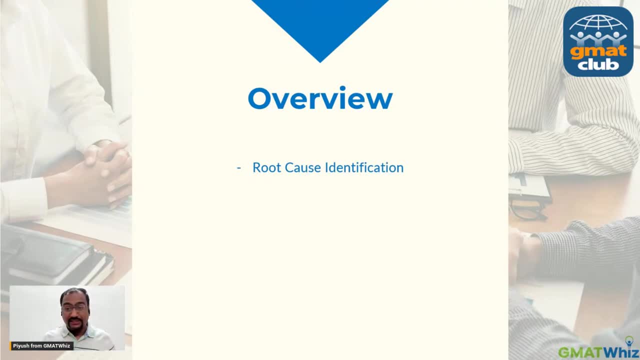 exactly how. almost half of the time today on this root cause identification, because i personally believe that if you get the identify the root cause correctly, it is very easy to solve the problem. the main problem is identifying the root cause. then we are going to go and talk about the solution. i'm not going to just leave you with the root cause. i'm going to provide. 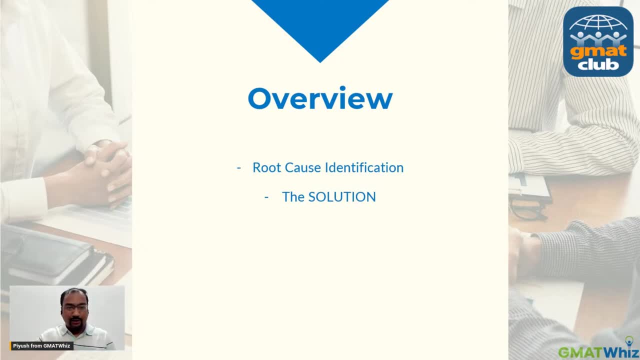 you a solution also that how do you solve the score plateau problem that you are replacing right now? and then we are going to talk about the important, very important tip, which is to review the solutions closely now. this is something which very few people understand and do in reality, and this is 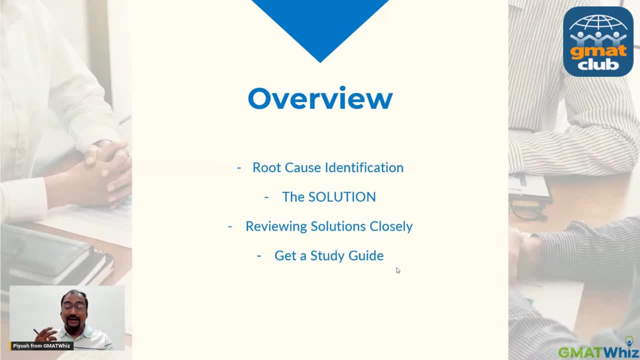 a very big game changer. then we will dive into uh and uh- the importance of getting a study guide- being having someone who can actually guide you in the right direction- and then they will focus on one more tip, which is focused fine-tuning. again, i know you are thinking i'm going to cover a lot right in the session, but i'll try to wrap this up in 60. 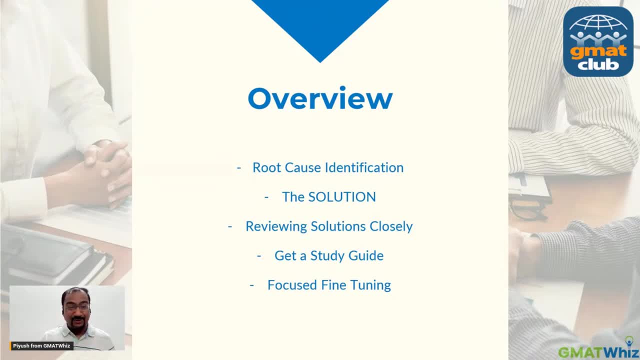 to 70 minutes. that's my target, but yeah, please keep the interaction going on. that's what will make this entire discussion very, very healthy, and in the end, i'll also talk about anxiety management. so, overall, i'm going to talk about the six steps which will help you improve your school. the first: 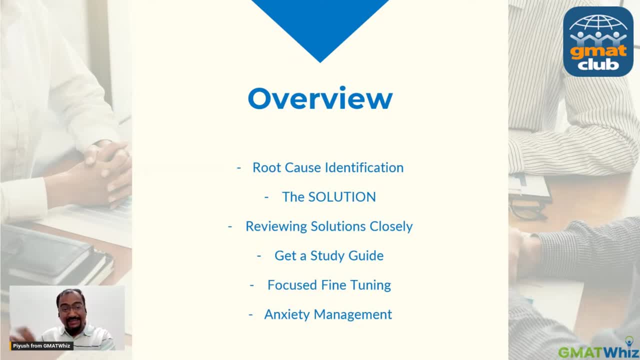 three are very closely linked to each other, so you might not see the transitions, life spot work, the, but all three will happen and come in the same order. so what are we waiting for? let's get started. so what is the root cause of all the problems that people face? why do people get stuck with their g? 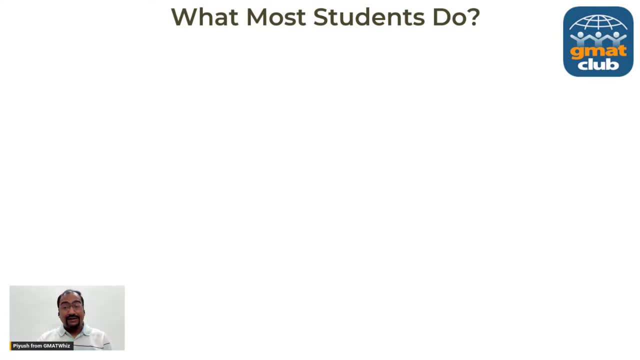 max code. now, before i come to that, i'll ask, i want to understand from you- those of you who have been preparing for one month or more, so people who are in category two, three or four- what are you doing today to actually improve your gmat score? what is that you are doing today to improve your gmat? 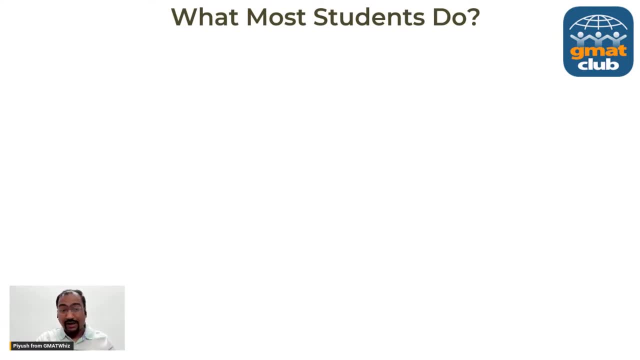 score. i would like to hear from you. let's, let's see what you guys are doing today. okay, and guys, uh, do continue giving this video a like if you really like the content being delivered. i have a target of getting to 50 likes today, so let's see if we can achieve that and we'll be back. 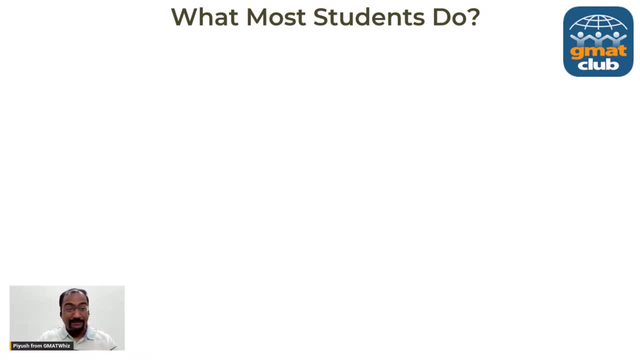 again, who knows, in another a couple of weeks, uh, discussing another important, uh like topic with you guys on the same channel. so, yes, keep the likes going if you really like the, the content, and i will see you in the next video. bye, but let me know what is that you guys are doing? basically, i want to understand from you that what 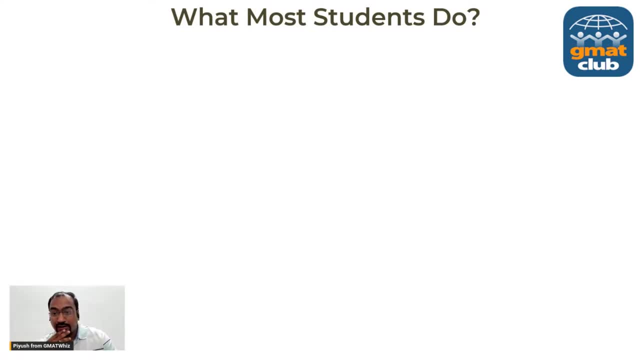 is your approach to improve your gmat score? okay, nishita says only practice, practice and practice, so she has focused on the word practice size. so that's a very common uh like approach which a lot of people follow. so thank you so much for commenting. uh, what about others? okay, although. 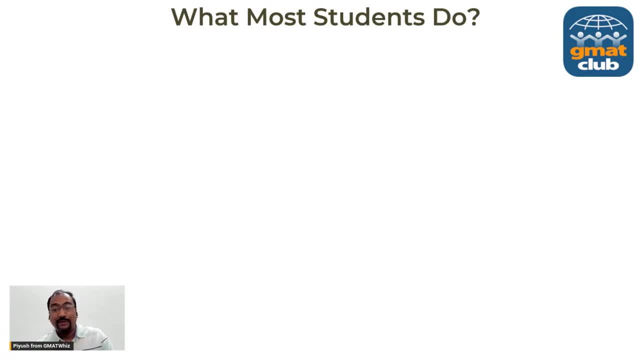 i'm from category one, but i have heard people maintaining error logs to keep a track of mistakes and i see that it is mostly useful for doing a lot of research, and so i have developed a lot of content because of that. but then can i do more work on how to do more work to improve my 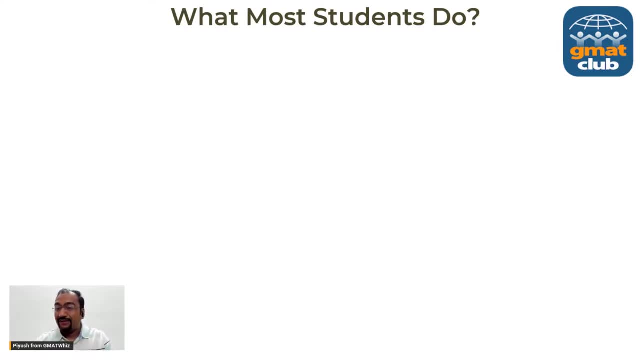 skills and i have done more research on my skills and i have done several research on my skills and i have done some research on my skills and i have done a lot of research on how to do better at gmat. so an initial phase of my preparation. so what i learned from that is actually error logs. 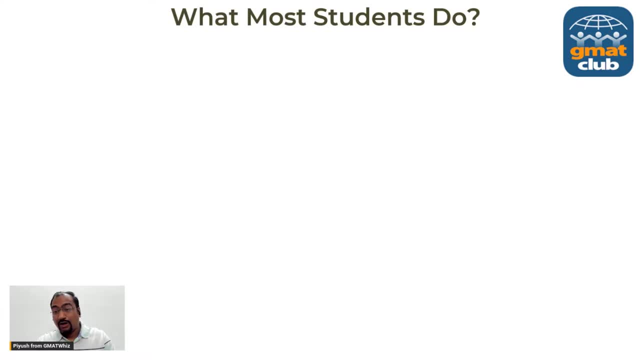 really, really helped you a lot, so that's a very good point you made. we're still learning the concept and using examples to understand the concepts i learned. so isaac says: i'm going to start the initial phase of the preparation. that's, that's understood. gargi says: giving mocks and. 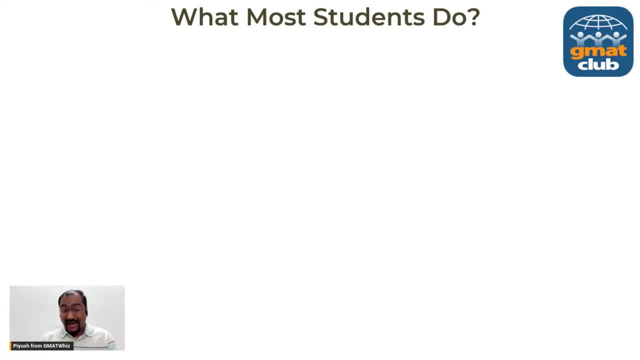 that's understood. gargi says giving mocks and analyzing my responses. okay, another important does make sense. i do agree that practice is definitely important, but how much and how is something that i'm going to discuss. so thank you so much guys. thank you so much joey isaac, nishta, gargi, all of you doodler as well, for the responses that you gave and let's 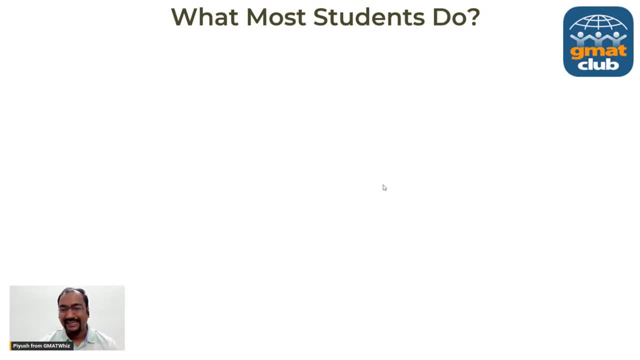 keep the responses going. i would love to see your thoughts at every stage. so what most students do when it comes to score improvement, the. the main thought process is that okay, let's practice questions. okay. the main thought process is: okay. if i practice makes a man perfect, so the more i. 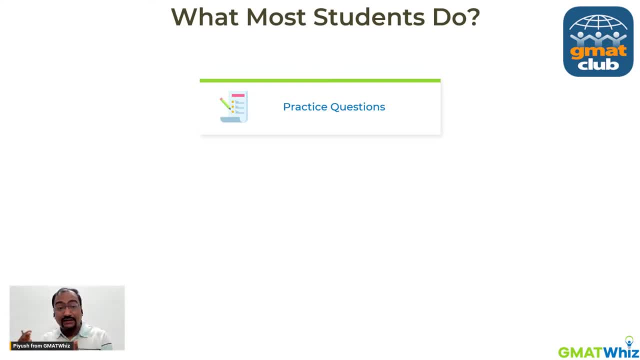 practice, the better i get, but that's something, uh, which may or may not help. if you are doing that alone. okay, guided practice: focus practice is the key, not just practicing. and, uh, many people just focus on taking marks. that, okay, i've done the curriculum. i have understood the 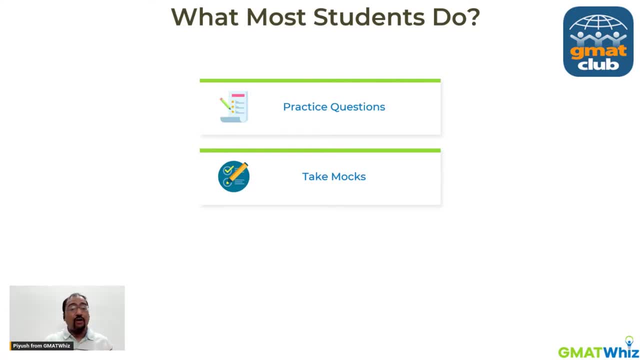 concepts. i have done enough number of questions. i have solved the official guide. now my time is to take marks and analyze the marks and improve from there. and then some set of people also work on, uh, the concept building part. that okay, let me work on the concepts in which i am weak. so they maintain their level of work on the concept. but 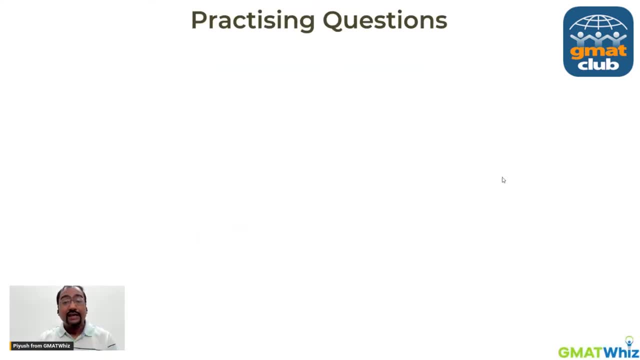 in many cases, i've seen people not improving even after all of this. the main problem with that is that when you are practicing questions, you are just focusing on practicing questions is definitely helpful, but if your score is still not improving, if your score is still not improving even after practicing more questions, like i spoke to a person today, 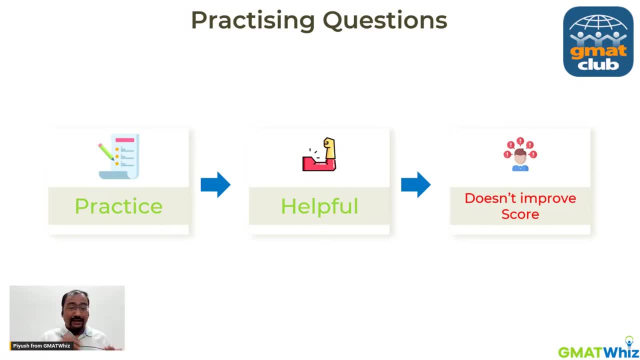 uh, in the afternoon, this guy told me that i completed a certain course. i scored a verbal 28 in a mock test. then i started doing more practice. i practiced for two more months on my own and even then, after those two more months, i was still stuck at a verbal 28.. now, why did this happen? like you, 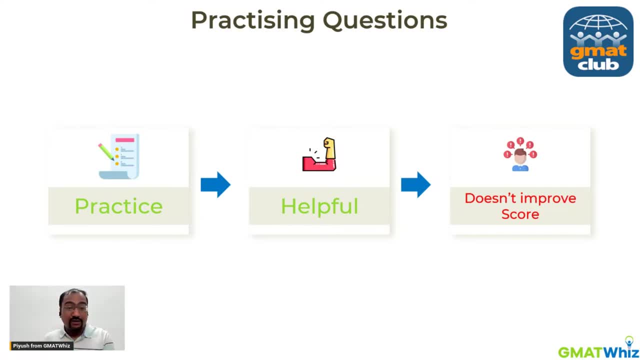 practiced. it's just supposed to be helpful, but it does not. did not improve your score. now why does that happen? that happens if you're practicing using the wrong methods. practicing helps when your methods of practicing or your method of solving a particular question is perfect. if your method. 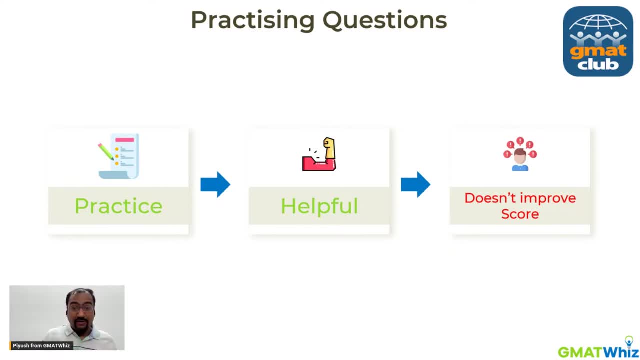 is perfect, the more you practice, the better you get. but if your method is not perfect, if method is wrong, then the more you practice you'll only get better at using the wrong method, and that doesn't lead to a significant improvement in your score. so before you move to practice, you also need 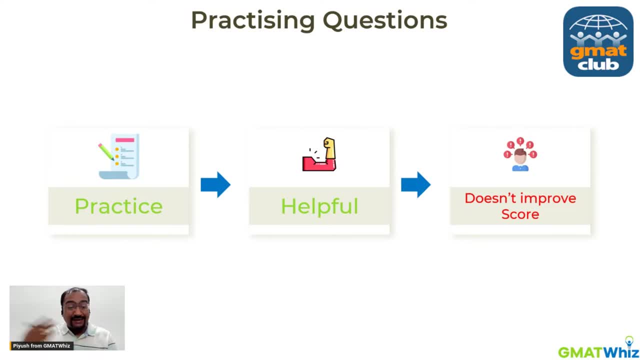 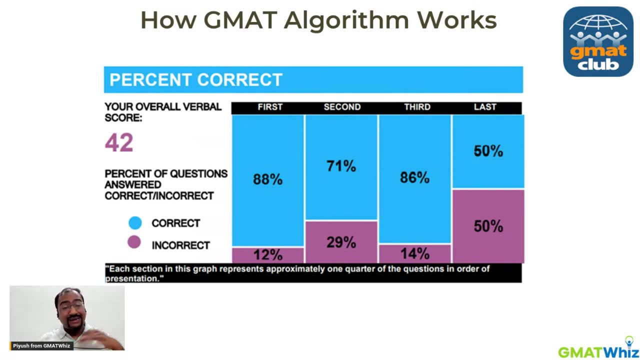 to understand what the gmat really tests you on, what is the gmat really required. and i'm going to focus a little, a little more on that particular part, because what i see is that most people don't even understand how the gmat function, how the gmat algorithm works. so if you look at this, 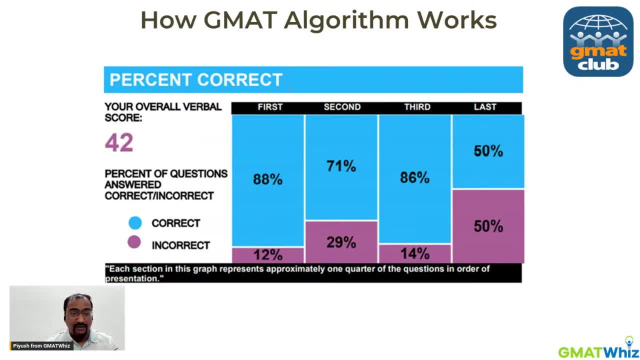 esr on your screen. this is a enhanced scorecard which is provided by gmat. this is for one of our students who scored a 760 on the gmat with a verbal score of 42. okay, so this is the verbal snapshot of that particular student. now what it shows is the number of mistakes or the percentage. 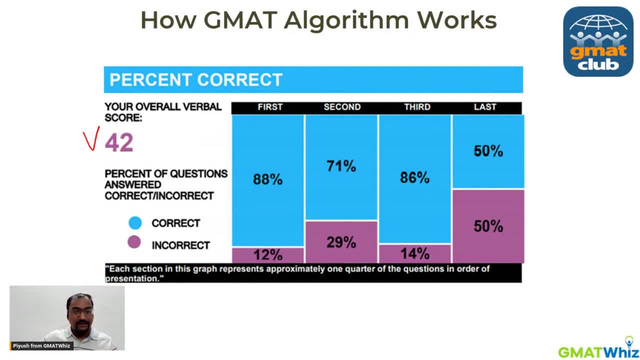 of mistakes made by the student in verbal in each of the four quarters. so the total number of mistakes made by the student is eight and he made one mistake in the first quarter- sorry- two mistakes in the second quarter, one in the third quarter and four mistakes in the last. 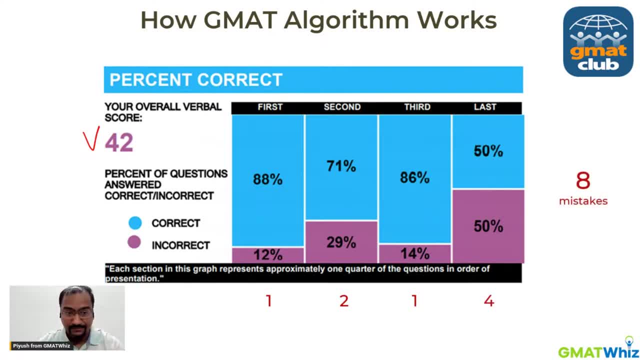 quarter. so total number of mistakes made by the student was eight. okay, now try to register this on your mind. okay, eight mistakes. he scores a verbal 42. okay, a verbal 42 with a quad 50 can get you up to a 760 on the gmat. okay, now what i'm going to show you is another snapshot. 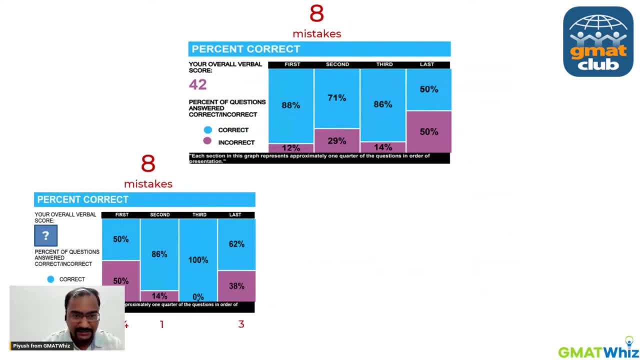 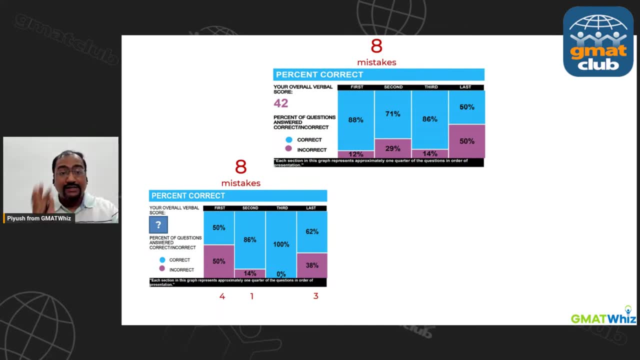 another scorecard. okay, this guy has also made eight mistakes. just take uh. change the orientation of the screen now the visibility will be better. so this guy has also made eight mistakes. the distribution of the mistakes is slightly different. like uh, for for the first student, shreyash, he made one mistake here, two mistake here, one mistake here and four. 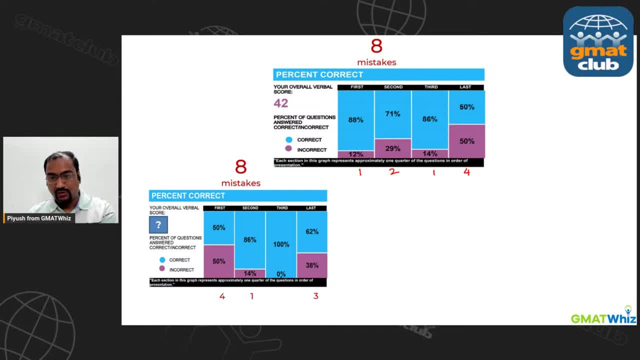 mistakes. here. the distribution is slightly different. for the second student, i wanted to look at the scorecard of this particular student and guess the verbal score of this particular student. he has made eight mistakes. shreyash also made eight mistakes. shreyash got a verbal 42, that's. 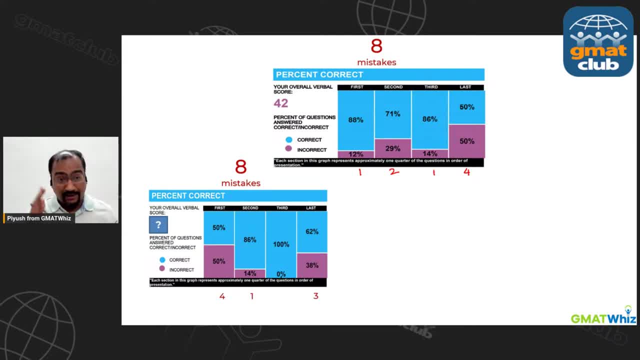 your benchmark, what could have been the verbal score of this student? i know i'm asking you to make a guess, but i want to hear all your thoughts. all of you talk, presenting your thoughts. uh, it's okay. if you're wrong, it's okay, but at least take a guess so that i can understand who knows the. 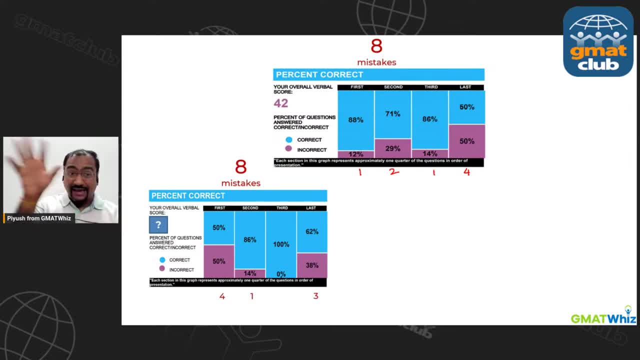 algorithm well. how many of you do know the algorithm well? because the reason why i'm sharing all this data in front of you is to help you understand the test. basically because if you don't understand the test and you're just practicing randomly, that's not going to help you improve your. 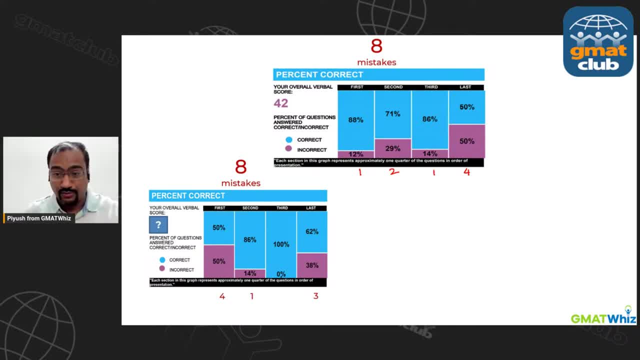 so, akila, i'm asking about akila, i'm asking about just the verbal score, not the total score, just the verbal score of the student. okay, ashok says 38. so ashok is saying the verbal score should be 38. akila says should be 35. okay, but why so same number of mistakes, right? okay, doodler is also. 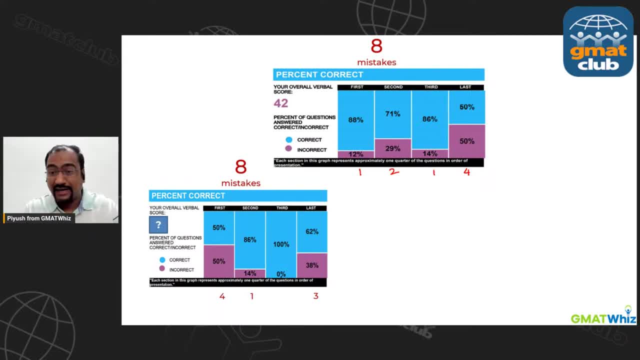 gunning for 35. so i have two people going for 35, one person going for 38. what about others? okay, isaac says should be 38. okay, isaac joins ashok. so i have, uh, two groups till now, ones who are going for 38 and the others who are going for 35. any other thoughts, guys? 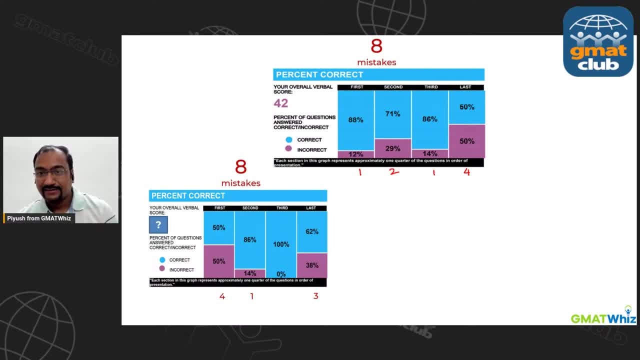 any other school of thought. okay, now i have uh mofusel saying it should be 32. all right, that's interesting. what about uh gargi nishita? what do you guys think? okay, i have zack and nelson joining in with 44. 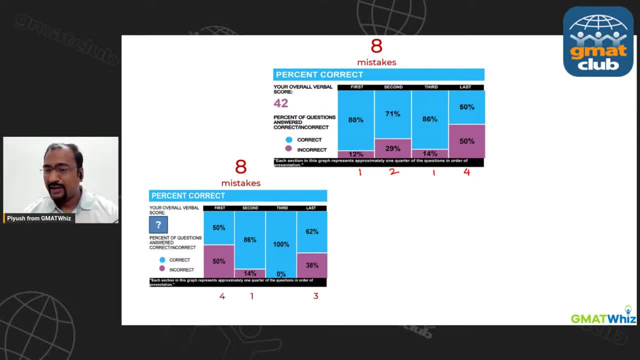 okay, you guys think it should be higher than 42. okay, any particular reason why you guys think, zack and nelson, that it should be 44 more than 42? any particular reason? okay, ashik and samistha has also joined in: uh 32 and 33.. ashok says relatively easier questions are wrong. very good, 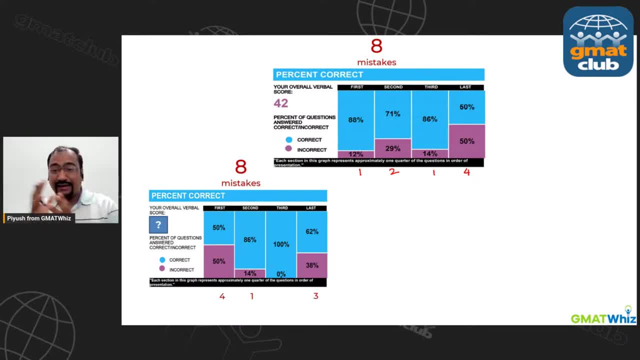 point ashok. so i see most of you uh in the thinking in the range of 35, 38 in that range, a few of you saying that 44, some of you saying 32, 33.. uh, let me uh show another esr. this i'll come to as well. 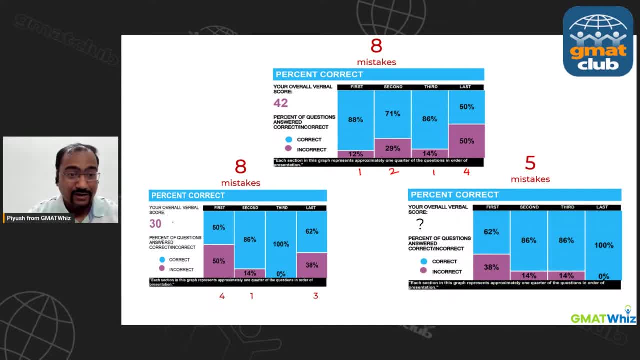 but let me reveal the score of the student. the student scored just a t on verbal. okay, try to make sense out of it. okay, 30 on verbal, 42 on verbal. exactly same number of mistakes. okay, jay kumar now says 26. so jack one has, like uh, provided a very low estimate as well. so, 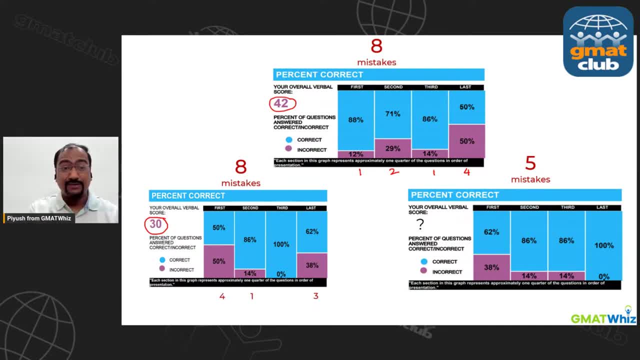 uh, 26. okay, possible, it is possible. i've seen people with nine mistakes getting a 21 on gmat in verbal. okay, i'll come to the analysis. don't worry, many of you are thinking how this, how that, but i have shown another esr and i want to make this even more interesting. 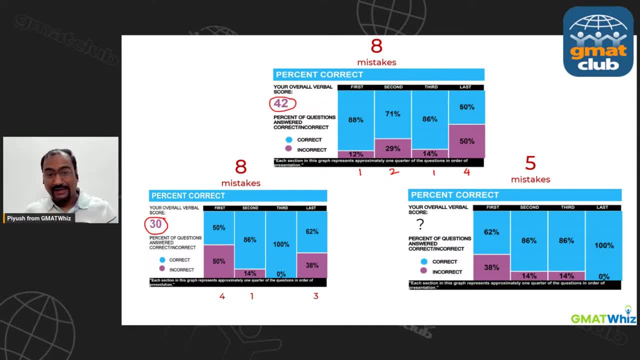 so i'll show you another esr on the screen. now, guys, five mistakes on the test? okay, five mistakes on the test. keep the benchmark. eight mistakes: the guy gets a verbal 42. now, what do you think? five mistakes, what should the score be? okay, mufasa says i am more correct. i said 32, yes. 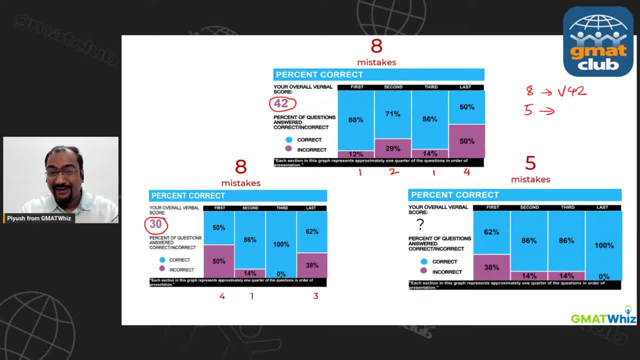 you are, i think, the closest to the uh correct score. what about other like? what about the second student? guys, let's make a guess on the second student. let's see how many of you understand this are genuinely okay. i'm not proctored this in uh adobe or anything. i don't know photoshop, i can't. 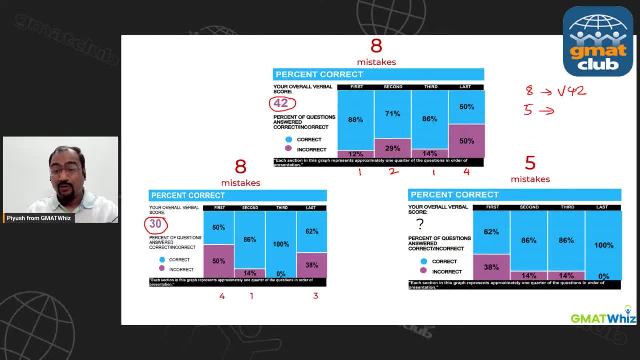 do that. i have not done that. these are actual scorecards of students who, who we know. okay, ashik says 38, but why less, ashik? why do you think it should be less? shouldn't it be more than 42? like the, the student has made eight mistakes with 42. like, uh, the student who made eight mistakes. 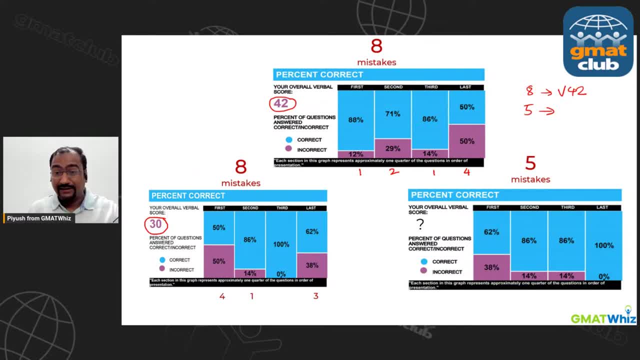 got a 42. this person has made five mistakes should be more than 42. right, that's how things should work: better accuracy, better score. akila says 30 to 35. okay. isaac says it should be close to 40.. yeah, makes sense, right, it should be close to 40. like, with eight mistakes, 42 you're getting, but i i see. 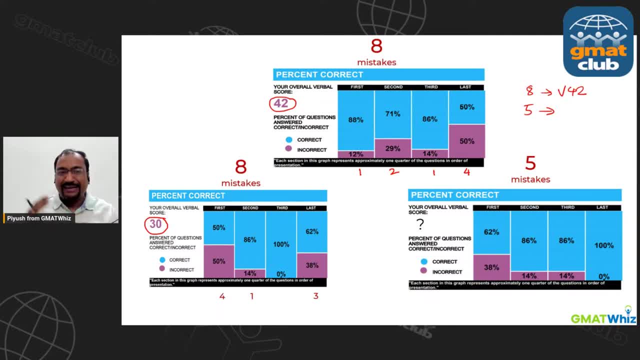 that many of you are seeing the other student as well, so i'm happy to see that now your estimations are getting more accurate. some of you are benchmarking with the 30 guy. also right, eight mistakes, 30, so probably with five mistakes, slightly more than 30. but how more, how much more? 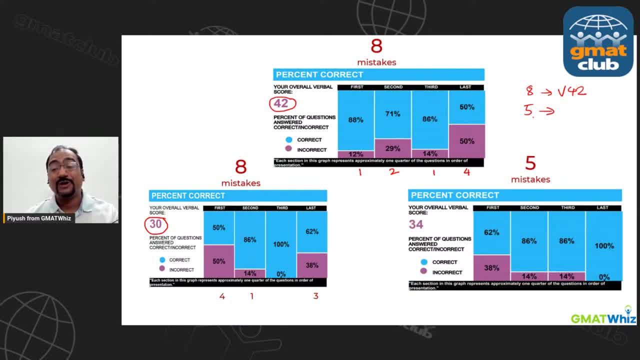 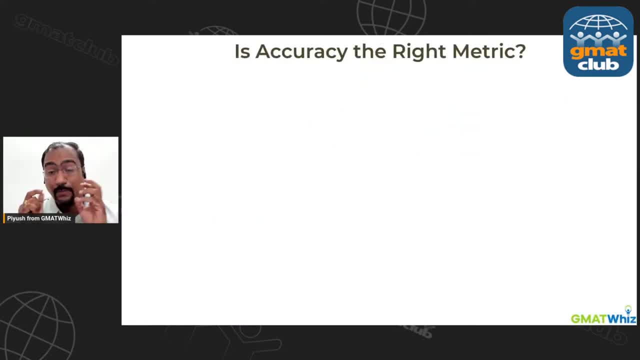 than 30.. uh, so again, this student just scored a 30.. this student just scored a 30.. this student just scored a 30.. now why i, why i'm presenting this to you? the reason i'm presenting this to you is to bring. 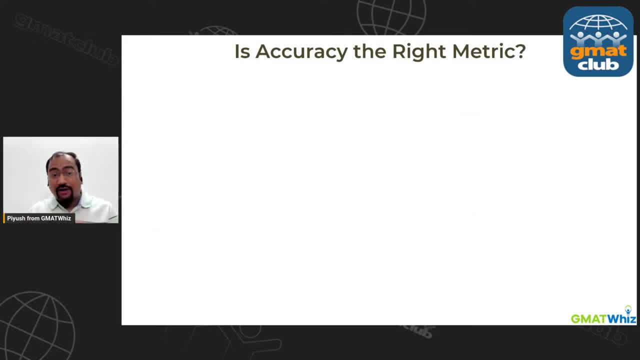 your attention to a very common misconception. a lot of people think that accuracy is the right metric to look at gmat. i have come across this question a lot of times from a lot of people who come to me and say if you should know what, when i'm solving official guide questions, i'm 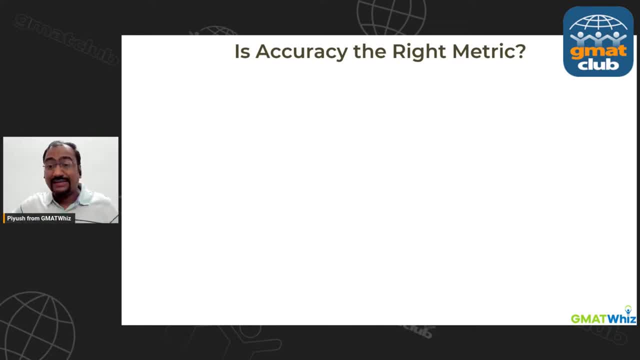 getting 80 plus percent accuracy. my accuracy is 85 percent, 90 percent, but when i take marks, my score is 100. how many of you have heard this statement? if you have heard these statements, do say a yes in the chat. if you have not heard this statement, say a no. but how many of you have felt this or heard? 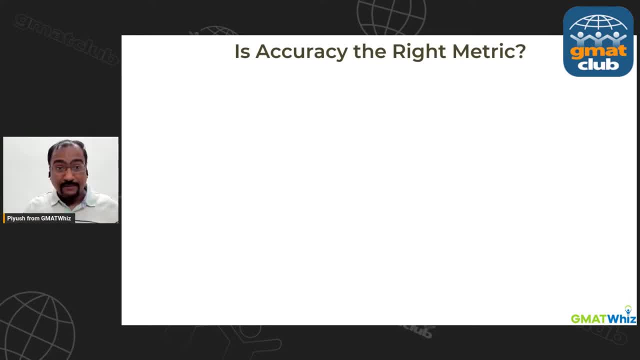 this statement from someone. this is a very, very common thing, because most people keep accuracy as the as the key metric, basically. so you are not understanding gmat completely. if you think accuracy is the correct metric, the data is in front of you. you can see with exactly similar. 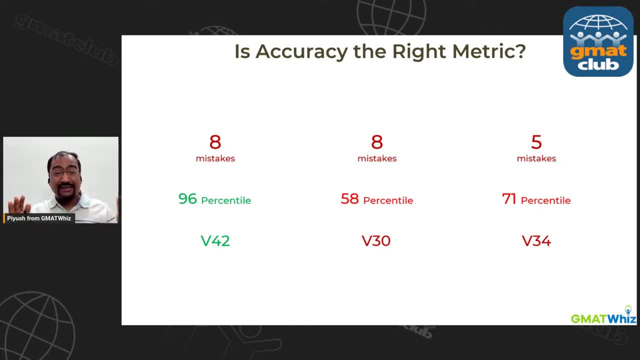 metrics and so on, but when you compare the data of people who have made the mistake and the people who haven't made the mistake- it's two people, eight mistakes- the score is significantly different and if you compare the percentiles, it's massively different. one person is: 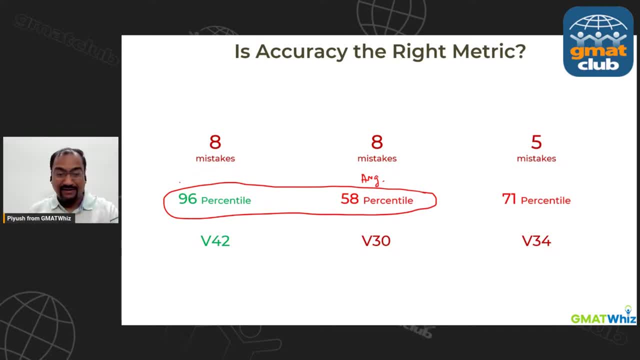 just performing average. this is just an average score. and the other guy is like exceptional, like this is above 95 percentile, this is above the bell curve, right like this, the amazing, amazing score. and then you look at a person who has made five mistakes. compare that guy with the verbal 42 guy. 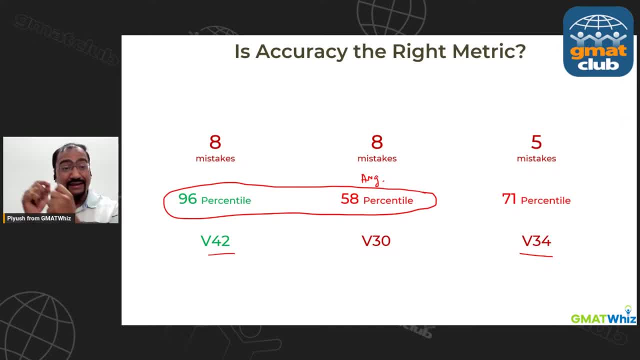 you'll obviously feel bad for him. right like five mistakes: verbal 34.. how does all of this make sense? All of this makes sense because in GMAT, something matters more than accuracy, and that is that what matters is basically which difficulty level of the questions you're getting right. 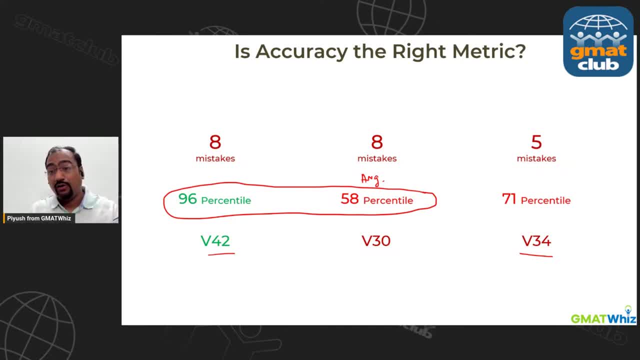 So Isha has a point. Isha says can't say, without knowing the difficulty level of the question, wrong question right. So I would say can't say like just say is the word for wrong to right. So your GMAT score is not dependent on your accuracy, like it's not dependent on your 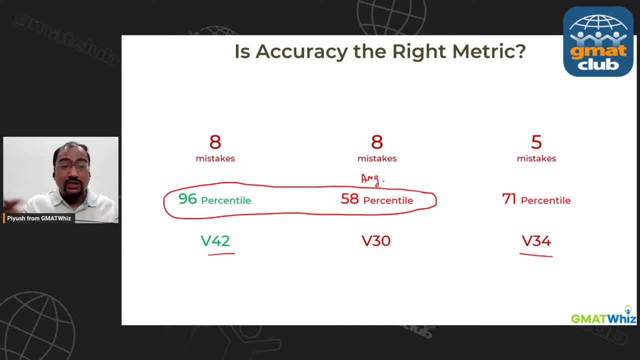 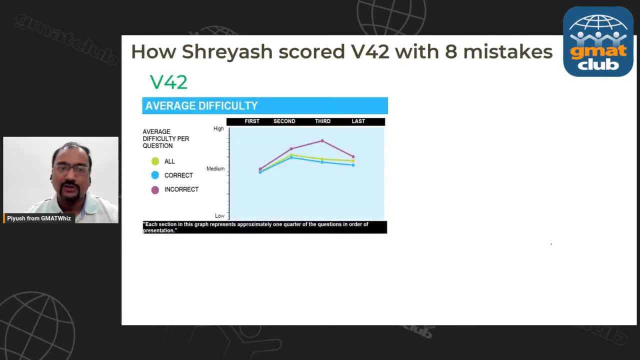 accuracy. It is actually depending dependent on the difficulty level of the questions that you're getting correct. Okay, So that's something which is important. So let's make more sense out of this data. So let's talk. let's let's talk about Shreyash's example, the verbal 42 guy. 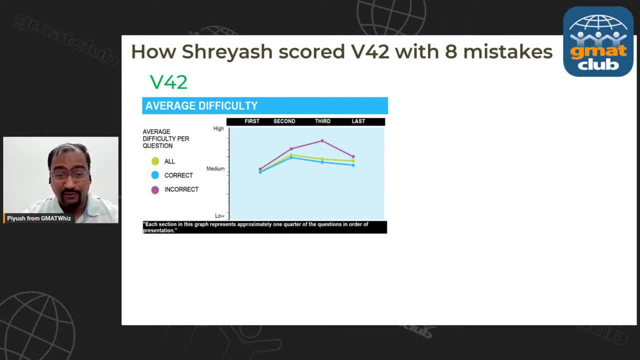 Okay, And again, I can't talk about his entire case. I know a lot of you want want to know from Shreyash how he scored a 760 on the GMAT. I can't talk about his entire case, but if you want, you can watch this interview. 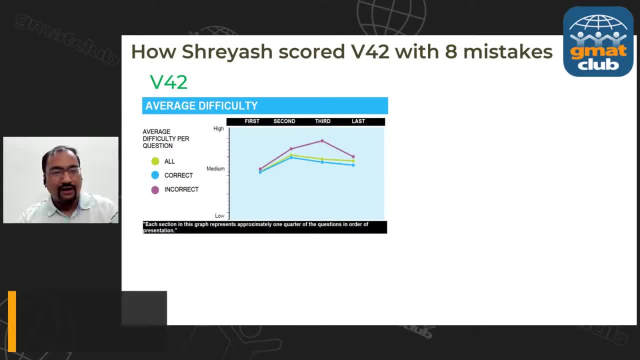 I'm just sharing the link. You can bookmark this. watch this interview later for your reference as well, to know more about his case. But I'll just quickly share the analysis of this particular person and I'll try to help you understand How the algorithm is actually functioning here. 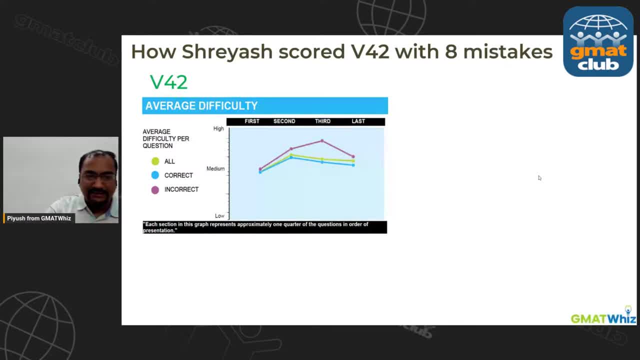 So what happened in this case is that when this guy started, if you look at this chart, it shows us the average difficulty level of the questions- correct questions in blue and the incorrect questions in red- and it is showing us the average difficulty in the four. 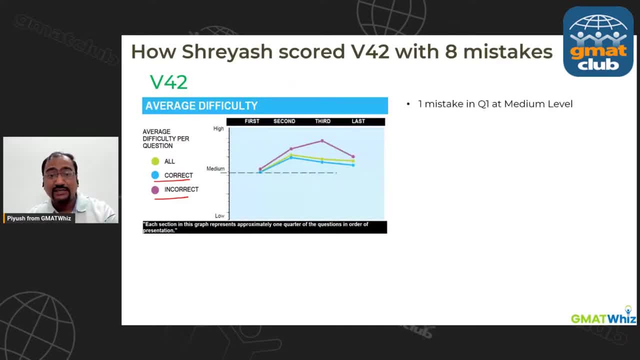 quarters. So in quarter one this guy, Shreyash, made only one mistake And, by the way, Shreyash is right now a Harvard student. He's going to graduate from Harvard next year. So this guy made just one mistake in the first quarter. 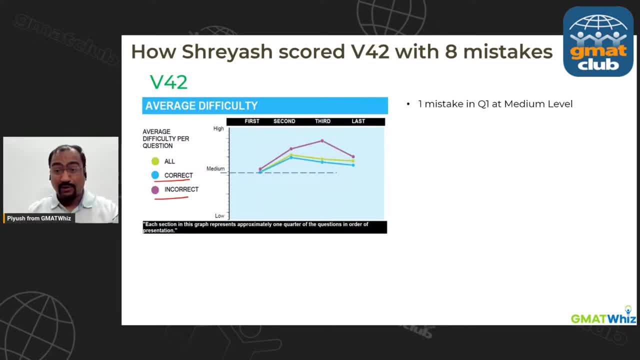 Okay, But at the medium difficulty level, right? I don't think Shreyash is leading at the same level of difficulty here, So it doesn't matter, He can carry 760 problems, But if you look back at there should be more, like you know, 25 Yeah. 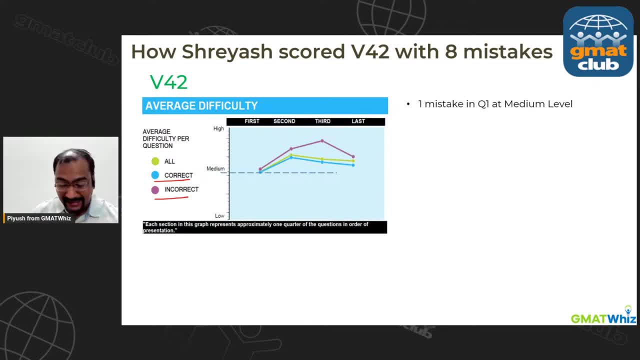 Can you see the math? Okay, Then he shows this. what is this? Let's see. Okay, That's all, Thank you. Thank you, Bye, Bye, Bye, Bye, Bye, Bye, Bye. medium level questions correct. so what happened and the most important thing you need to understand? 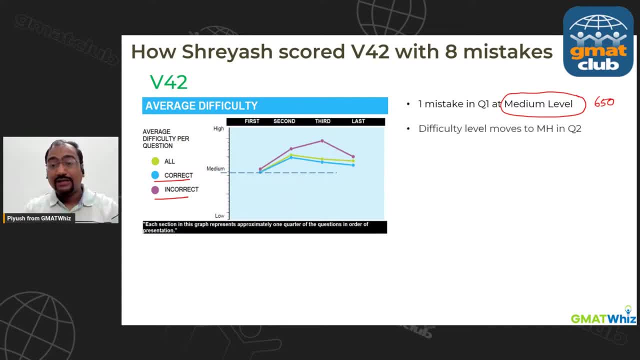 was the consistency in medium level questions. so what happened was the difficulty level of questions moved to medium hard in quarter two. let's do let medium hard. you can think of it as 700 level. so the algorithm now felt that we can try testing him on medium hard questions. 700 level questions. 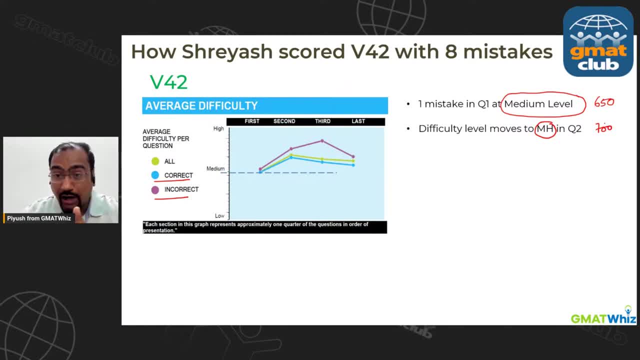 because you can get 650 level questions correct. now we got five medium hard 700 level questions correct in quarter two. you can see this uh line like: move to 700 level questions in quarter two and you see this line is: this dot is very similar to similar level to this line. so five medium hard. 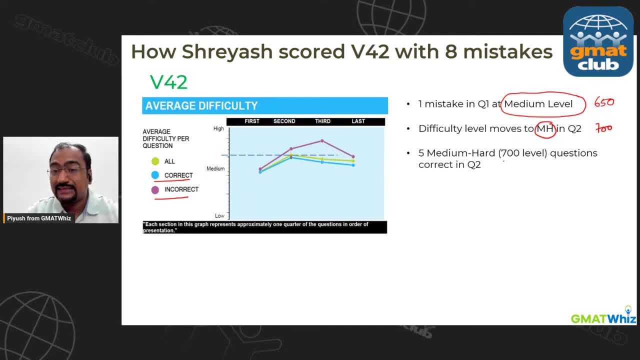 questions he got correct, so the algorithm understood that he is. he can easily get 700 level questions correct as well. now gmat started testing him on 750 level questions, basically like hard level questions, let's put it that way. so what i'm trying to say is that he was able to show gmat 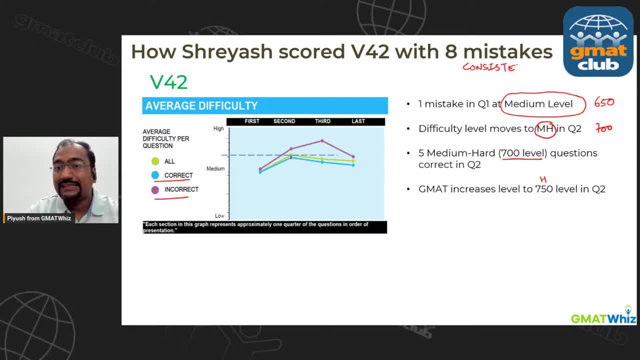 that he is concerned the condemning good. he is consistent with safety and 700 level questions more. he can get almost all of them correct. okay, that's when the algorithm moves to 750 levels. he was not able to get those question side. he made two mistakes over there. the mistakes happened at: 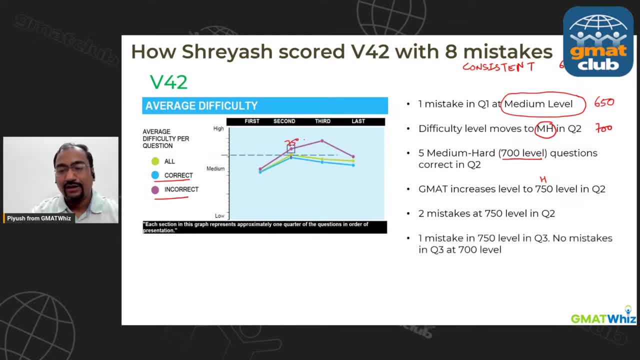 750 level questions only. and that's when the algorithm again like kept him at 700 level, 50 level in the third quarter also. he made one more mistake in 750 level. algorithm felt that okay, probably he can't get 750 levels questions right. so he was brought down back to 700 level again, but he did not make any mistake in. 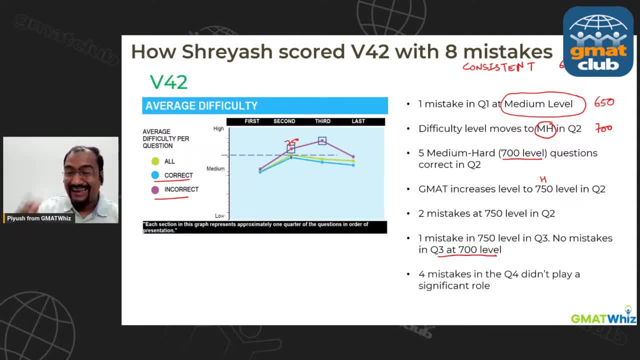 7700 level questions at all and because of that, the last quarter, the four mistakes that he made in the last quarter, did not play a significant role. why did it not make a significant role? because a lot of people think that your score is determined based on the level, that at which you 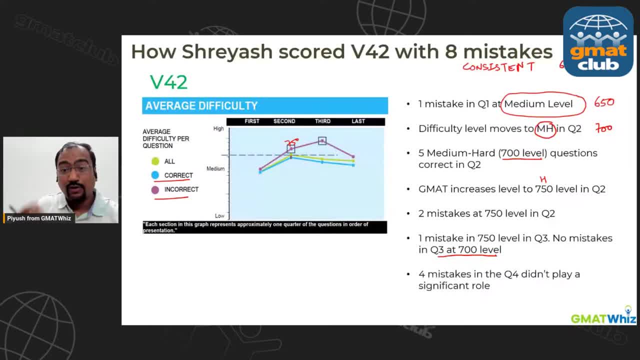 end the test? not really. it's not just that, it's also about the difficulty level of the questions that you are getting right. so what happened with shayash was that he was able to consistently get 650 level and 700 level questions correct. the consistency is the most important thing that. 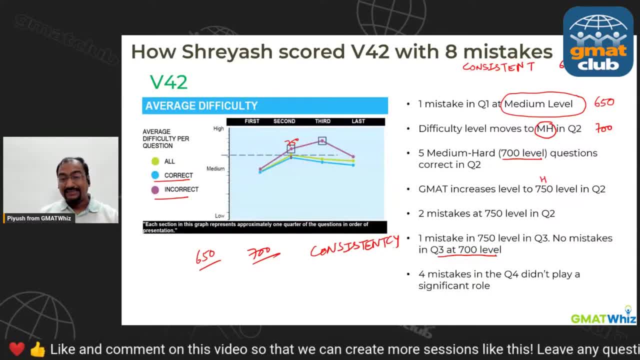 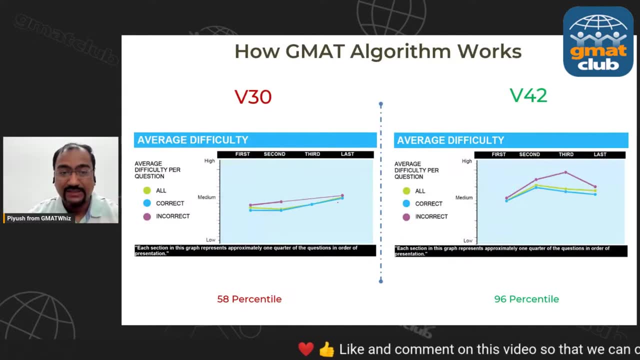 you have to focus on right. since he has consistent- consistent there- the algorithm did not penalize him a lot. the algorithm made sure that he gets the right score, so he scored a verbal 42 because of that. now, if you compare that with the verbal 30 scorecard, the person who made eight mistakes 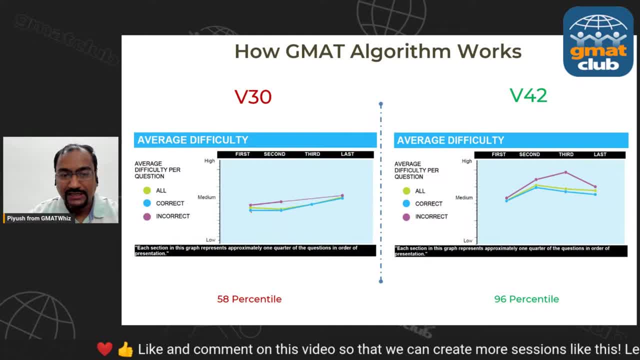 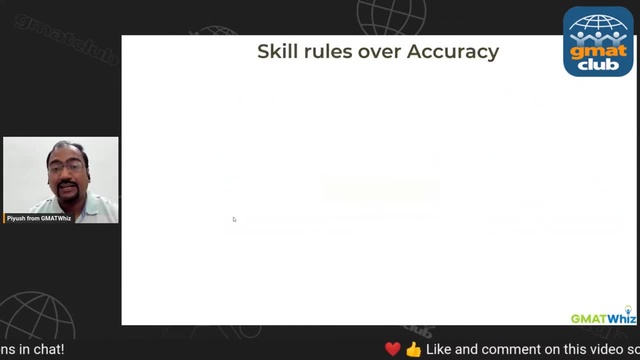 if you compare them side by side, you will see that the correct questions were always in this range of medium itself, which was like 650 level only. in fact, in many cases he had made like four mistakes in the 650 level also in the beginning, so that's why the score was low. that's what you need to understand over here. so what matters on, 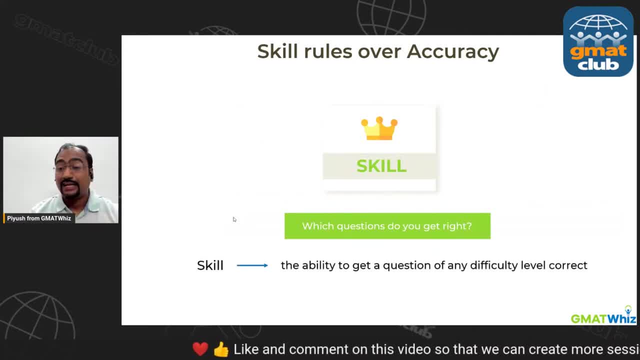 gmat is not accuracy. what matters on gmat is your skill, the ability to get a question of any difficulty level correct. so if you're just practicing randomly and you're being very happy with your accuracy, without considering what is your accuracy in the more difficult and without considering the consistency factor- the consistency factor is also very critical- if 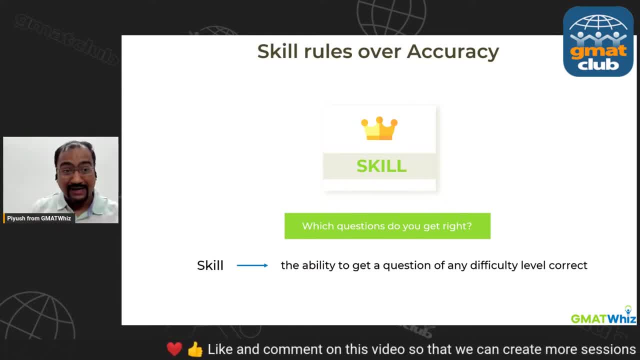 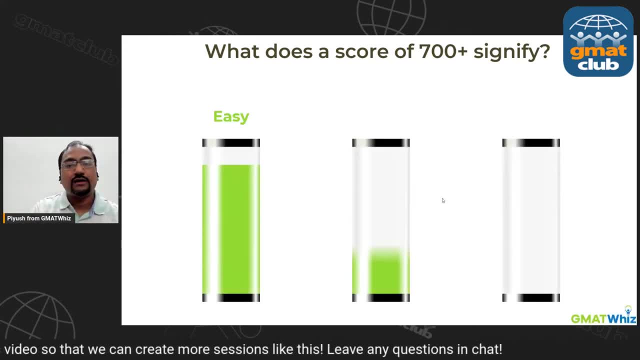 you're not taking into account those two factors, you're not preparing for gmat in the best possibility. okay, so what does the score of 700 plus really signify? to get to a 700 plus, you cannot go wrong with easy and medium questions because again, remember shares his example. he 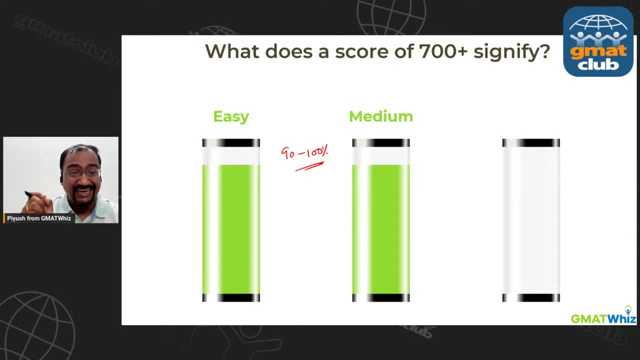 hardly committed any mistake in that level. you have to start the test right. but starting the test right is just a part of it. you need to also get the hard questions correct. so to get to hard level you have to pass through the medium level. but once you get to the hard, 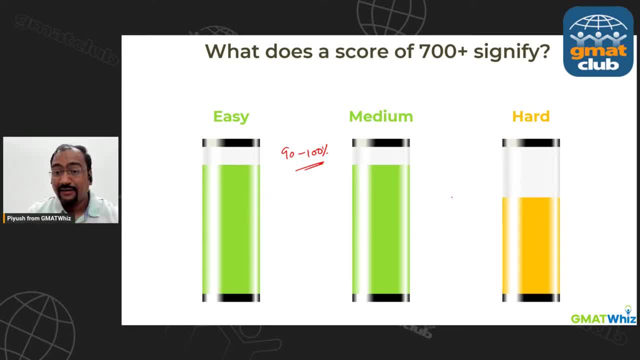 level, you have to get them right. so if you are looking at a 700 level, 50 accuracy will be sufficient for a 700 level. okay, but if you are looking at a 750 level, let's say you might have to look at somewhere around 75 to 80 accuracy. in the hard questions, like when i say hard, i 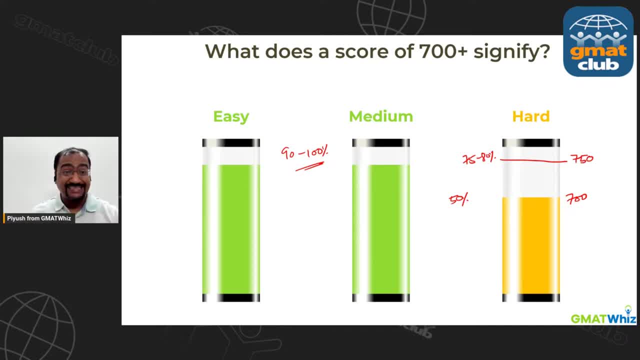 mean 700 level questions basically. uh, if you are looking at 760, 770, you might need to also get some level questions correct also. okay, so that's, in short, what matters on gmat. so if you have gained certain understanding from this, do share your thoughts in in the chat here. what is the learning? 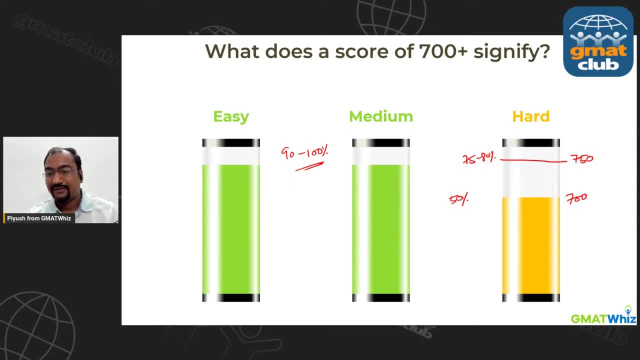 that you have gotten uh from it now. okay, so do let me know if you have any thoughts here for the same and uh, like, like in thoughts as in you have. what is this understanding that you have generated from this? i would love to hear them that from you and, if you are liking, 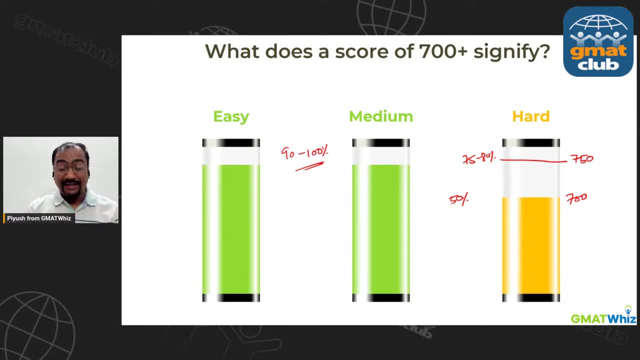 the session till now. do give it a like and subscribe to the channel. uh, i told you i have a target of 450 likes. if i meet that, i will see me again. uh, so do give it a like if you have actually found something interesting and found something uh very insightful through the session. so 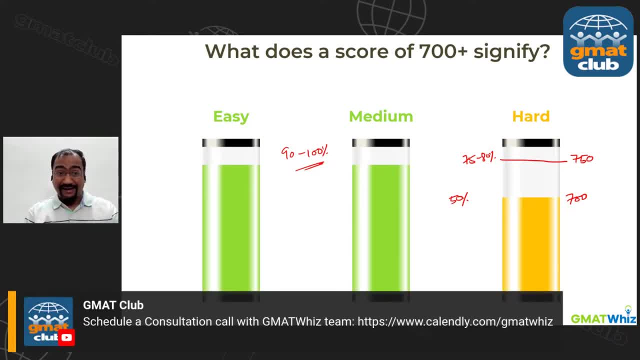 they give it a like, and i'm also sharing a link to schedule a call on my calendar in case anyone of you wants to connect with me, discuss your progress, understand how the gmat, this team, can take your score to the next level. we have been, uh, the one of the most important things that we have. 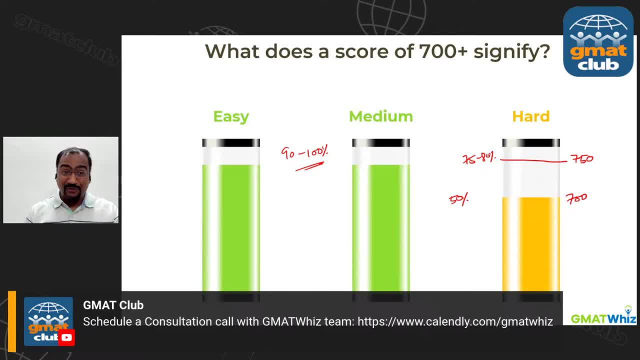 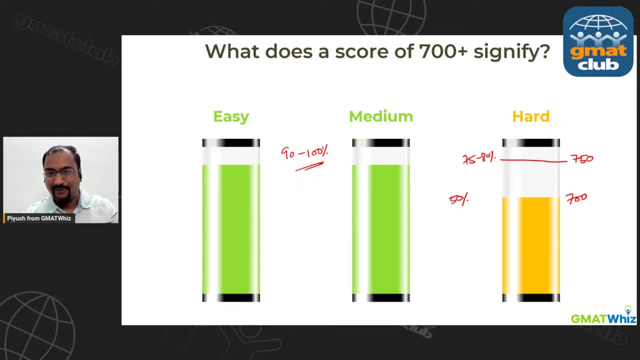 like we have generated the highest score improvement in the industrial day. so if you want to take our help for gmat for improvement, do feel free to reach out to me as well, but i don't see any comments from you guys till now. what is your summary summary of this that i have discussed? okay? 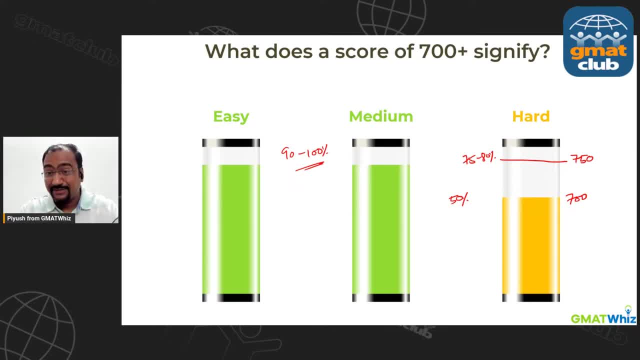 nelson says that. uh, it's very insightful. i have learned something new. but what is that new that you have learned? i would like to hear your thoughts. how would i? how have you understood this basically? so, just to summarize, the main idea which i'm trying to propagate here is that 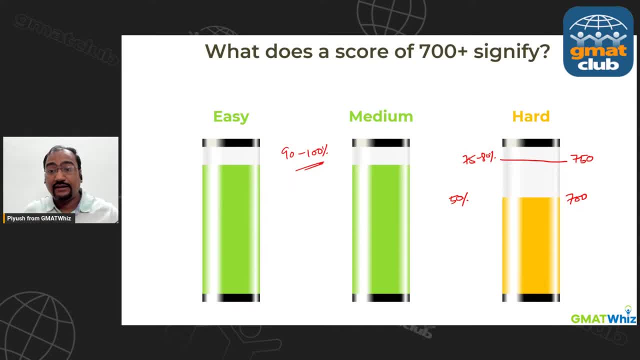 gmat is not just any ordinary test where you can just think about the uh accuracy overall. you have to think about the difficulty level of questions also. you have to be consistent with them as well. if one day your score is very good, another day your score is pretty bad, or one day you're doing 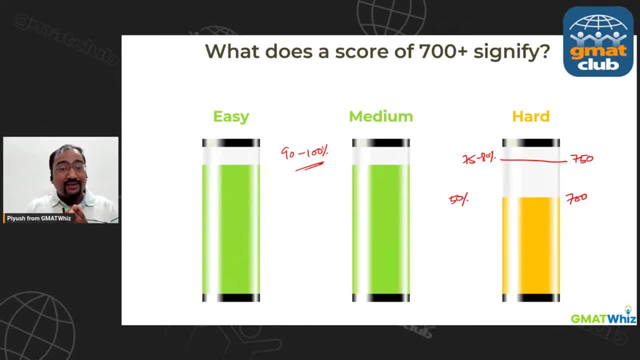 well on hard questions. another day your score on hard questions is not good, you'll not be able to. you might not be able to get a good score on gmat because in gmat consistency matter, it's an adaptive test. if you don't get the questions correct, it will face problem. now i'm 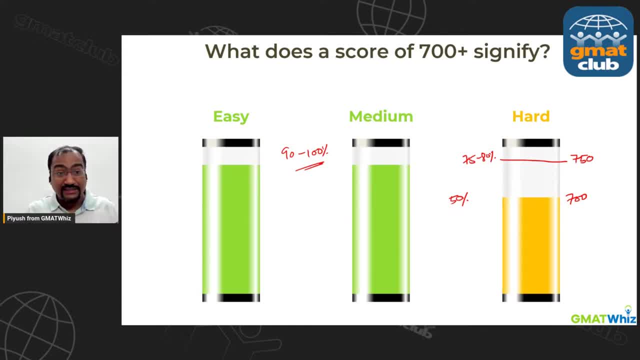 i've seen a question from ashok and community medicine also about focus edition. in the focus edition also, same thing is going to happen because it's an adaptive test. question level: adaptive test: same algorithm is going to work. obviously the scoring and everything is different. but at the 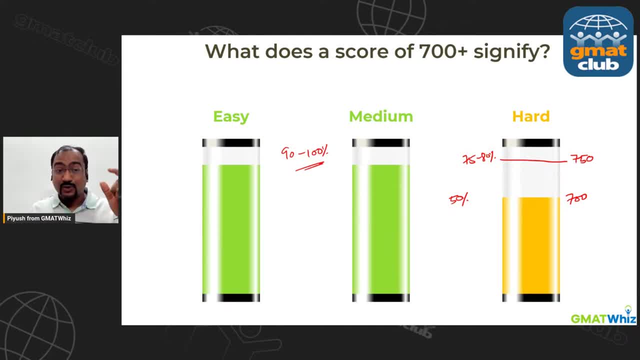 end, the percentage course will basically be decided in the same way. so whatever i'm telling you today, i'm using uh gmat classic scores as a guidelines because obviously, gmat focus scores are not out yet, the test has not started. but whatever i'm telling you today will work equally. 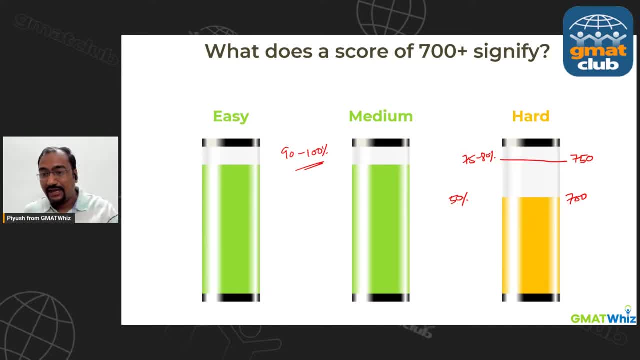 well for competition as well. okay, so that's it for today, Thank you, Okay. Isaac says I've learned that we have to make sure we spread out the errors we make, and this is based on difficulty level two. That's a very valid point: spread out the errors. 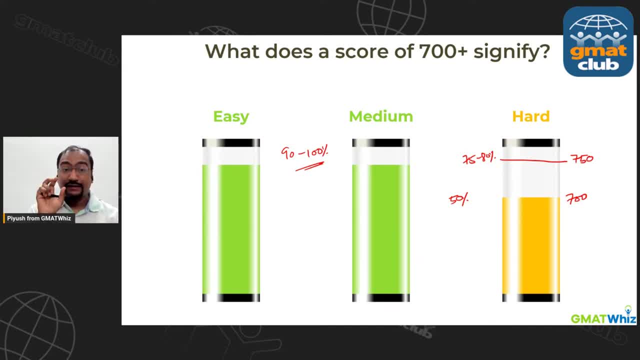 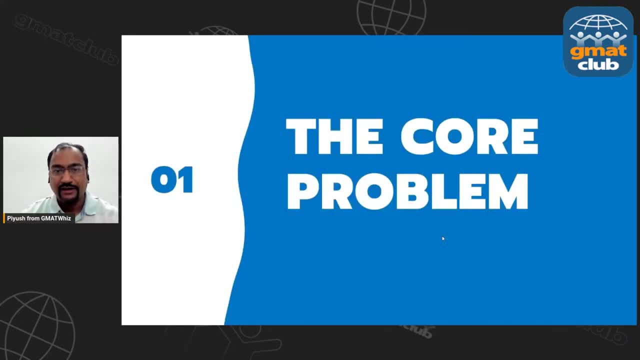 More important is consistency. Now what the main thing you have to focus on is getting consistent accuracy. and back to your hard questions. Now that brings me to the next point, the core problem. The core problem generally is that when it comes to hard questions, 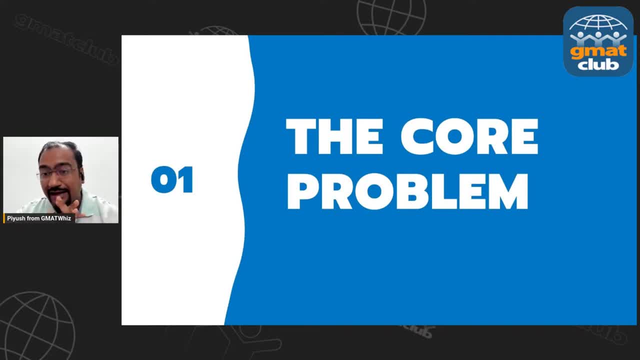 people think of hard questions in a very different way. Okay, and again I would love to ask you: how do you tackle hard questions? What do you think is the main solution to tackle hard questions? But again, we have been into the session for half an hour. 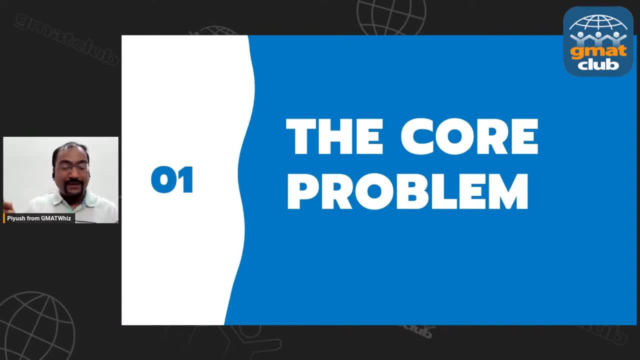 so I want to just move forward with it a little. So I'm gonna increase the pace a bit, but I'm gonna ask you whether you agree with me or not on the core problem. So do say yes or no when I actually present the thought over here. 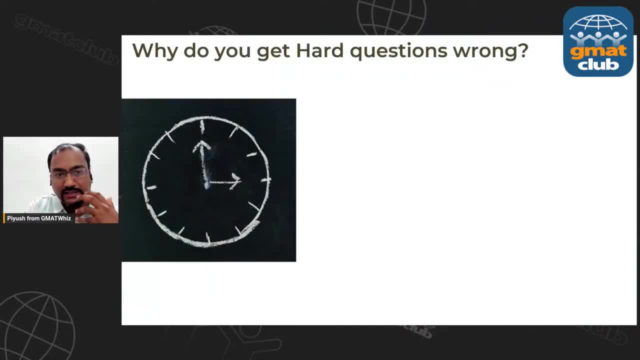 So, when it comes to hard questions, when it comes to hard questions, this is the understanding of people. When they think, why do they get a hard question wrong, they think in like most of the people think in one simple way. They think that they can possibly get a hard question. 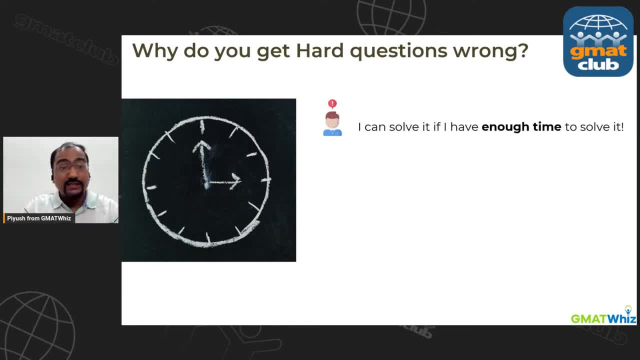 correct if they have enough time to solve it. If you also think the same way, do say yes in the chat. I wanted to ask you this question, but I'm not to save just some time. But if you feel the same way, 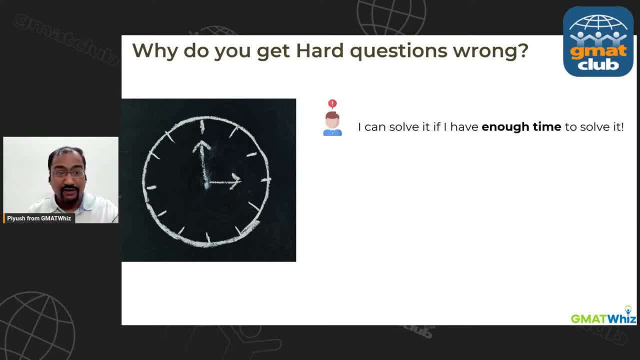 that you can get the hard questions right if you had enough time to solve it. It's just because of lack of time you're not able to get the hard questions right. Do let me know their thoughts in that. What does that mean for chapter-wise accuracy? 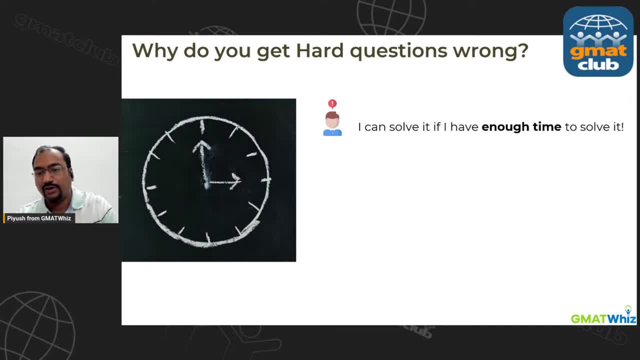 For example, I can do easy, medium, hard for some chapters, but only easy medium for some. what do I do? So, Isha, again, if you are only able to do easy, medium for some questions, not hard, then first you have to become consistent. 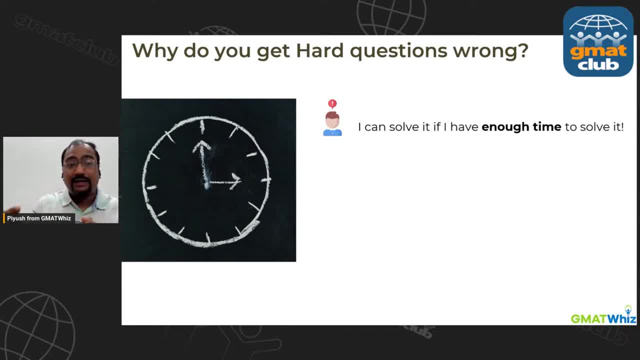 with easy medium properly, Then take up hard questions one step at a time. but you have to get hard level questions correct. Like one or two hard level questions wrong doesn't create a lot of impact. So if there are one or two chapters where you're getting those questions wrong, 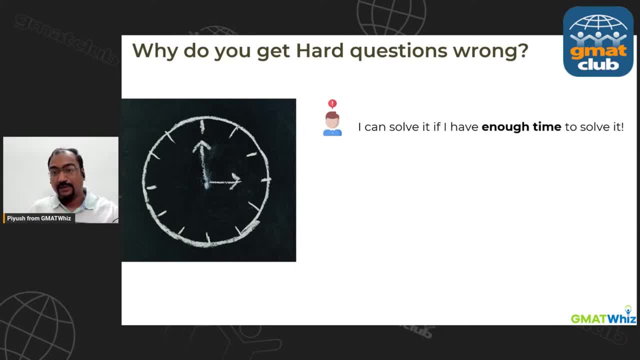 it's still okay, but that can't be too many chapters, Then it's a problem. So Madison says no, Amart says yes, community says yes, Isaac says no, Mosfer says yes, Insha says yes. So I do see a few no's as well. 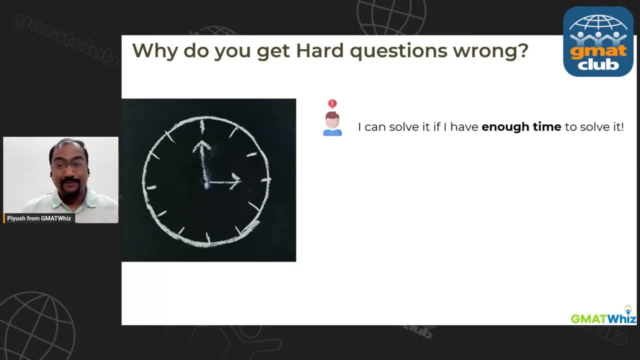 That's really great. Thank you so much for sharing your thoughts. I do see a good number of yeses also- that many people think alike. Many people think in the same fashion: that if I have more time I can get the hard questions wrong. 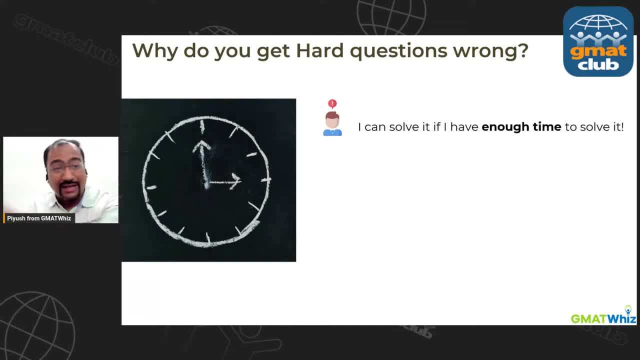 Now, when you think that, when you start thinking that if you had more time you can get the hard questions correct, what is your next thought process? The next thought process is: how do I learn to solve questions quickly? Yeah, that's our natural approach, right? 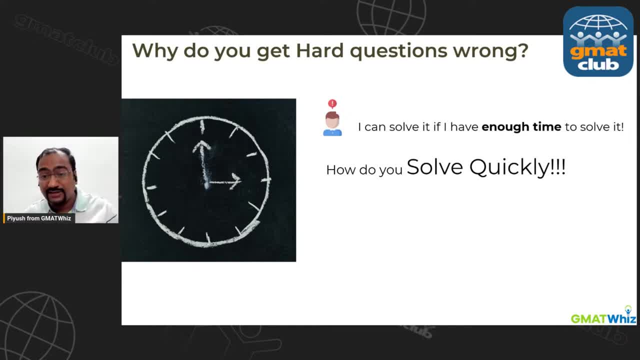 We don't have more time. Ashok says it takes me four minutes to solve some CR questions. but I get them right 90% of the time. But you know you don't have four minutes on the GMAT, So your next thought process is: 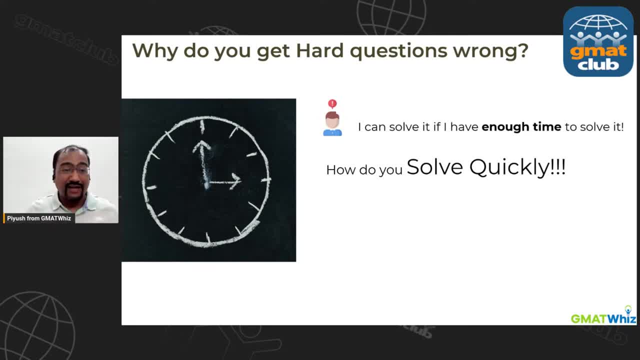 the moment you start thinking about timing, the next thought process is: how do I save time? How do I solve quickly? Now, the moment you think about how to solve quickly, the next thought process which comes to you is: I have to somehow cut corners, correct. 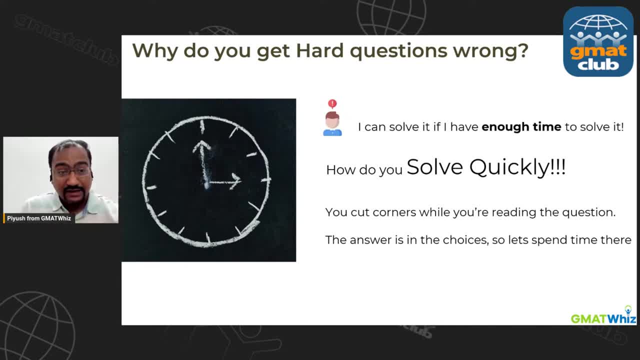 I have to somehow cut corners. and where do we cut corners? We cut corners while we are reading the options, because many people think the answer lies in the choices. right, And this is more true of verbal, I understand, but it is also true for quant. 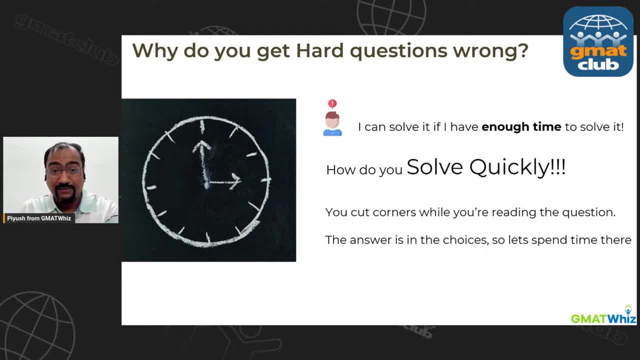 especially in data sufficiency. People don't spend enough time on the question. in many cases, they read questions faster In verbal. this is more true that answer lies in the choices. So let's spend time on the choices. So let's cut down time. 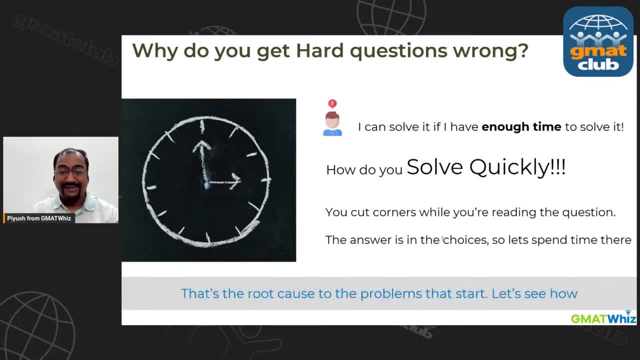 on the questions, then, And that's where the problem starts, That's the root cause to the problems that actually lead you to the score plateau, And I want to show you how you have to understand how. Let's see, okay Now, whenever you read a question quickly. 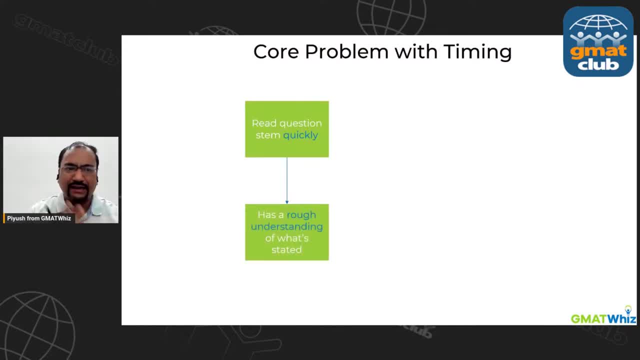 whenever you read a question quickly, you're able to understand it at a rough level. You have a rough understanding of the test- a question of what's stated. Now, based on that rough understanding, you're able to eliminate two to three choices confidently. 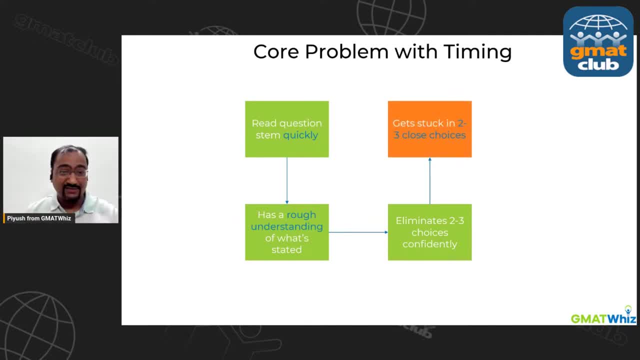 But the problem happens when you get stuck in the last two, three choices, Just the close ones. with a rough understanding, you can't answer those two, three choices. So what happens is whenever you get stuck in the last two, three choices. 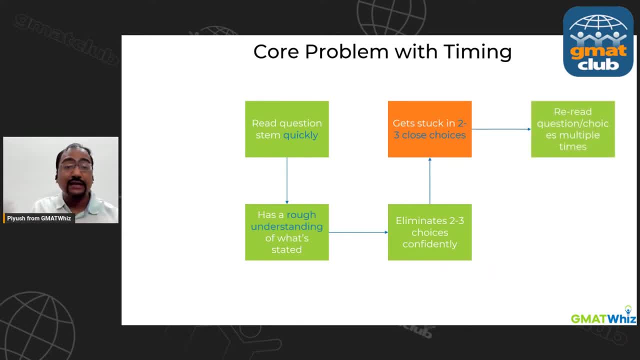 what do you guys do? Everyone, almost everyone, re-reads the question, all the choices, multiple times. Okay, And what happens after you read the options or the questions multiple times, even if you don't even after that, if you don't know the answer? 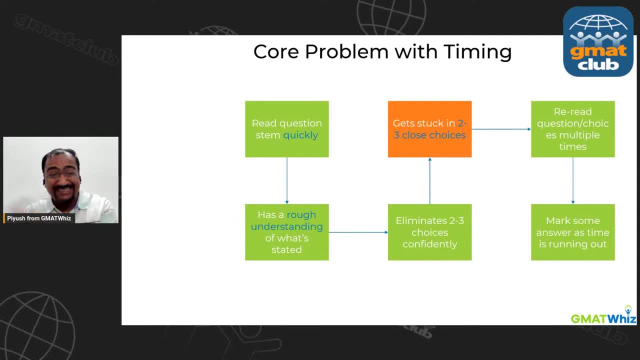 it'll mark something, especially if you don't know the answer. But when you read the options or the choices multiple times, even after that, if you don't know the answer, you will mark something as well. time is running out. that's the process which most people follow. so what started was the thought. 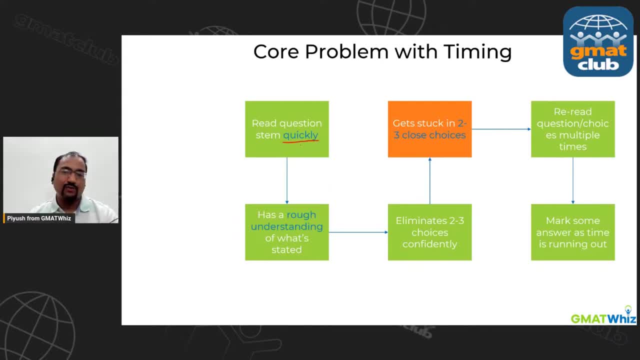 process of solving questions quickly that lead to reading questions quickly. that could have saved you time, because you did that in 20- 30 seconds and you are able to eliminate two or three choices in 20- 30 seconds. so at the end of one minute you feel that you have. you have come down to last two. 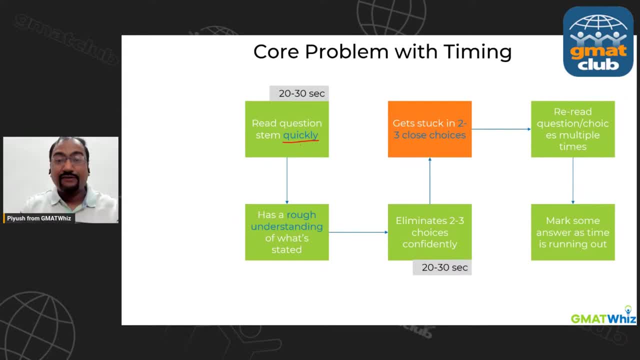 choices. that's when the problem starts. then have you, we're down to last two choices and you start reading things again. you are ending up spending actually a lot of time on this part, and then that's when you start thinking that my problem is not with timing, my problem is also 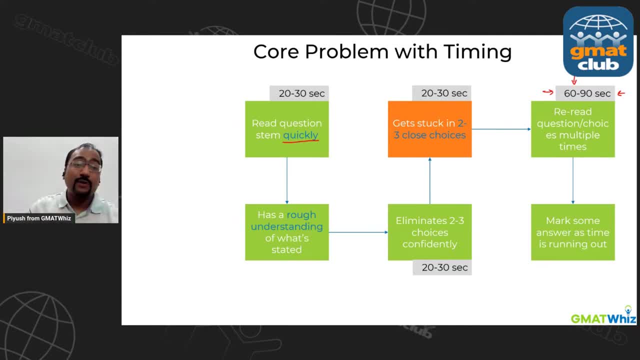 getting down to the last two choices. but what is the main problem in the entire picture? if you focus on the entire picture and you will understand that why you took extra time is because you read the questions time too quickly. that's the main problem, and this happens either. 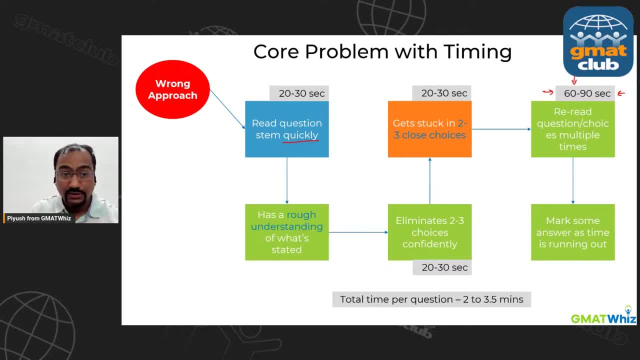 if you do because of the wrong approach, if you don't know how to approach the question side, if you don't know how to solve questions methodically, it can happen because of that. in my case this was the main reason i i remember in verbal no one taught me the right approach like my approach in verbal. 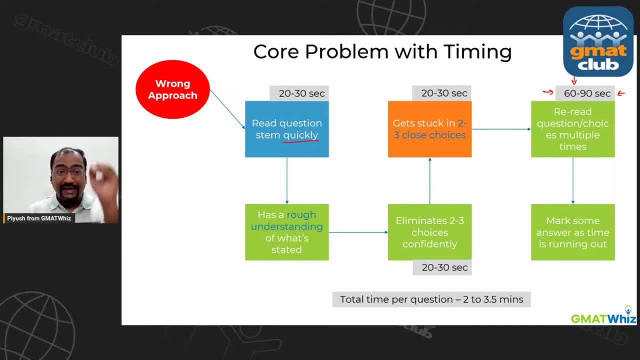 was just to read and eliminate choices. that's all i knew in sc. i knew: look to look at the options, identify the differences in the choices used by grammar understanding and solve it. and in rccr it was just reading, answering, reading, eliminating, reading, eliminating. there was more. 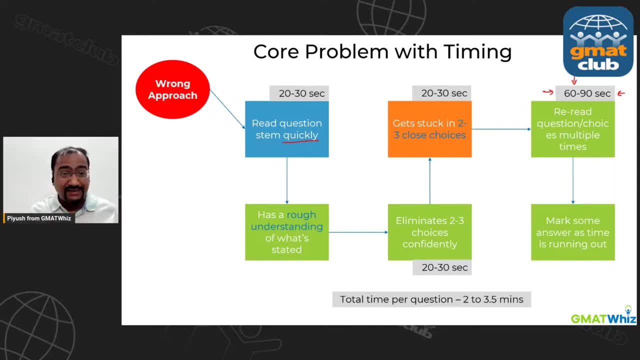 than madness. there was no approach. in fact, i didn't even know that there exists an approach. i didn't even know that i just thought of. i just knew you have to read. you have to read more. if you're not able to understand, read more and that will help. but how to read is something no one. 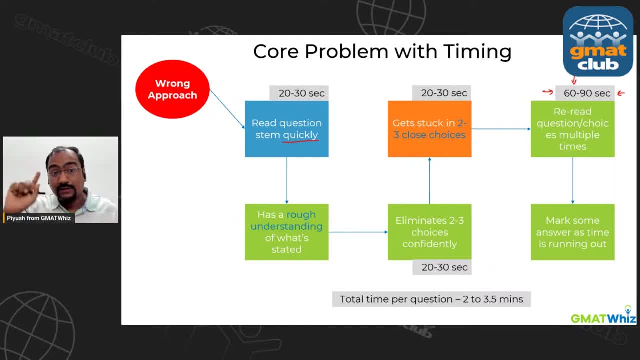 taught me. so my approach was wrong and that's why i was stuck at a verbal 13 even after six months. and after that, when i changed my approach, within about two to three months of effective preparation, i was able to improve my verbal score from a 13 to a 41. imagine that, okay. 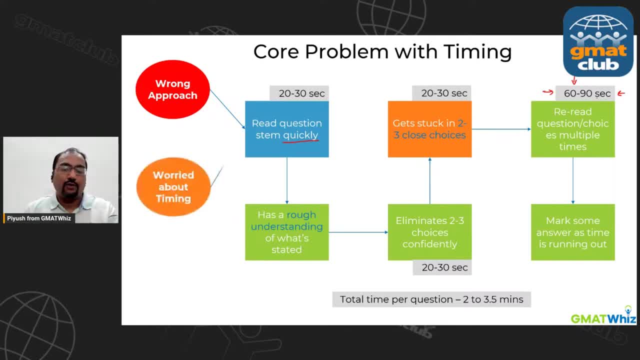 so wrong approach is one reason. second reason is when you're too worried about timing, you think, okay, i have to get the hard question side, i need to save time, and that's when you over compromise on basically the question stem. so both these are problems. so what? what is the solution? i'll talk. 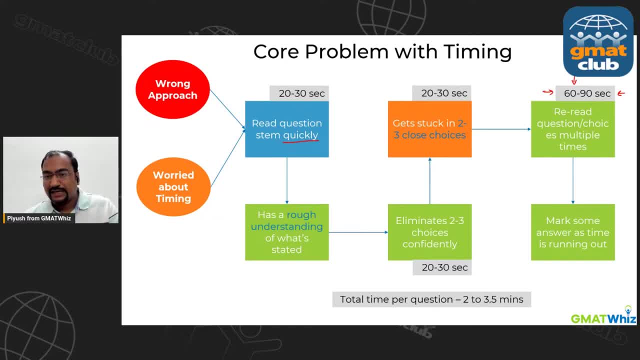 about that as well. but let me take up this question. she says: when i started doing verbal in the initial stage i used to take 30 minutes. then it came down to 15 minutes, then to six minutes and now three minutes. okay, i'm not sure if you're talking about one question per time, per question. 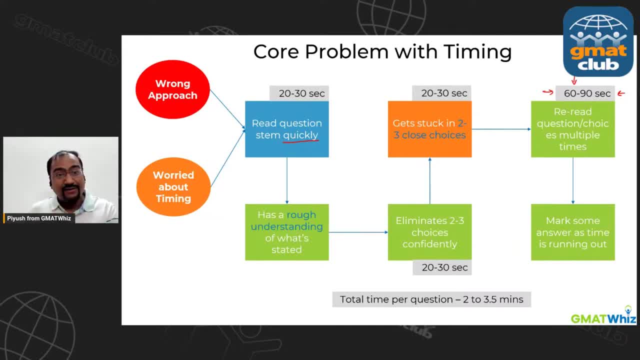 so it's good that your time is coming down, but again, you should not have even taken 30 minutes to start with. i'm not sure why that happened, uh, but do let me know your thoughts, or you can discuss that personally with me, uh, on a call, if you want to. i'm more than happy to discuss. i'll share the. 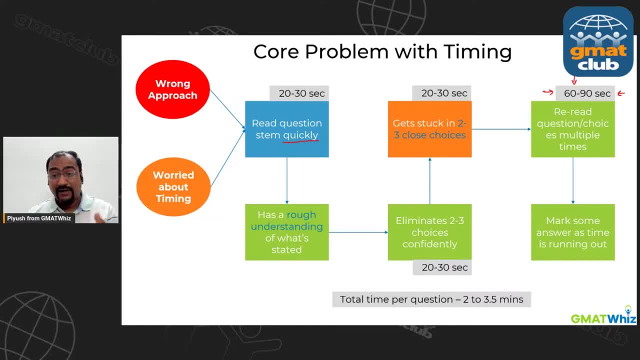 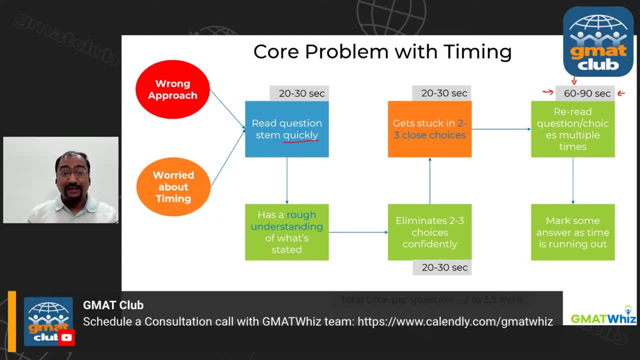 link to schedule a call on my calendar again, nishita, but 30 minutes per question time is too high, uh. so if that is the, that is the thing, and you'll have to understand why that happened. but if it has come down to three minutes, still good, okay. so this is the main uh problem. 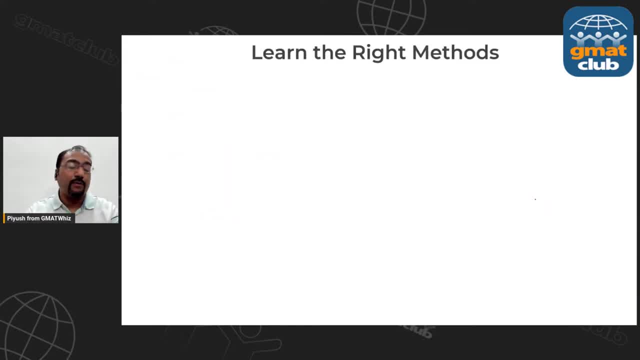 that people fall face. they don't have a proper approach. so, when it comes to solving questions, you have to ensure that you invest your time in learning the right methods. that's the key to score a 750 on the gmat. that's the most important thing, guys. there is no shortcut to this. let me tell you. 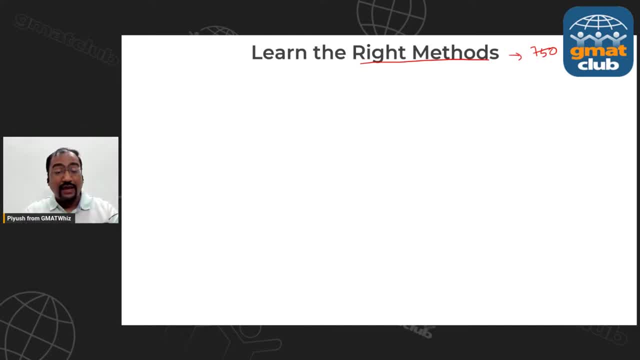 there is no shortcut whatever to this. if you're thinking, okay, 750 level questions are. if you want to get to that level, you have to get the hard questions correct. i've shown you enhanced scorecards making just five mistakes, not able to crack 750. i've shown you people making eight mistakes. 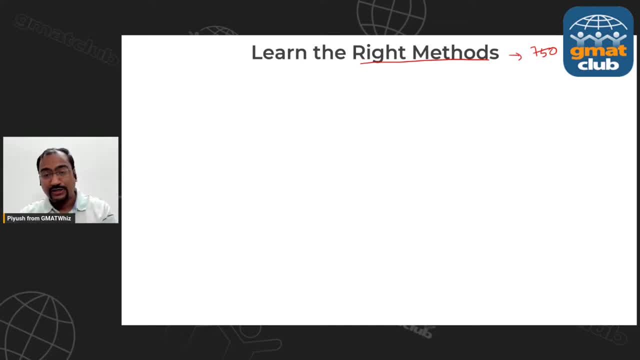 able to get a 760 because they got the hard questions right. and the thing with hard questions is that shortcuts or, uh, let's say, faster methods that you see here in the industry- skimming and all- there's a very, uh big name in the industry which is actually running into a lot of trouble: these. 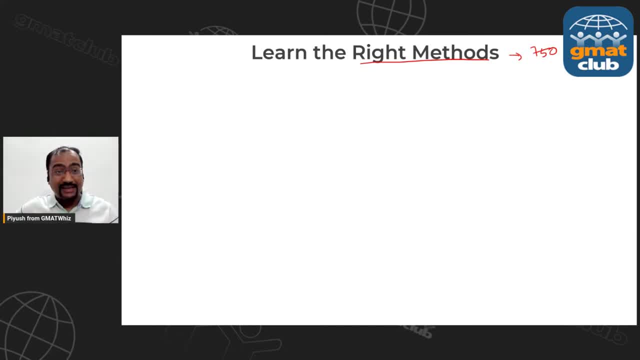 days who actually educate that you can actually read the first line of rc passes and the last line of rc passes and i pretty much answer everything. skimming works in rc doesn't work, so you have to invest your time in learning the right method. okay, there's no shortcut. and what are 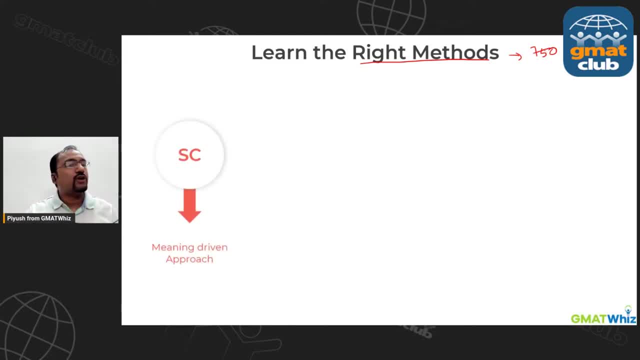 the right methods that i'm talking about. in sentence collection, you have to focus on the meaning based approach in critical reasoning. you have to learn pre-thinking and a lot of people don't even understand what this pre-thinking actually is. most people actually think pre-thinking is about rethinking the answer. it's not about rethinking the answer. it's about. 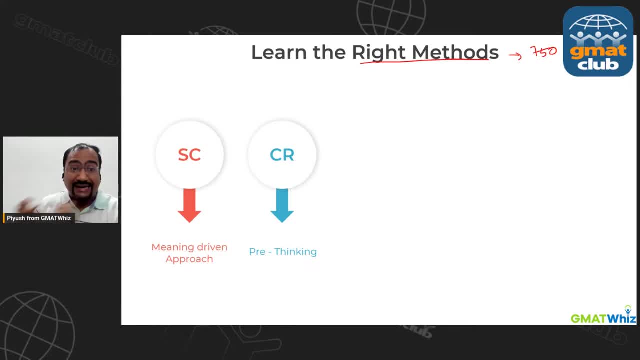 pre-thinking the argument structure before you go to the choices, understanding the line of reasoning, understanding the conclusion, understanding what is the scope of the argument. and again, we are planning to do a session on 25th on critical reasoning which will be taken up by sunita singhvi, who's our lead verbal expert at gmat race, who's an amazing teacher, has helped. 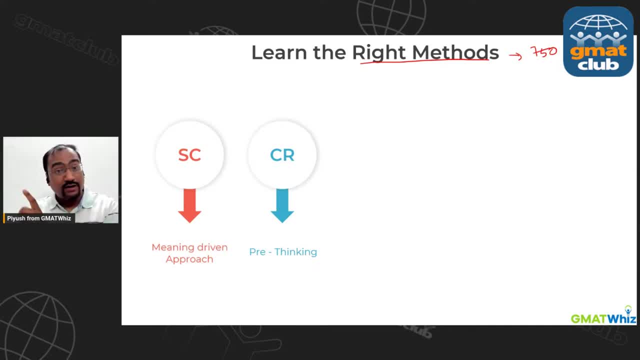 a lot of people improve their verbal score, so do stay tuned. uh, it's gonna come on the 25th, uh, most likely of this month. uh, we will have a session on critical reasoning thinking around that. so cr pre-thinking is important, not just running random pre-thinking, proper, structured pre-thinking rc. you have to involve yourself in the passage. 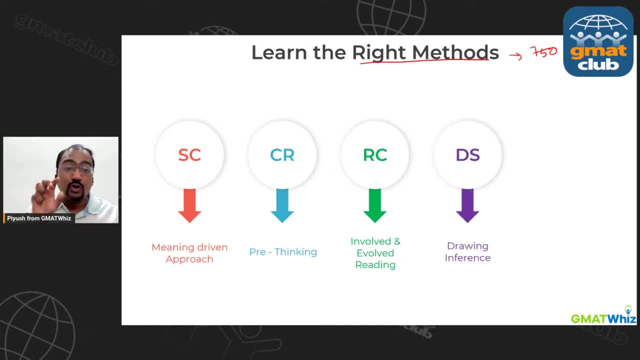 understand the passage as well. in data sufficiency, you have to draw inferences from the question set. that's a very big mistake. a lot of people do, and in problem solving you have to follow a three-step process: understand what is to be found out, what is given to you and create a 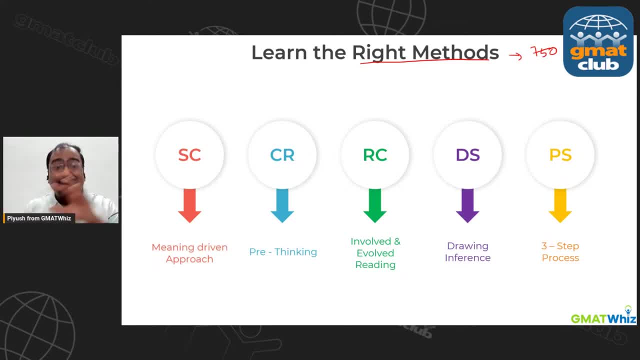 link between the two. there's a proper approach required for acing all the areas. if you have not learned these approaches, this method, you're not gonna improve your score. okay, so just take a note and if you have any questions- now anyone has any questions, please feel free to ask. 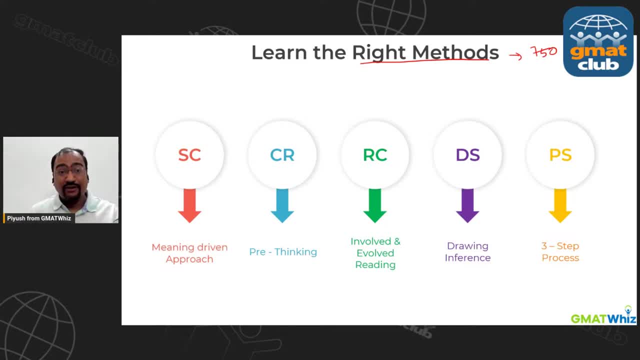 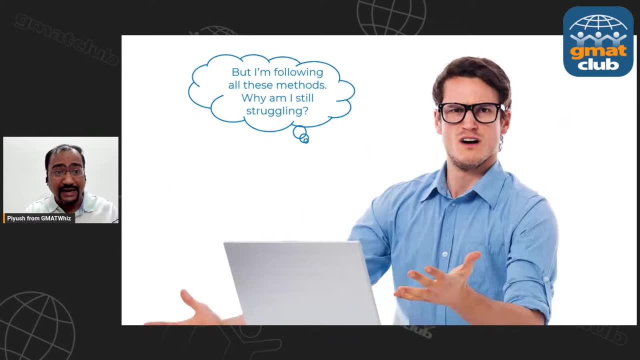 me now. i'm pretty sure at this point of time, many of you might be thinking: but ph, i'm actually following these methods, the methods that you're mentioning. right, i'm using cleaning based approach, i'm using pre-thinking, but i'm still struggling. why am i still struggling if these methods work? 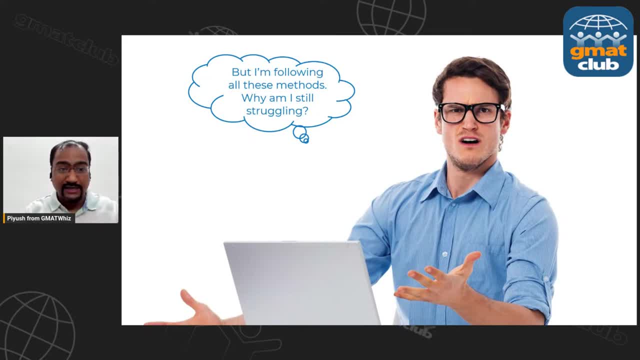 then why am i still struggling? this is a very common question i hear from people. people tell me all that all day long that, okay, you know what i use: cleaning based approach. i think about the meaning of a sentence and still i am not improving my score. now, what you need to understand is to follow the approach. you need to understand the approach also. 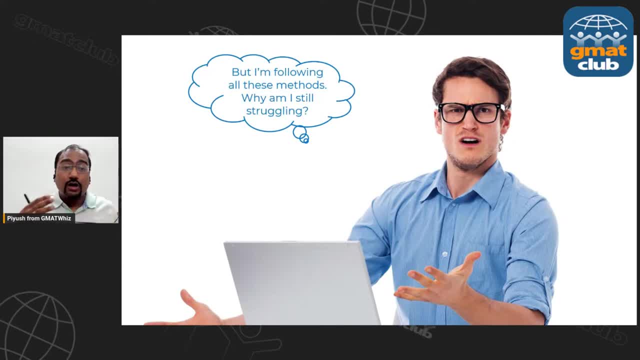 in many cases, people don't understand the approach correctly or they do not follow the approach correctly. many people are not even able to relate to the approach completely. so what i'm gonna do now is i'm gonna show you, just through an example, what is the right meaning based approach. so i'm 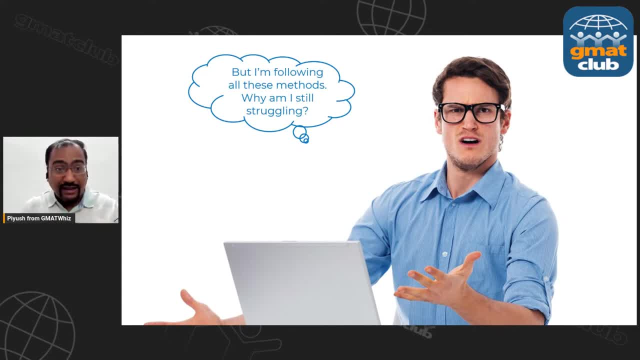 gonna just talk about some tense correction a little today. so what i'm i'm planning to do is i'm going to show you some of the things that you need to know and you need to understand. so my first question is: i will give you an official question to solve. this is the official question. 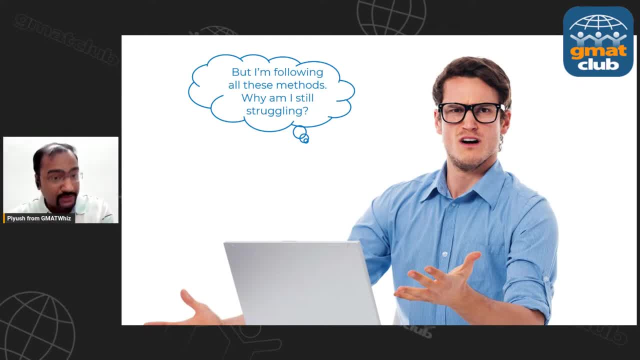 which i want you to solve. i'll show it again, don't worry. i'll go on full screen mode and show it to you. but i will give you an official questions to solve. give you two to three minutes to solve it and please don't post your answers in the chat. only post the answers when i ask you to post them. 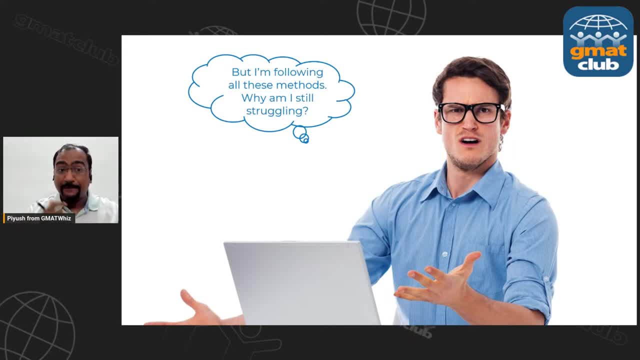 okay. so please, uh, stay quiet. if you have solved it, just note down the answer in your notebook. when i ask you to force the answers, then post it. but please understand my rationale for you. solving this question is not going to solve the question, to teach you how to solve that question or teach you sentence correction. the rationale is to help. 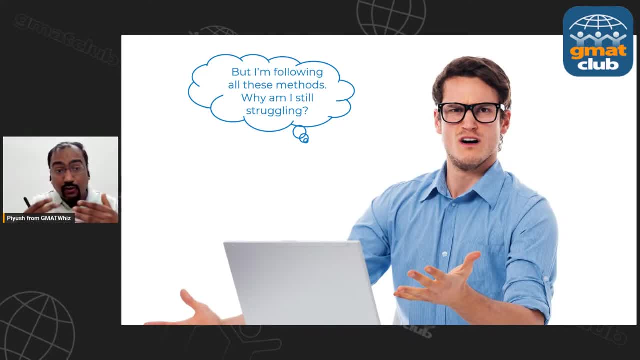 you understand what the right approach really means for those of you who really think that you follow the meaning-based approach. if you are really following it, i'll be very happy, i'll be glad. but for those of you who are not following it completely, it will be an eye-opener and open. 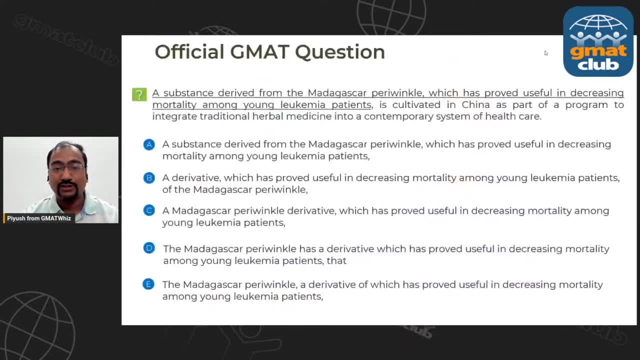 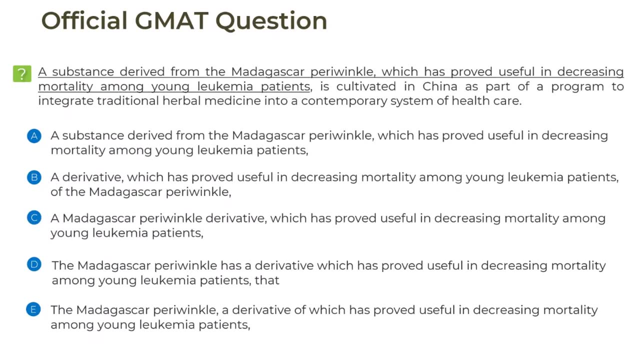 your mind towards it, okay? so, without any further ado, let's do this official question, okay, guys? so i'm gonna just do the uh uh, uh, just remove the logo for gmat club once and go full screen so that you can see the question properly. and, as i said, guys, don't post the answers right now. 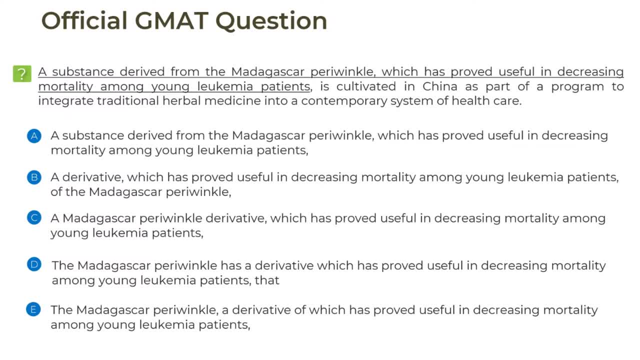 take your time, solve this question and when i ask you to post the answer, then we'll post the answer. so your time starts now. i'm gonna be on mute for approximately two, two and a half minutes and those who are watching this recorded. you can pause this video, solve it and and or, if you have, 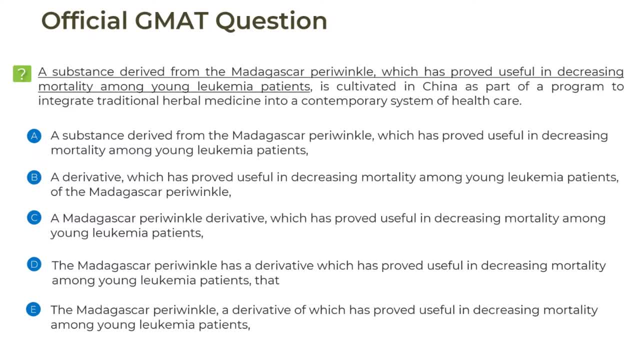 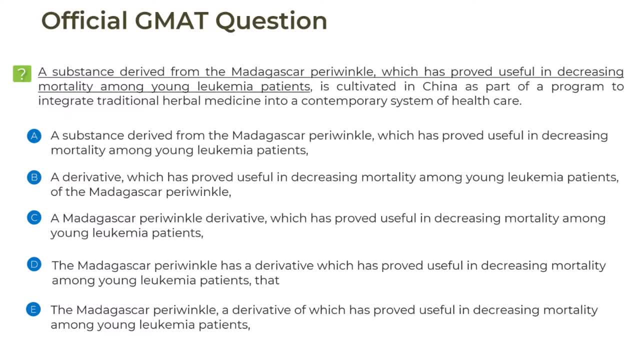 give another 10, 10, 10, 10, 10 seconds, maybe for you to post your answers, and then we are going to solve this question together. okay, and again, guys, uh, what i'm going to do now is i'm going to show you how i would. 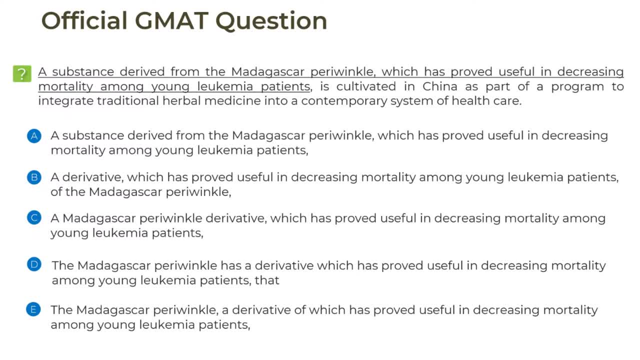 solve this question how. i would use the meaning-based approach in general time to solve this question and to help you figure out what should the right approach be and how you can do it yourself okay, so you can actually do a very good comparison then between how you solve it. so i want you. 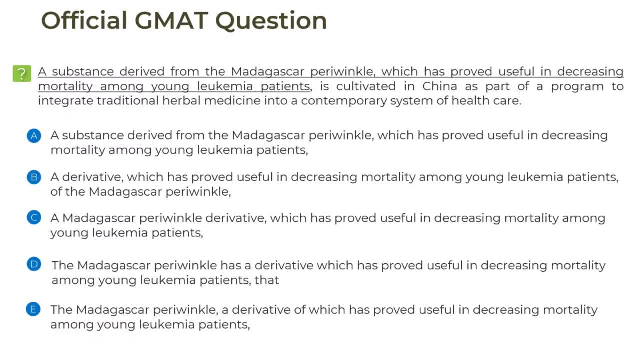 to look at your method, look at my method very, very closely and compare it with your method and later on, when we are done solving it, i want you to share your thoughts is in terms of what is that you saw in terms of the difference, uh, in solving this question, okay, so i have. 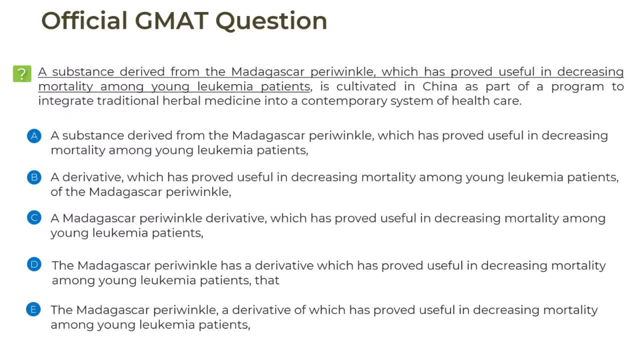 three people going for e till now. uh, community saumishta, miguel. uh, akhida goes for option b. shireen goes with option b. okay, what about others? narshan, also going with option e. okay, so e seems to be the most popular choice till now. uh, let's solve this question together. 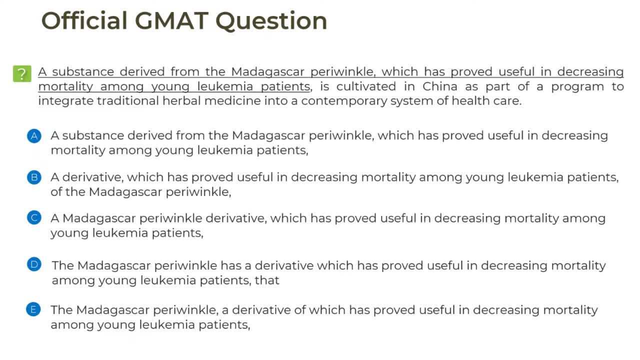 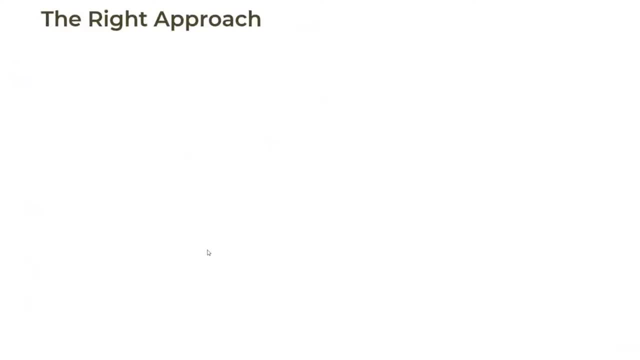 uh, please keep sharing your answers. that will really help in me understanding how many which people got to which question. uh, the options, uh. but in the meantime, i'll start solving this question. so when i talk about, when we talk about the meaning-based approach, the main thing that matters while solving- 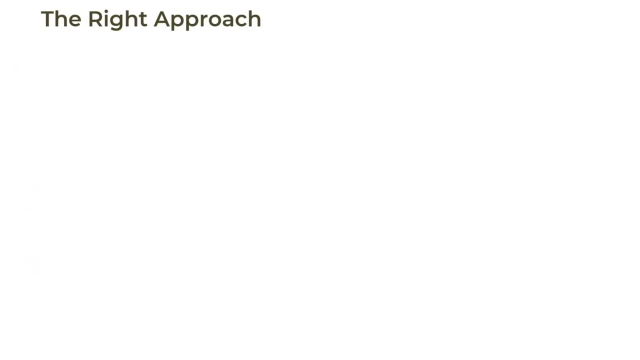 questions. using the meaning-based approach is understanding the question stem, understanding the meaning of the original sentence, and for that you have to break down sentences into small parts. you have to understand each and every part of the sentence. okay, saumishta says my sc is in 80 range, but i'm troubled in cr- how to improve. so cr, i'm not going to. 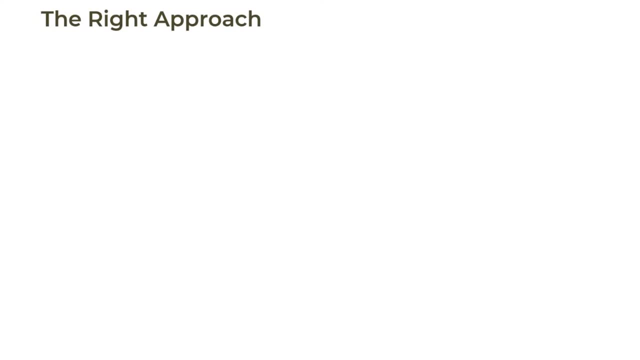 cover that today, and i was not supposed to cover sc either, but i just wanted to take up one idea to help you understand whether you're using the right approach. for cr salmista, you can go to the gmat list channel. we have a lot of videos that we have covered on critical reasoning. you can check it out. we have a free. 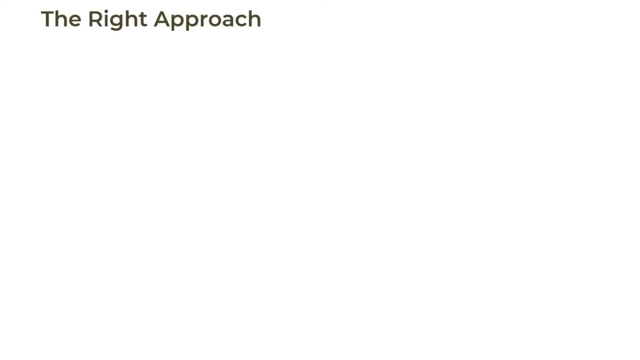 trial of our product as well, where you can actually learn some. uh like some get some free content to kind of learn some methods for critical reasoning. but if your approach in critical reasoning is wrong, then working on the approach part is important for you to improve your score. basically okay. so i'm just going to share the link to try our free. 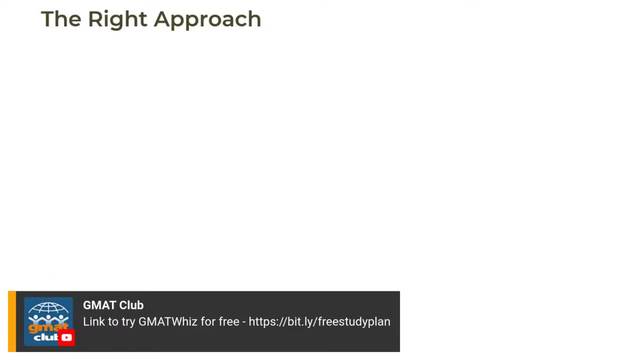 nisha, you can try doing that. so, nista, sorry, you can try doing that. this is the link which you can use to create a free account on our website and that should help you learn certain things, or you can wait for another couple of weeks. this live session is going to come on particularly. 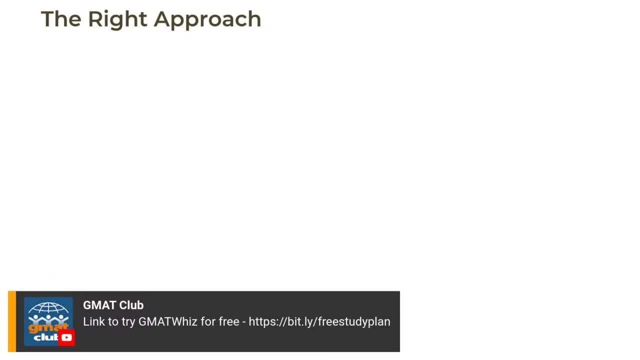 or you can go to gmat with youtube channel and find some other videos there. okay, so, if possible, i will also try to give some youtube links uh in the session, if possible to for cr uh, but yeah, let's focus on this question. so the idea is to read the question properly, break it down as we. 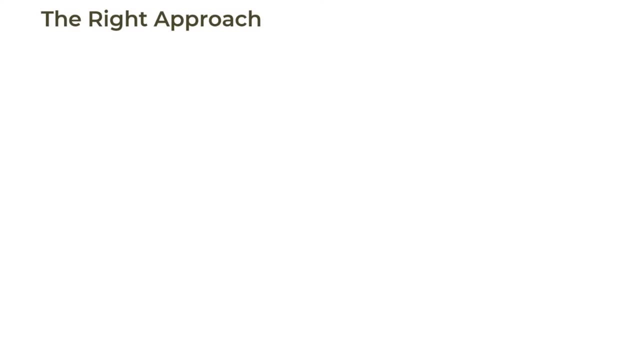 did it, so i see a lot of people going with choice c as well. now, uh, he is also more popular. uh, federico says i was stuck between uh a and c. i decided to go with c due to the modifier issue in me. okay, that's great. thank you so much for explaining that. now let's focus on the sentence. 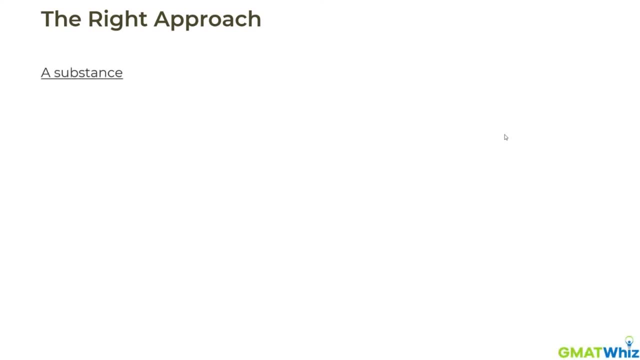 and let's see what is the right answer. okay, so let's read the sentence: a substance. okay, the moment i read a substance, i try and assimilate that. okay, the sentence is talking about something- a substance. what about the substance? i don't know, and i continuously ask these type of questions. 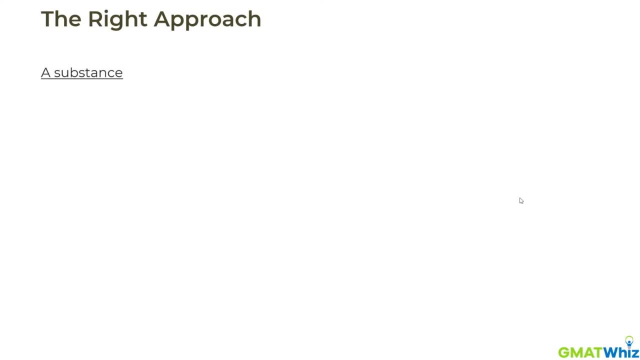 to myself, not just in sentence collection, but in every other area also. but let's a substance- let's see what comes next- derived from the madagascar periwinkle. okay, so this substance is something which is derived from madagascar periwinkle, let's call it mp. what is madagascar? 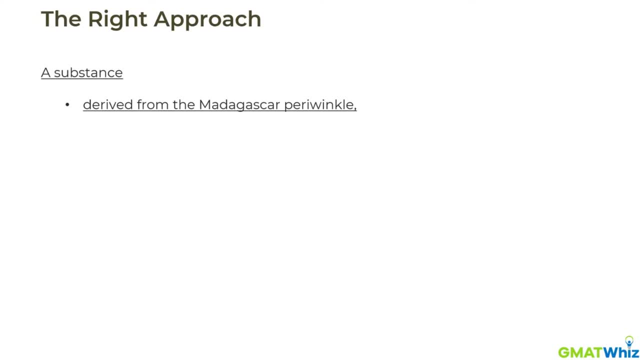 periwinkle, i don't know something in madagascar, i don't know what, but it's something with, like, it's something there, uh, substance is derived from it. okay, now, whenever we always recommend a gmat this, that you should pause at verb-like words. okay. 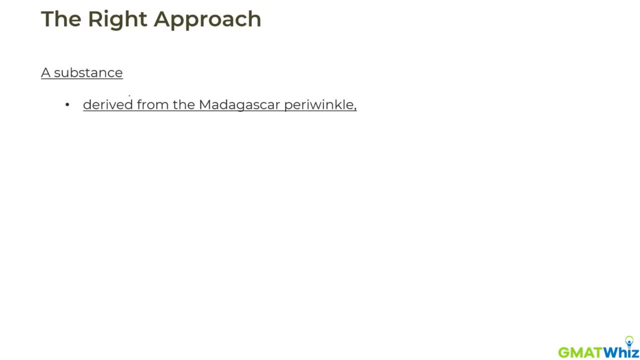 it's the words which look like work. so, for example, derived is a verb-like word. you need to understand whether it is acting as a modifier or is it acting as a verb. basically, that is something which is very important. so i'll ask this question: is derived? 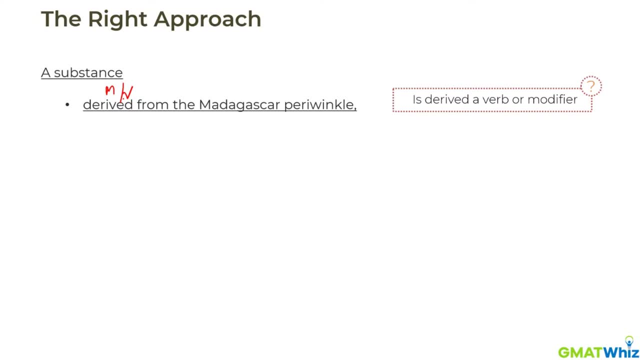 a verb or a modifier? it is actually a modifier. it is not a verb because it is not preceded by is. uh, if i say a substance is derived from the madagascar periwinkle, then it will act as a verb. now there are certain tests that you can use to kind of understand when a ed verbal is a verb. 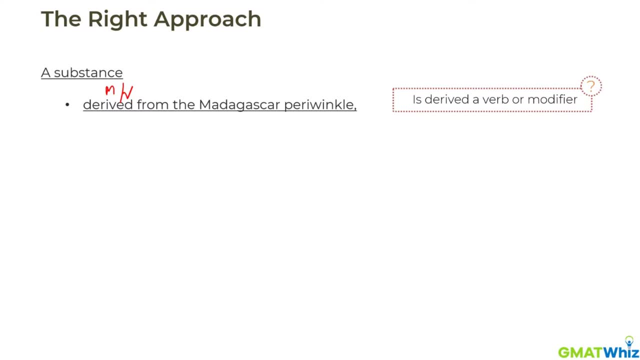 when it is not, and that is something which we have covered in our free trial also. so if you want to learn that, you can use that. there is a proper test that we use here. i'm not discussing that because i'm not teaching sc today, okay, but the idea is that, uh, this is a modifier, so i don't. 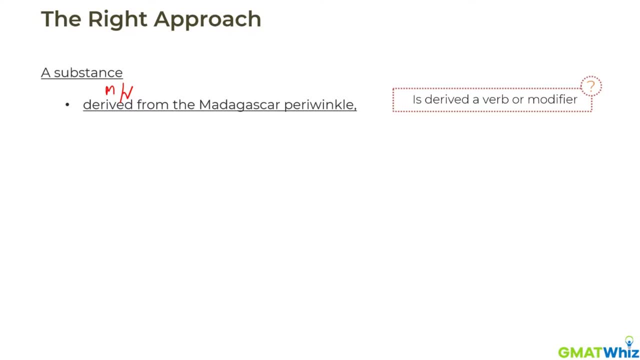 have a verb for a substance. now i understand that the substance is something which is derived from the medical scripture. let's read further. which has proved useful in decreasing mortality? in decreasing what? mortality? among young leukemia patients. so it has decreased the mortality rate in some patients, some patients suffering from some type of disease. but what has proved useful? 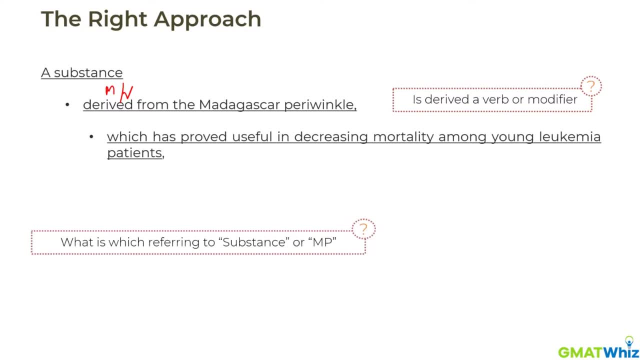 if i ask myself: what is that which referring to is the sub? has the substance proof useful? or has madagascar periwinkle proved useful? now, when i say structurally, which is placed next to mp so it can modify mp, it seems like it is talking about the madagascar periwinkle. but if i go by, 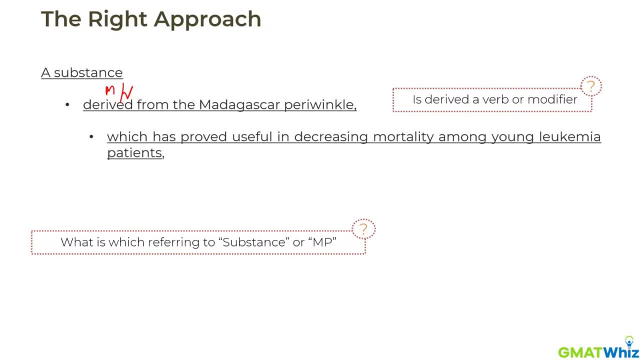 logic, a substance derived from madagascar periwinkle. if i'm talking about something derived from madagascar periwinkle, probably that is something which has proved useful, but the sentence is not telling me about that. it is not telling me what is which referring to. is it referring to the substance? is it referring to the periwinkle i? 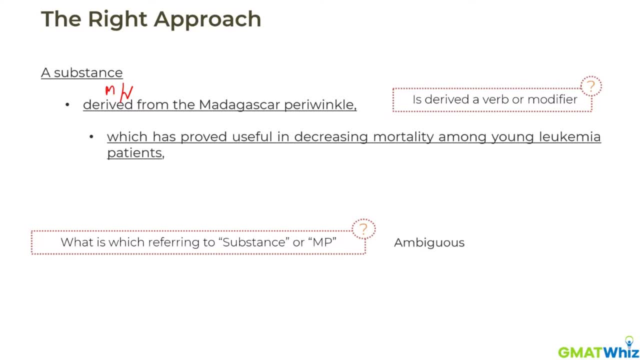 don't know that, so the part is ambiguous. this is a error which is there in the sentence, so i have found my first error. okay, let's read further. so in the right answer. i don't want this error. i don't want this ambiguity. the structure should be clearly telling you what is that which reflecting to should. 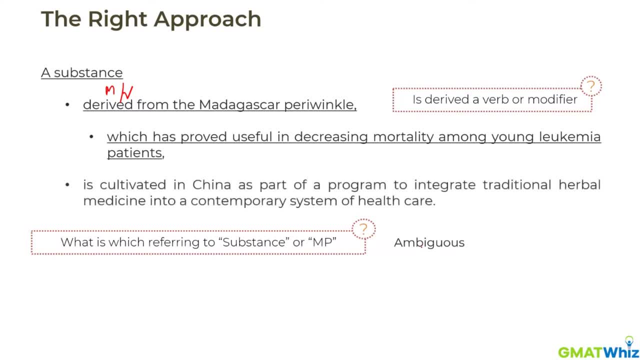 be referring to the substance. let's see it further- is cultivated in china. okay, so i now see the verb likely. this is related to a substance, so this tells us that the substance is cultivated in china. now when i see a substance and cultivated being used, i i feel a little weird, like how can? 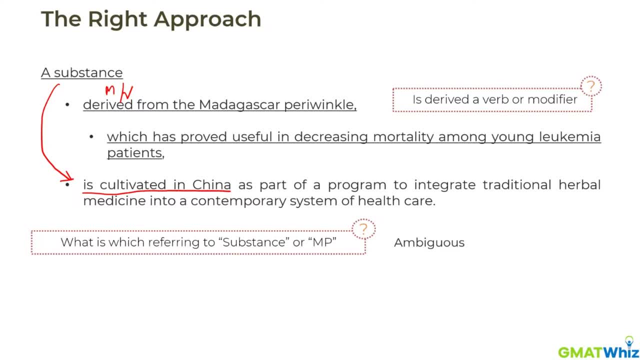 a substance be cultivated. we use the word cultivated with plants or something, right, but uh, can a substance be actually cultivated? i'm not sure. i don't think so. it should be that way. and we are saying the substance is derived from the madagascar, so probably saying that a substance 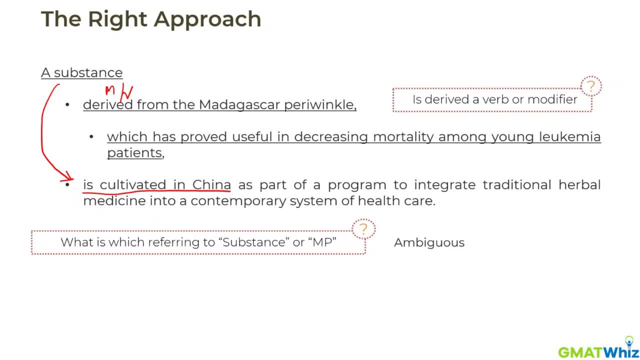 is cultivated is still wrong. right, if you are deriving it from madagascar perinatal, how can we cultivate it? if the cultivation was possible, probably wouldn't have derived it from madagascar either way. so i feel there is a problem with this. is cultivated in china, should not be. 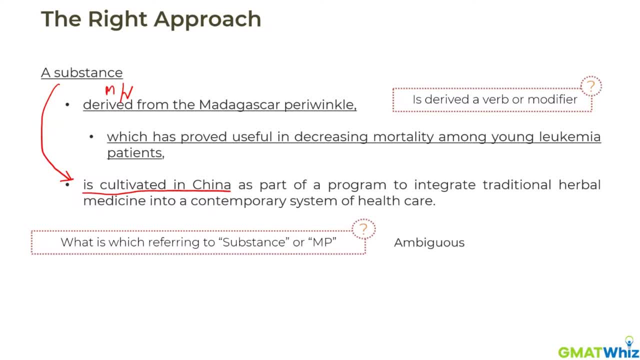 talking about a substance, but do we have another plant or anything which we can talk about here which is cultivated? i don't know. let's see it further. it's cultivated in china as part of a program. as part of a program, what is this program about? the program is for integrating traditional 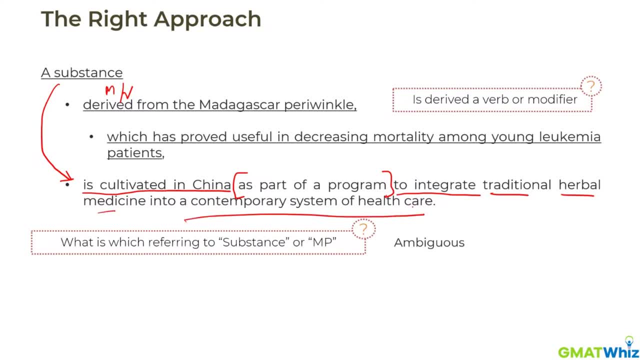 herbal medicine into a contemporary style of health care. okay, so integrating traditional herbal medicine into contemporary healthcare. now, what is herbal medicine? herbal medicine is something which is derived from a herb, right, so this could be the medicine. i'm talking about this substance being useful in decreasing mortality in patients. 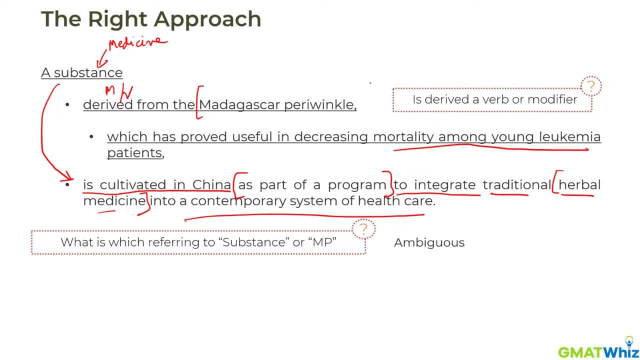 uh, this substance is the medicine and this is derived from what this, so this should be the herb that we are talking about. so if this is the herb that we are talking about, doesn't it make sense to say that it should actually be the madagascar perinatal, which is? 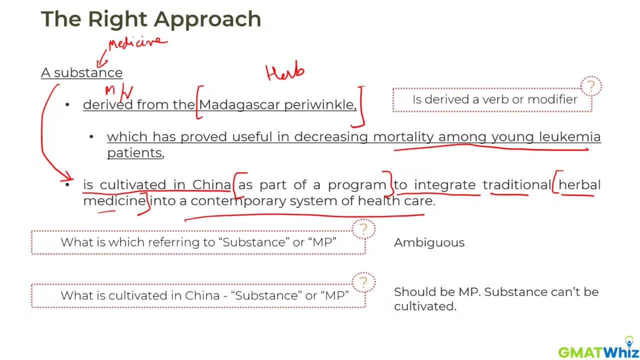 actually cultivated in china. it is not the substance which is cultivated in china, correct? this is how i would read the sentence. so i have my two errors. i don't want which to be ambiguous, i want which to be clearly modifying the right entity, and i know that. 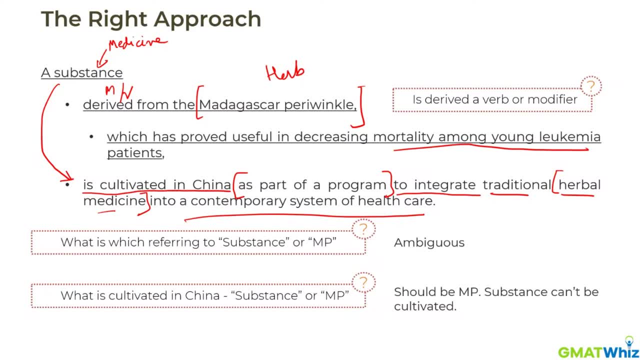 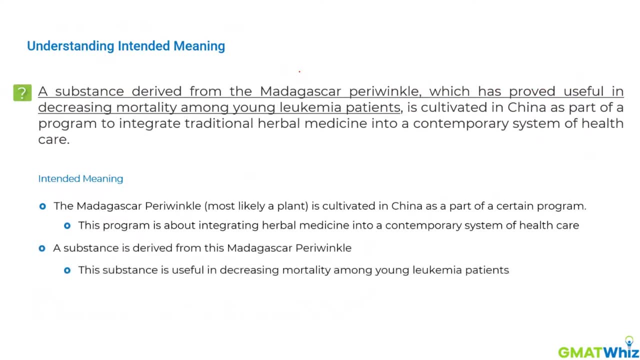 is cultivated should refer to madagascar perinatal. it should not refer to the substrate. okay, now let's look at the answers, basically. so this is the intended meaning. i've already talked about it. in option a, we see what are the errors. option b: a derivative, which has proved useful. so this: 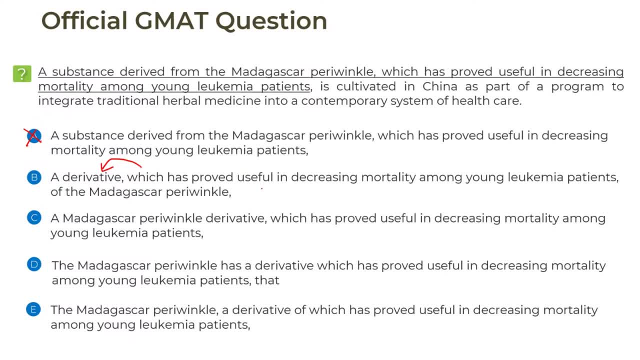 clearly tells us that the derivative has proved useful in decreasing mortality rate, but now it says a derivative is cultivated. so it still says the derivative is cultivated, which is not right. i need madagascar periwinkle to be cultivated. i need a choice which talks about madagascar. 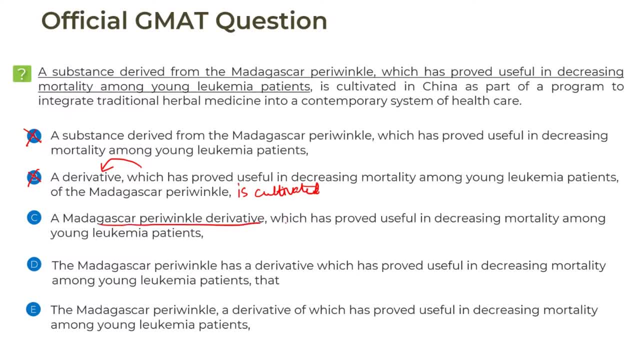 now let's look at the next sentence: a madagascar periwinkle derivative, which has proved useful. so this part is right. but it again says: is cultivated. so what is this cultivating referring to? it is again referring to the derivative, which is wrong. i need madagascar. 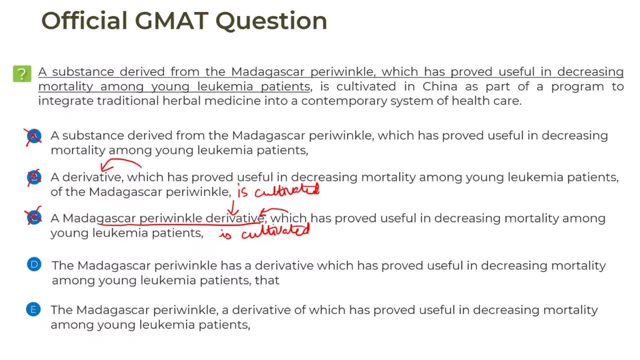 periwinkle to be cultivated. let's see it further. the madagascar periwinkle has a derivative which has proved useful. so this is again talking about the right thing. b is not picked by anyone by, by the way, but still let's look at it. has a derivative which has proved useful, uh, in decreasing mortality. 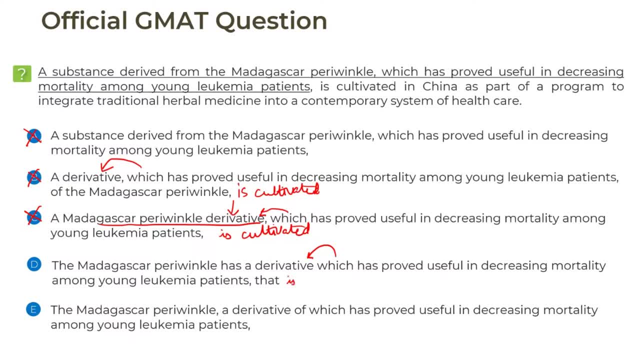 that is cultivated in china. now i'm not sure what is this that referring to it just still seems to, still seems to refer to the derivative, and i don't see which, and that to be connected very well. so this is the correct answer. so let's see what is the correct answer. so i'm leaving with the choice e. 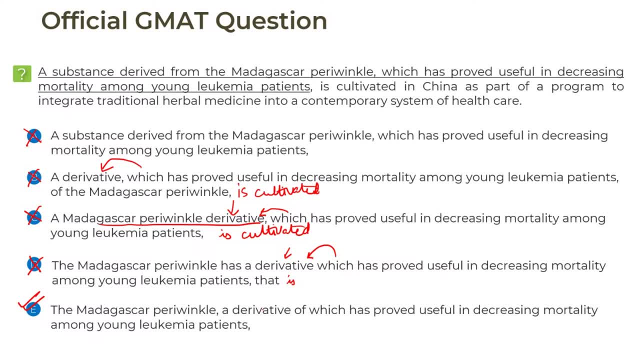 which should ideally be the correct answer, but i would still read it to see whether it is the correct answer or not. the madagascar periwinkle, a derivative of which has proved useful. so it clearly tells us that the derivative has proved useful or the substance it was derived has to be. 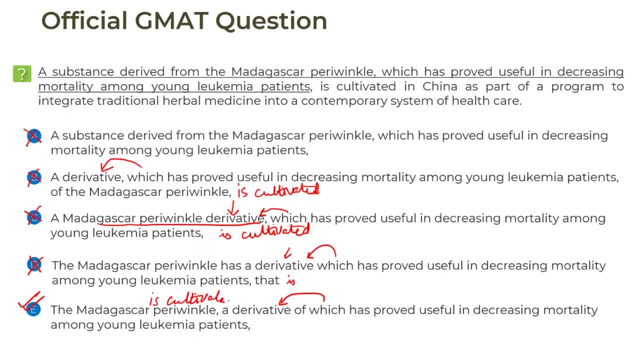 useful, and this madagascar periwinkle is cultivated in china, so this choice takes care of the intended meaning as well, so this is indeed the correct answer. so many of you got this and really, uh, congratulations for to those who have gotten this right, but what i want you to, 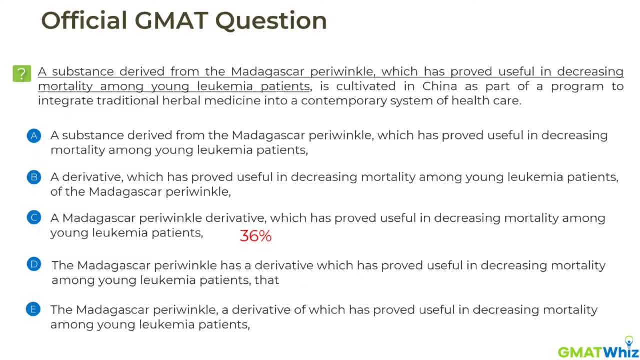 tell me now is the difference in the approach that i followed and that you follow for solving sentence correction question? i want you to tell me that in the chat here, because this is important, guys, unless you tell me what is the difference that you saw in the approach that i follow in. 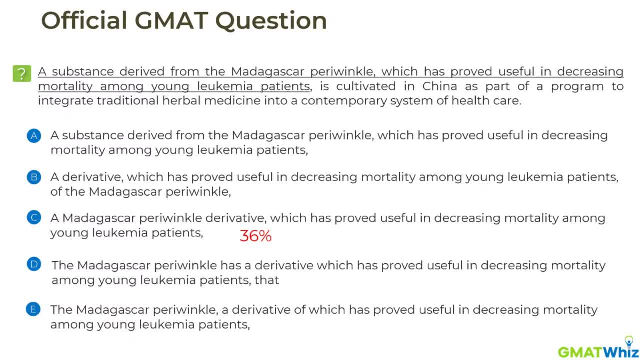 the post that you follow. the entire time i spent on this, close to about 10 minutes we have done given to this will be gone. based because the idea is for you to understand what is the right method to solve questions really mean, are you actually using the right methods? just thinking about the? 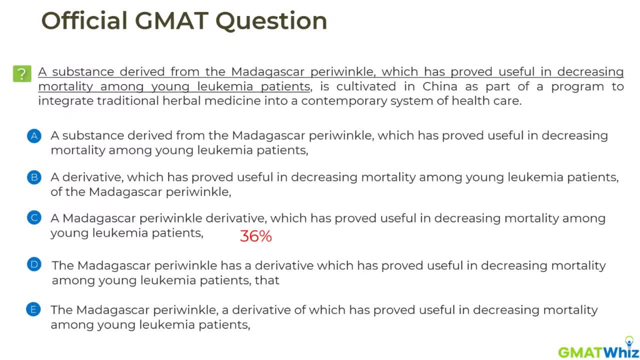 meaning is not appreciated. you have to break sentences down. you have to understand each part and see how easy it becomes when it comes to answer choice elimination. i hardly had to spend any time on answer choice elimination. i usually in gmat. if i look at my own esr, i scored a 93. 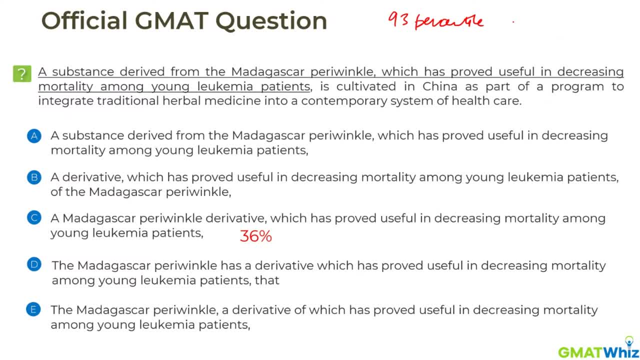 percentile in sentence correction? okay, and i ended up doing sentence correction questions in about one minute 15 seconds on an average, and out of this one minute length of time, i was able to solve all the questions in one minute 15 seconds on an average 15 seconds. i used to spend about 50 to 60 seconds alone on reading the original sentence answer. 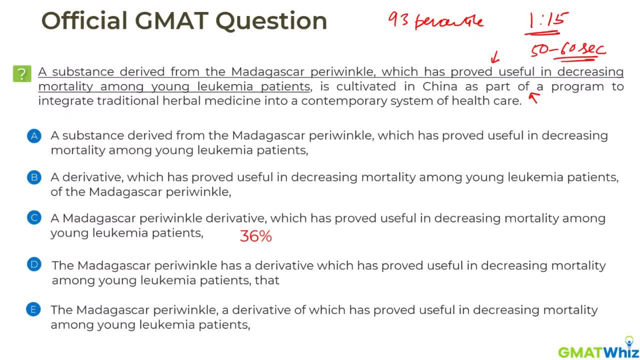 elimination hardly takes me any time because i focus on the meaning. i get the errors on the sentence, and that's when it is easy. i just have to pick the answer from the uh options, just like i do it in coin. okay, isha says this answer choice is one of those classics. sounds horrible to say. 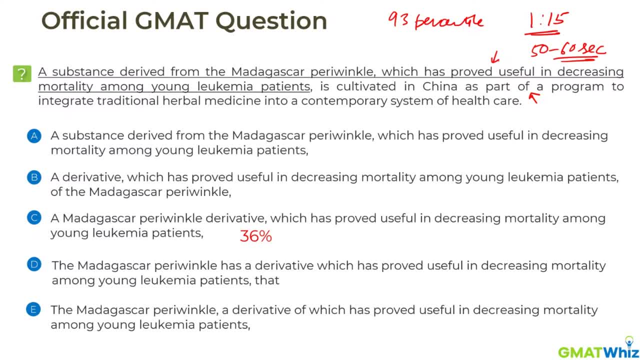 aloud, but it is technically correct. yes, so you should never go by your ear, isha. it should always be logically sound as well, not just sounding right to your ear. so stop saying that, okay, this sounds right, this doesn't sound right. that should not be the case. 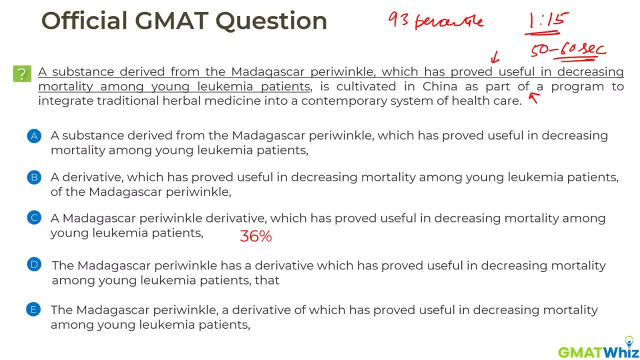 if it doesn't sound right, then why is it doesn't? why does it not sound right? it's important. derivative can't be cultivated. okay, community what? but what else did you learn that's more important? it's not just about this particular question. uh, this is a 700 level question, by the way. okay, so 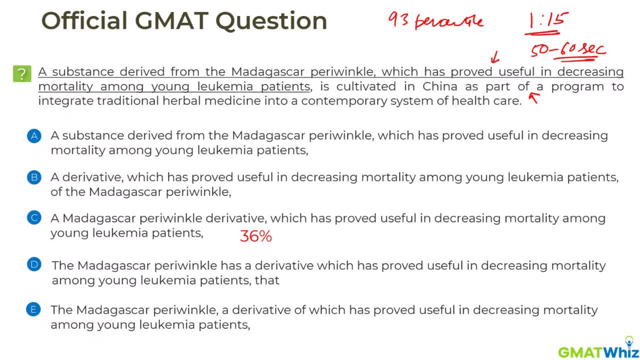 this is a 700 level question. uh, hard level question and i want you to understand you can't solve a hard question by just going through the option. if you just go through options, try to identify the splits in the options, use that approach. it won't work on hard questions. it will not work ever. you. 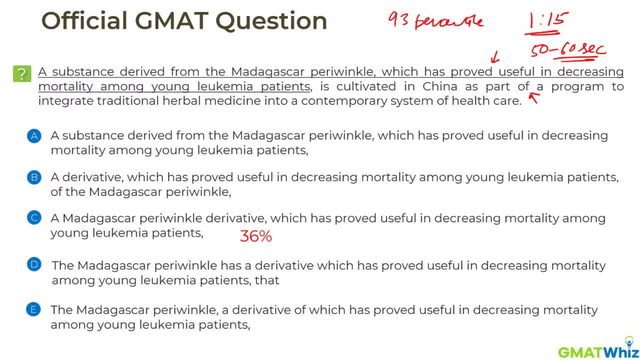 have to focus on the right approach. uh, amart says: missed in understanding the meaning of the sentence as a whole. uh, very valid point. what about others? what is the learning that you've got like? i just see four comments and out of those four also, just one is a. one is actually a question. three are: 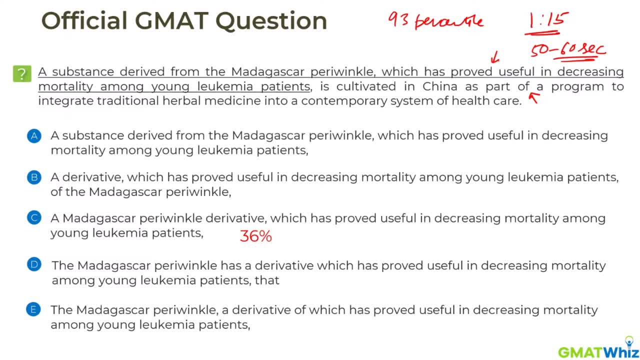 actually common? what did other people learn? what is the difference that you guys saw in your approach, the approach that i showed you? and just to show you guys, this is the difficult question. most people end up getting stuck with option c and a. these are the most common choices outside of. 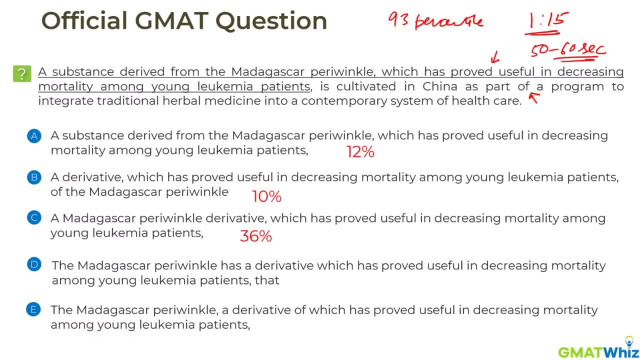 obviously my bad, sorry guys. outside of option. obviously the correct answer. a lot of people get this wrong and this data which i'm showing you is from gmat club, by the way. basically okay for this particular question. would you please minimize the questions so we can see you? yes, i'll, i'll be. 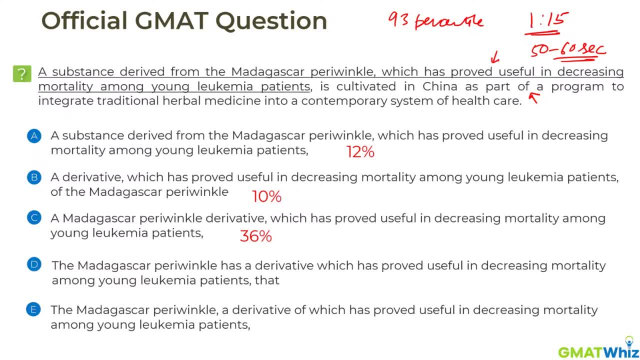 doing that right now, but i wanted your focus on this question right now, basically. so don't worry, i'm still here, i'm gonna show myself. i used a similar approach- really happy to know that, karki, that's still really great to know and i want you to do that. so the right approach to solve. 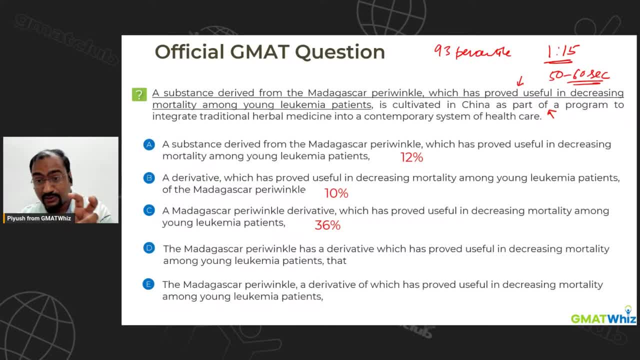 questions is to understand the questions properly. it's very important that you break down the sentence and rutuja again: you said that i missed the miscalculated error, so you can miss one thing, but what you need to understand is: why did you miss it? the moment you start thinking about why. 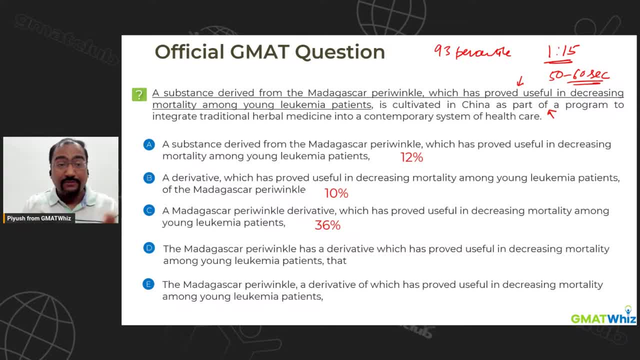 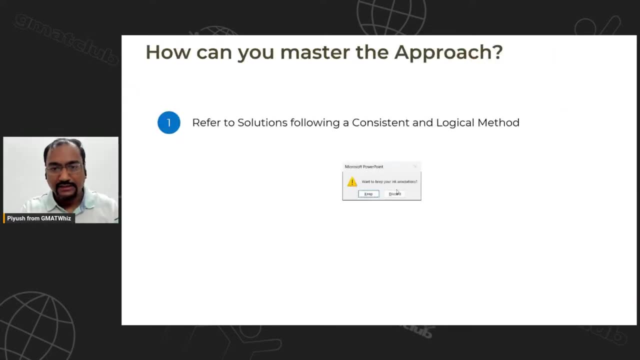 did you miss it, your score will start improving. the bigger problem is when we actually look at solution. we actually focus more on the what part, what went wrong, and that's where the problem starts, and i'll just cover that at the next slide. so let me actually do a small thing. just just give me a. 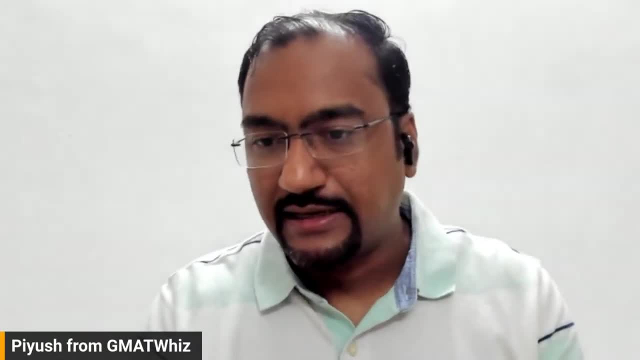 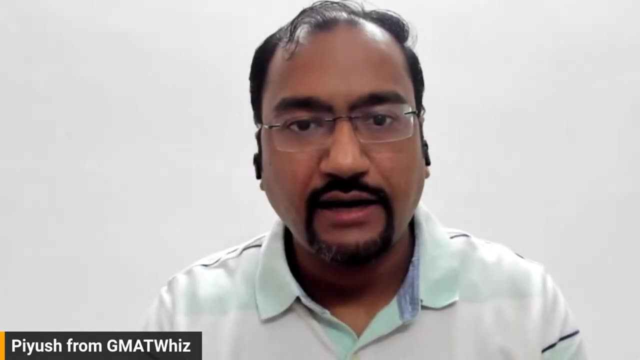 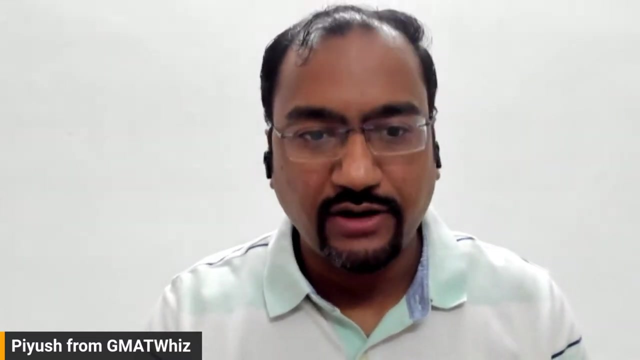 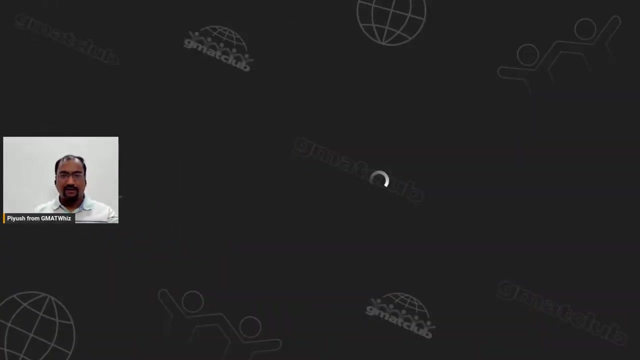 second guys, just a second, and just for now, give the slide a bit. all right, wait. so now i'll just bring back the slide again. just wanted to make a small change in the slide. okay, there we go. should be visible now, all right. so satyaki say, satyaka says breaking down the question. stem before jumping to option. 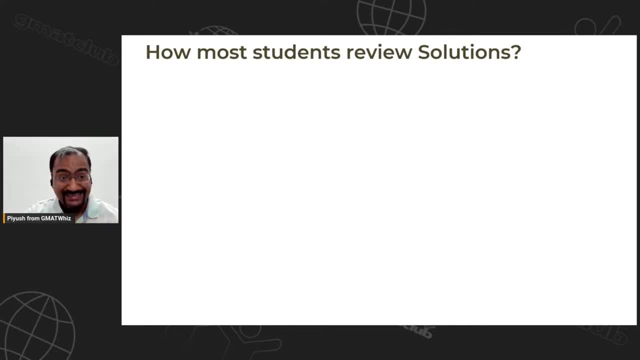 choices. very well said, satyaka, and i wanted all of you to understand this particular part. now, when it comes to solution, see if you can understand this particular part. now, when it comes to solution, see if you can understand this particular part. now, when it comes to solution, see if you can understand this particular part. 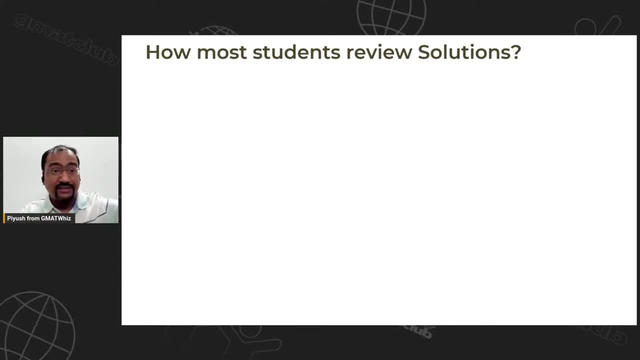 methodology is very critical. on gmat, i told you all of that. i showed you a lot of examples. hard questions: you can't get right without the right method. but how do you develop that methodology? so one part of it is to know the methodology then, and that is the easier part, like you will have. 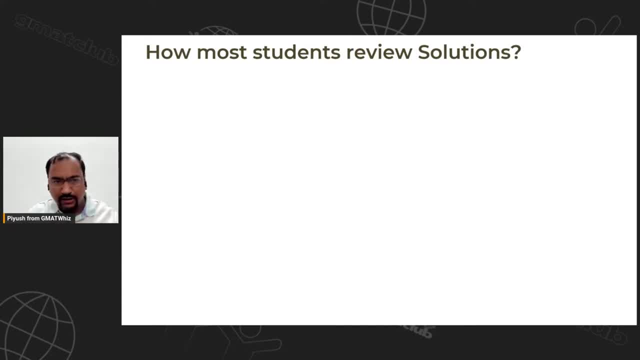 sessions, you will find a lot of people talking about it and you will learn the method, probably. but the more problematic thing is to follow the method consistently. and in order to follow the method consistently, the most important thing you need to do is you need to review the solutions in. 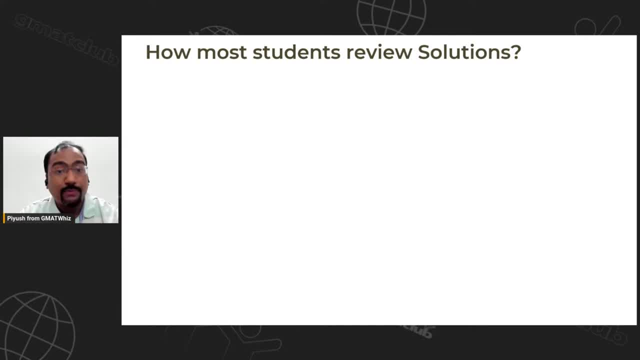 the right way. most people don't do that. how do most people review the solutions? they would directly jump to option choices, and one. one reason could be why this happens. probably is also because an official guide will just see option analysis right and in many, many cases, in uh, multiple. 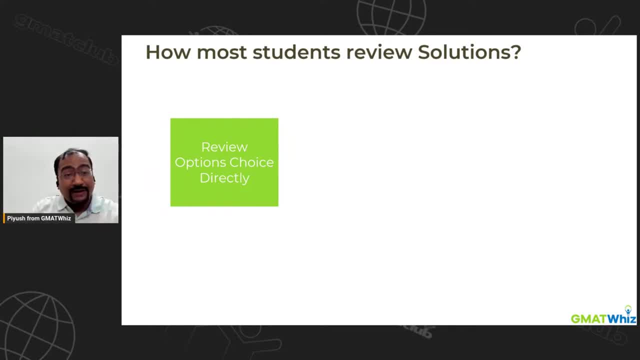 forums also, people just focus on option analysis. so what many people do when they look at solutions is they will directly jump to choices. that, okay, what's wrong with choice a? what's wrong with choice b? what's wrong with choice c? let's look at that. and when they do that, 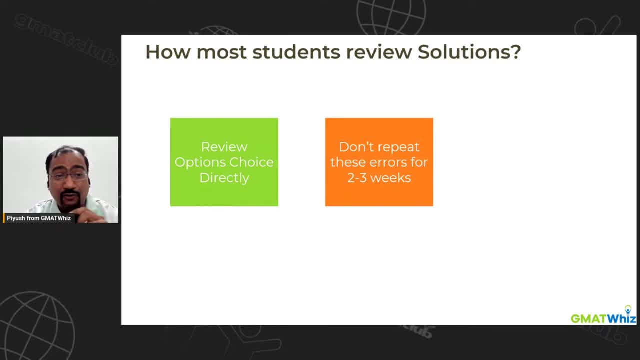 they memorize the error that. okay, this time i did not focus on the verb, like i did not focus on this continuity. this time i did not focus on the word tense. i have to be more careful with simple past and present. uh, past, perfect time. i have to be more careful with that error. so we 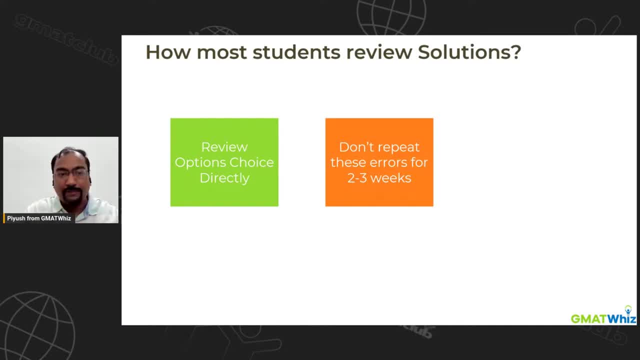 try to remember the errors that we don't, should not be making and because of which our score improves for a small time. because we don't make these errors right for two, three weeks, because we have just analyzed the solution and we have understood that we have to stop making this error. so, for two, three weeks, your errors. 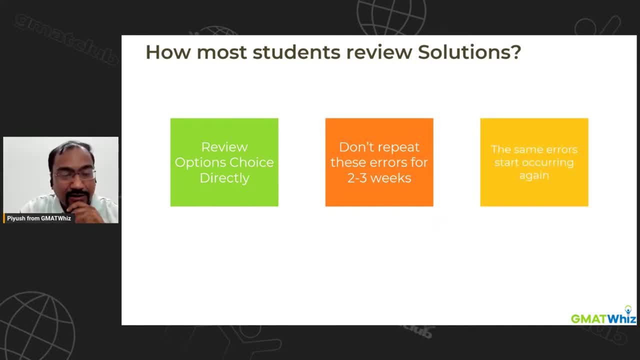 won't repeat, but after that the same error start repeating. how many of you face this problem? but for some time your players don't repeat, but after that you start repeating the same errors. just say yes or no in the chat. it's a very important question i want to hear. 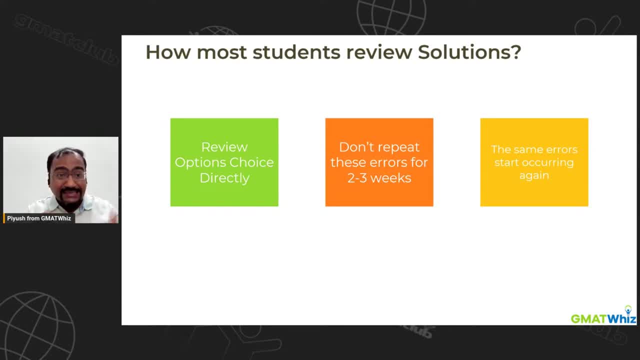 from you guys, if i'm making sense, if i'm able to present something which really happens, or i'm just blabbering, i'm just giving you some random damage which is not even true. okay, so isha says: yes, at least there is someone who says that, yeah, this is happening with me. 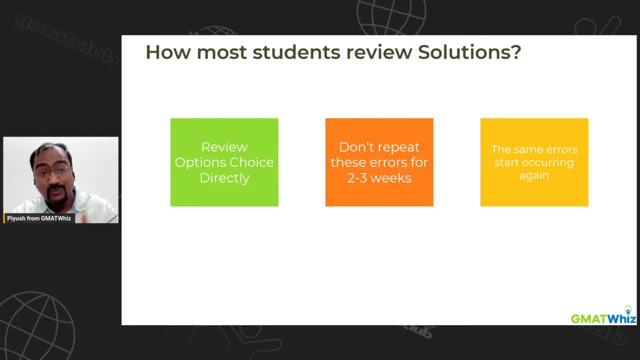 now all this? what i'm saying is from my own perspective as a student. i face these things myself and i see a lot of people coming to me and telling this to me. gargi also says: yes, this is, this happens to me as well. we need to understand why this happens to you. why does this happen? 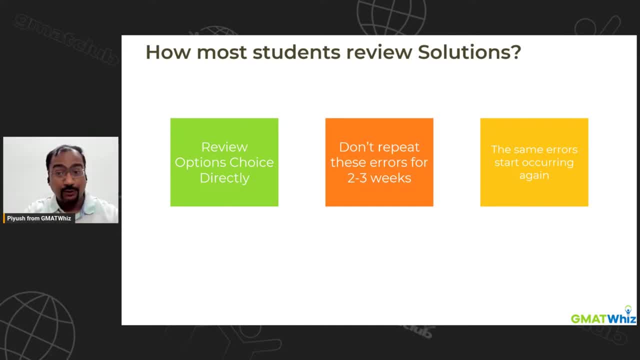 why do you end up making the same errors? the reason i'm going to tell you today, the main reason why this happens, is because what you are doing technically is not trying to memorize or things that you should not do correct. you are trying to remember. i should not do this, i should 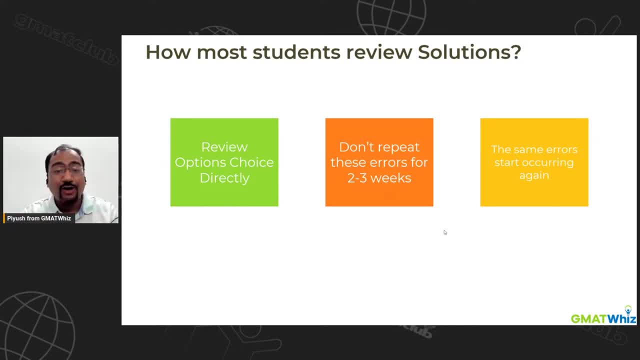 not do that. x, y, z, whatever. and on gmat, you cannot focus on 200 things that you should not do. your error log might say: okay, you are making this 10 errors or 20 errors or 50 errors or 200 errors. you cannot remember 200 things that you should not do. you can only focus on one thing that you. 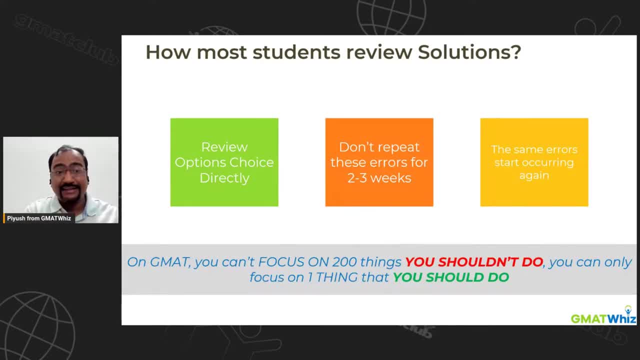 should do. that's important and that one thing that you should do is reading the question completely, so you read the question properly, the meaning based approach. if you do that right, you will not miss the simple pass versus fast perfect, you will not miss the subject verb you. 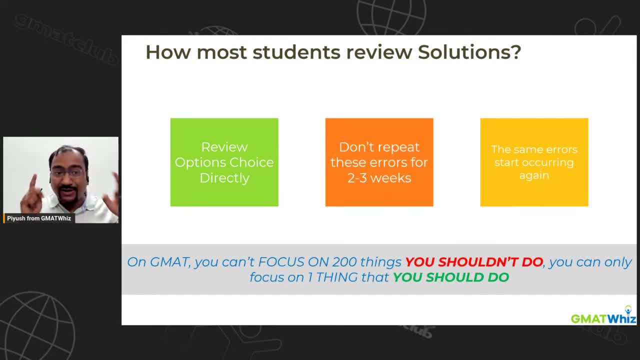 will not miss the pronoun agreement. you will not miss any of that because you are focusing on every element. you are not just focusing on the underlying portion, you are focusing on every element. you are understanding it completely. is that time taking? initially, yes, but once you use, 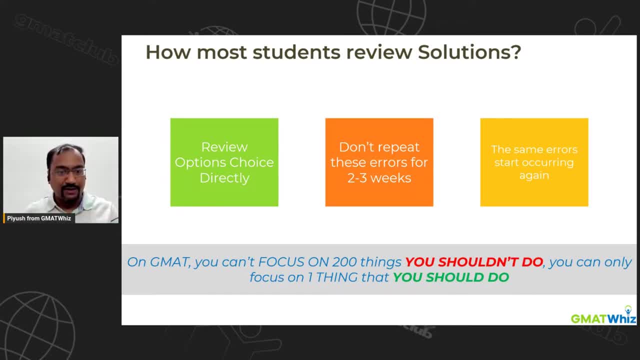 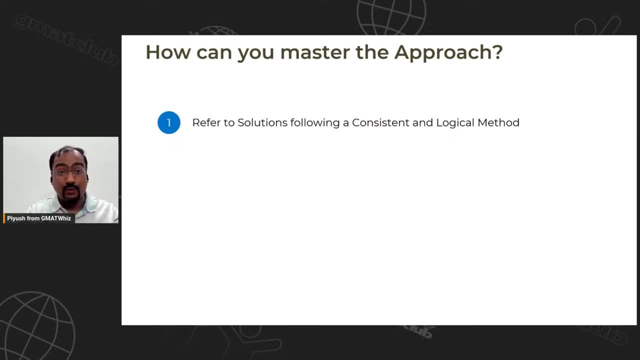 that approach, the time will also reduce, so that's the best way to go about timing also okay. so the main important thing to master the approach, to learn the approach, is to refer to solutions. you need to make sure that you spend time on solutions and when you look at solutions, look at solutions. 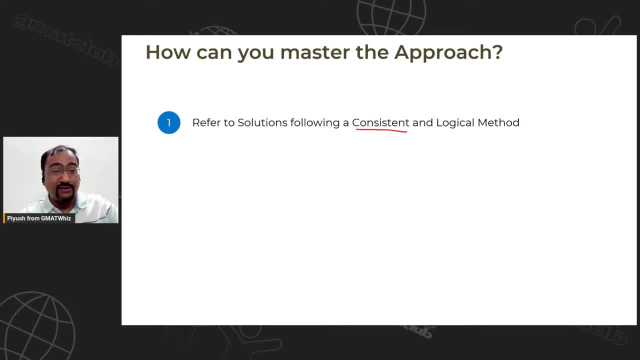 which are consistently using the same method, because if you are referring to one solution which uses a one method, then you refer to another solution which produces another method will be confused. and the method should be logical. it should not be shortcut based, it should not be eliminating choices. it should tell you a logical method of solving. this is very, very important. the 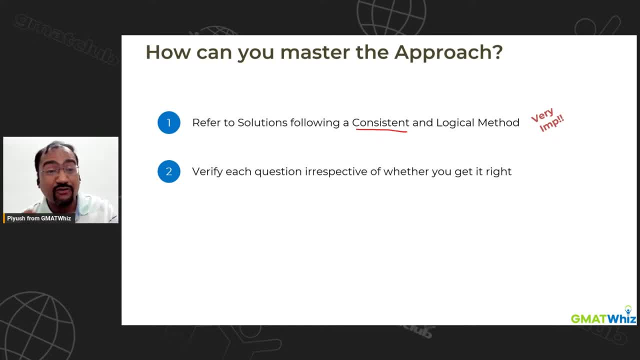 fact, then verify each question, irrespective of whether you get it right or wrong. now this might sound very rudimentary or something, but this is the key to improving your score on gmat. if you really want to improve your score, you have to review the solution when you have to improve your 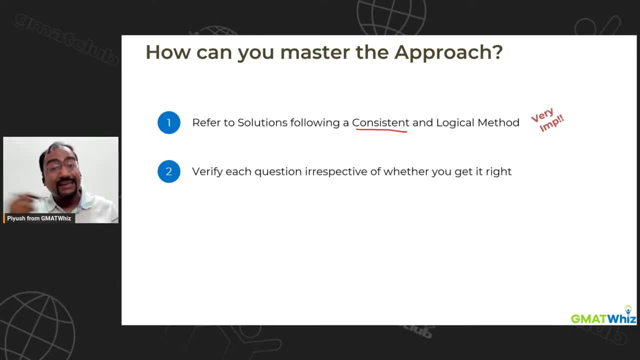 approach and make sure that you give you each question, irrespective of whether you get it right or wrong, and spend your most of the time in the review part on the question stem, whether it is a sentence or an argument or a passage. make sure that you spend time on that, don't jump. 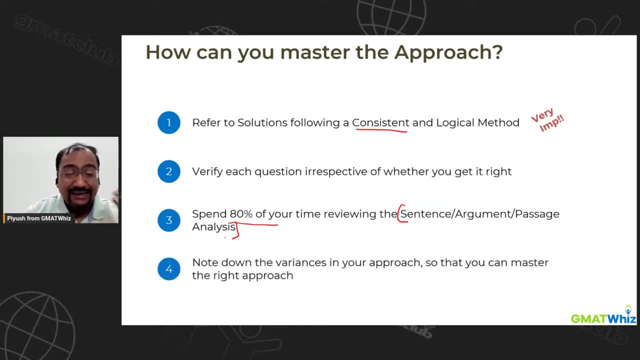 to options. try to see what was your understanding. try to draw the variances in your approach to with the right approach. try to understand what is the fact that is very, very important. okay, when you do that, you will start building the right. now many of you might be thinking: how do i do this? how do i? 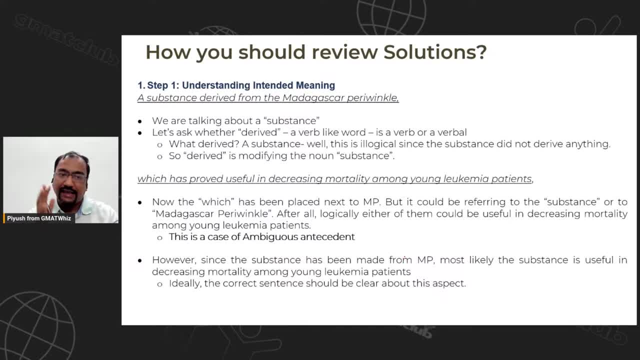 get to those logical methods again, gmat. this is there to help. in every single gmat risk question you will find that the solutions are very detailed. for example- i'm just showing you an example over the same question that we did- you'll find gmat with solutions presenting your line of reasoning. 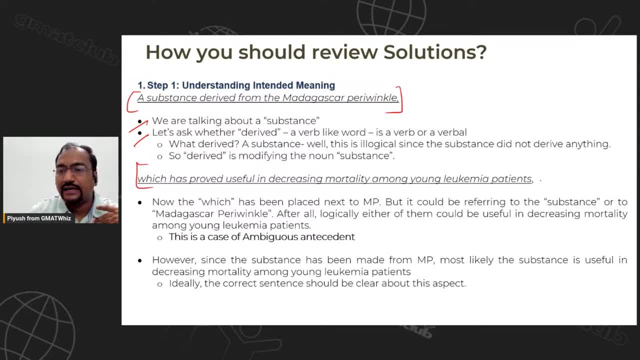 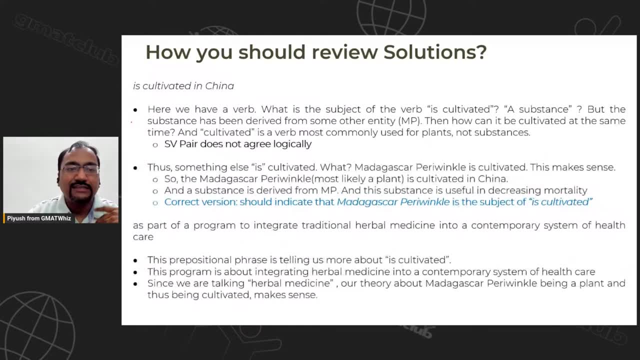 for each part of the sentence. each part of the sentence is presented in a detailed fashion so you can go through this line of reasoning and you can understand that. okay, when i was reading the sentence, did i understand it in this fashion? did i understand this part of this fashion or not? 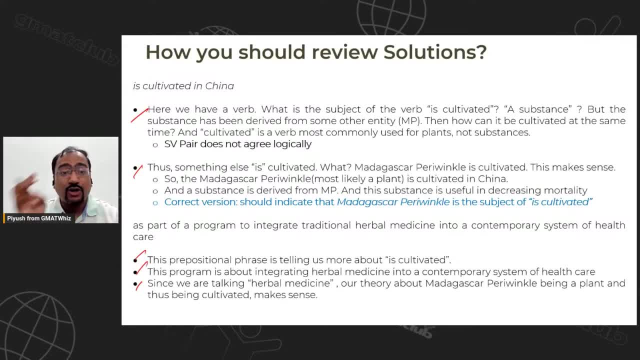 and that's where you will be able to relate that. okay, i did not break down the sentence enough, i did not focus on this part enough, and all this will help you in actually understanding where you are going wrong right now. obviously, if you are not uh able to use the meaning based approach, 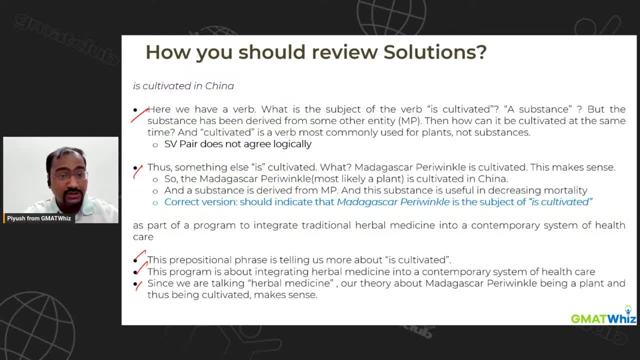 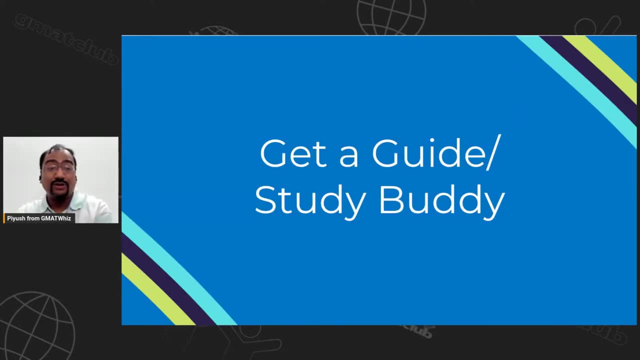 initially it's okay, but if you review the solutions properly, you will understand what the meaning based approach really means, or, for that matter, pre-thinking in cr, so you will be able to understand those things better understood. so this is very, very critical, the most important thing. the next thing that you need to improve your gmat score. i'm just shifting to the next. 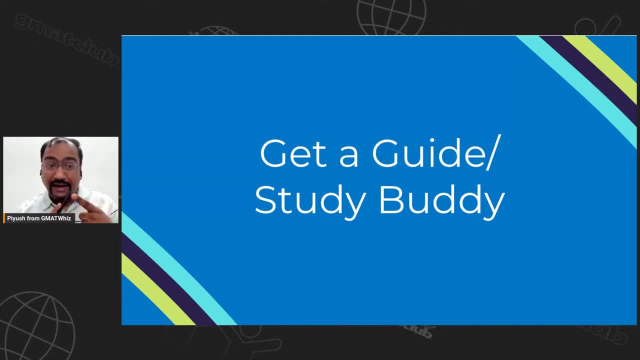 uh, the fourth tip actually. so i've already talked about three things. okay, the uh right real problem. the real problem is basically not focusing on consistency in hard questions, but rather focusing on more practice. that's problematic, uh like, and that happens mainly because of, like, hard question accuracy is low because of your wrong approach, so solution is to learn the right. 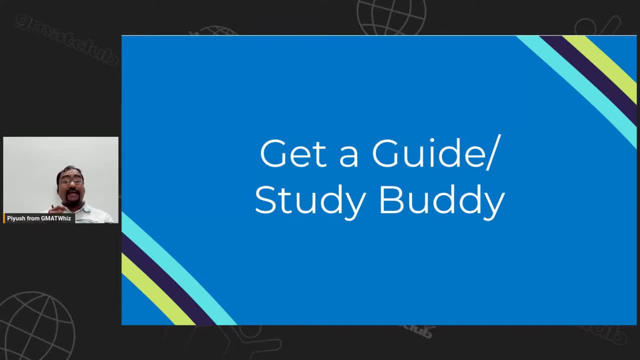 approach. and third, to implement the solution in real time. you have to ensure that you review the solutions carefully every single time and match your line of reasoning with the solution. okay, to improve your gmat score now is to get a study buddy or get a guide, because when you actually 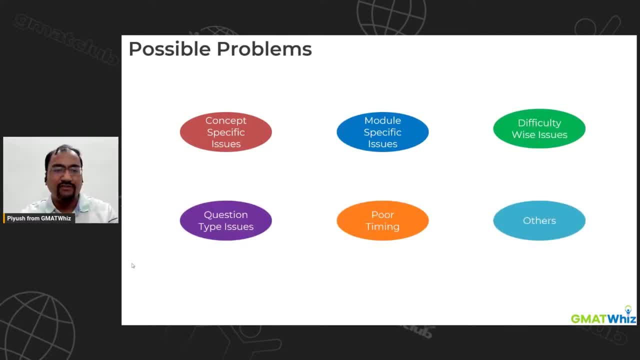 when you're struggling with your gmat score. it could be because of multiple factors. it could be because of simply concept specific issues- you might not be good at specific type of content. it could be because of module specific issues, that it is critical reasoning or reading comprehension or 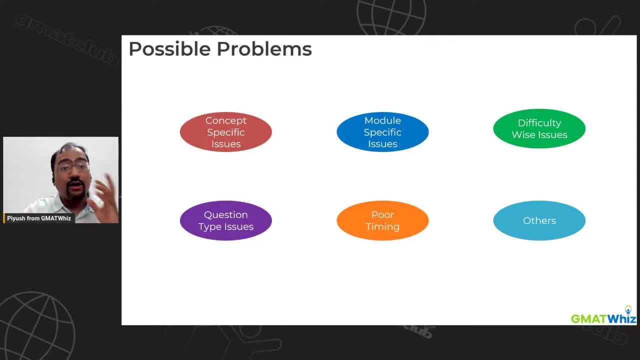 or data sufficiency or word problems or algebra or maybe data insights, which is actually creating trouble for you. it could be difficulty, wise issues that you are doing well or easy and meeting questions, but you are not doing well on hard questions. or it could be because of question types, but you are not doing well on data as efficiency or you're not doing. 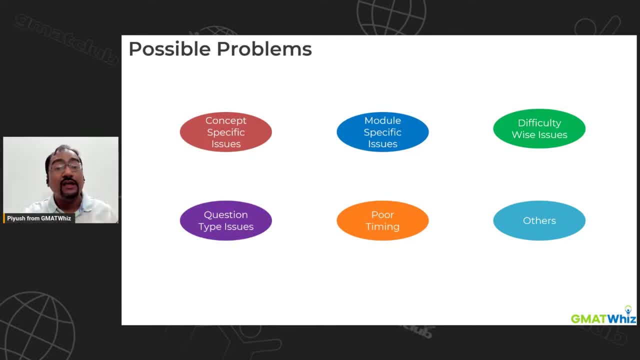 well on paragraph style questions where you have to read a lot of information. it could be because of poor timing, it could be other reasons also, but when you work with a study guide, we are able to give you that third person's perspective because you yourself are so busy in gross, so engrossed in. 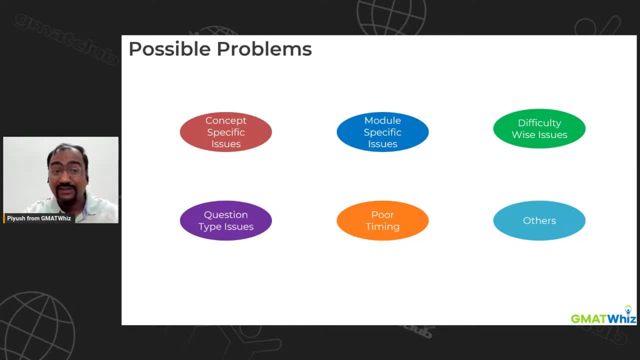 your own preparation. sometimes you are not able to distance yourself and see it from a different view, so sometimes a study buddy or a guide will be really helpful. so either get a guide or get a study buddy, someone who has a complementary skillset, who can guide you- and at gmat this. 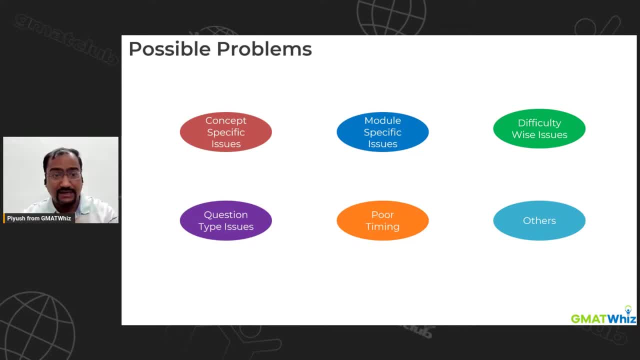 we provide study guides to every single student study but, like study guide, you have a mentor support for every single student. uh, we can help you out. you can schedule a call with your mentor every 10, 15 days, understand from them where they are going wrong and just to tell you about this. 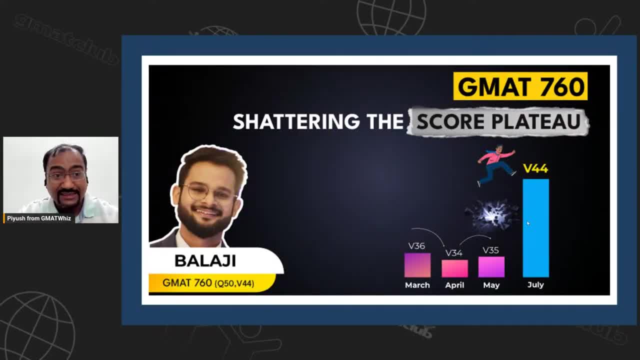 uh, i'm going to talk about a little about balaji. this guy story is very, very interesting. i i did an interview with him a little while back on gmat club, i think what one one almost a month back. that it is his interview, so his story was very unique. 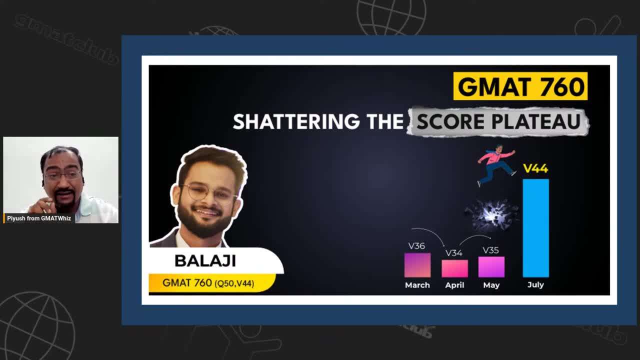 and the reason i'm taking this example is for you to understand what can be actually done with the right guidance, what can be actually done with the right thought process and aligning your thoughts, like allowing your studies in the right way. so balaji prepared for gmat for six months on using 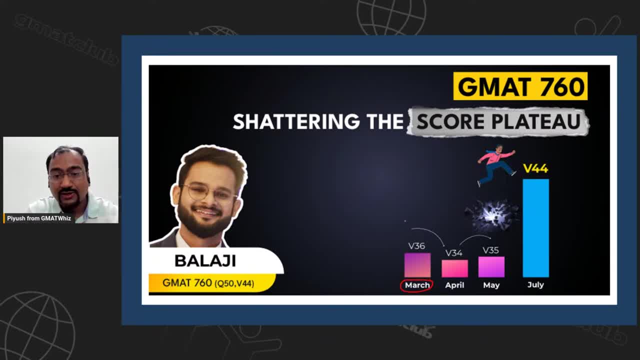 and in march he took his first attempt on gmat where he scored a 710- okay, and this was like after six months of preparation- okay. and then he scored a verbal 36 with 710. he did not get his standard score. next month he tries the gmat again, prepares for one more month, twice the gmat. 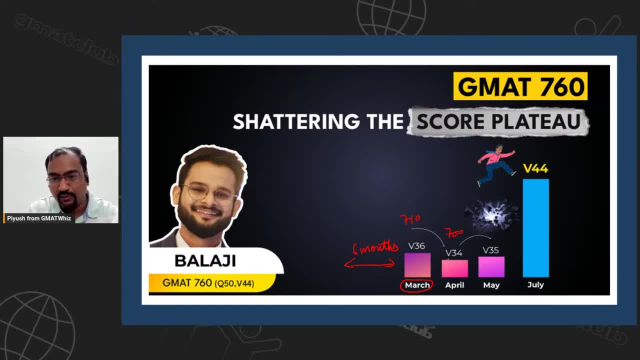 again gets a 700, this time verbal score of 34. okay, next month in may again twice. the gmat gets the 700 on gmat with a verbal 35. so what i'm trying to show you is that after six months he achieved a verbal 36. he got stuck at the same score for three entire months, kept on preparing, kept on. 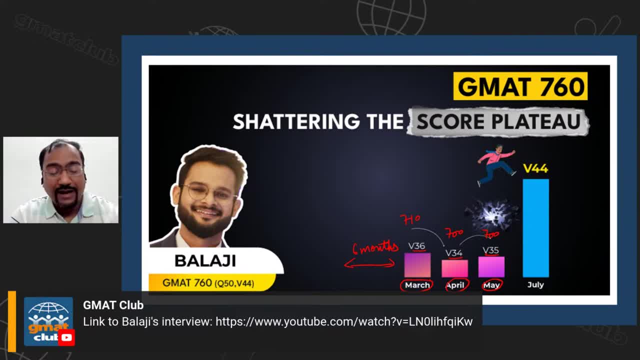 preparing scores were not cheap- had a score platter. he was not able to understand what was the core reason why he was struggling. then he came to us at gmat test. we took our private tutoring service for verbal. we were able to help him improve his score in the very next attempt in. 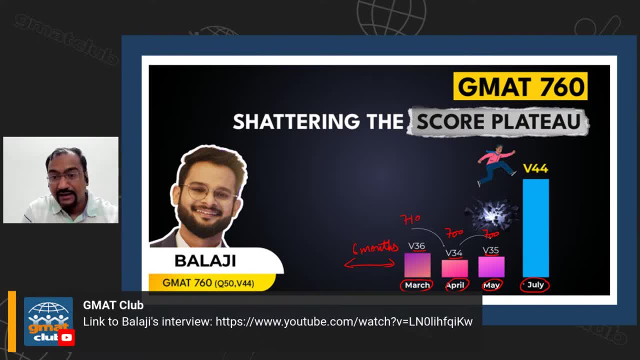 just the very next attempt in the sport attempt overall in a couple of months, and his score in verbal didn't improve by one, two point, one point or two point. he was able to increase his score to a 44, a massive verbal 44 and, by the way, 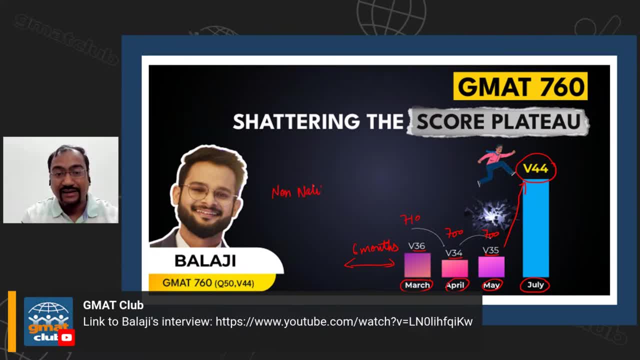 this guy is a non-native speaker, studies his entire life in india. uh, a non-native speaker scored a 760. the same person who was stuck with 700- 710 for three entire months and before that he had prepared for six months. so that was the impact of right guidance. he worked with sunita man. 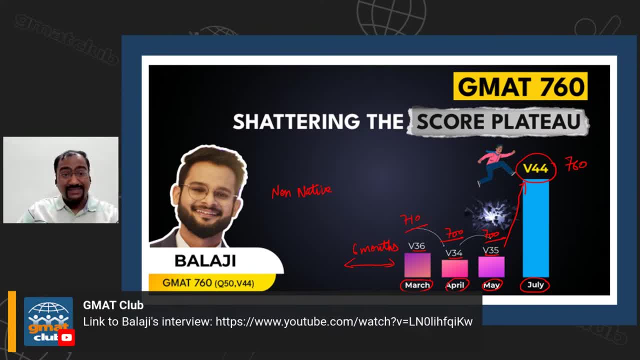 in that way, he was able to do the right thing. he was able to do the right thing in his experience and he was able to do the right thing in his case study and you can check out his interview in depth. if you want to take more clues from his case study, you can check it out as interview. i've shared the. 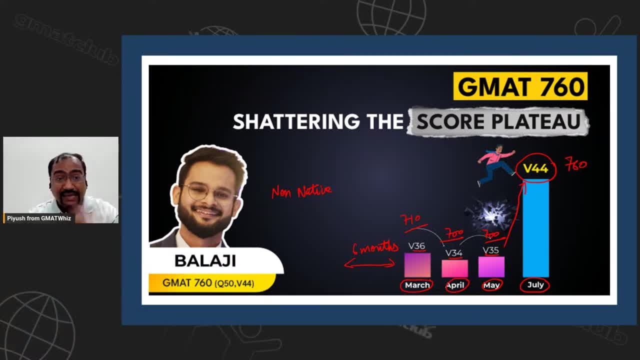 link in the chat. you can obviously do that. uh, check out his interview later on. but the main thing which i'm trying to talk about over here is that he focused on identification of his weak areas and the study buddy was able to help him. a study guide- sunita man in this case- was able to. 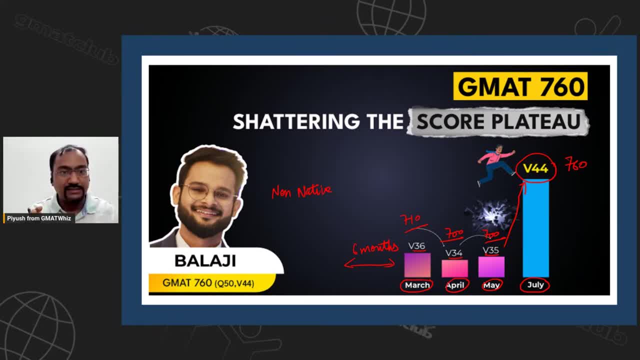 help him, because what was happening with him was it was not that he didn't knew what the meaning, But the problem was there was no consistency in the approach that he was using In one question. he will do this in another question. he will do that. he will look at. 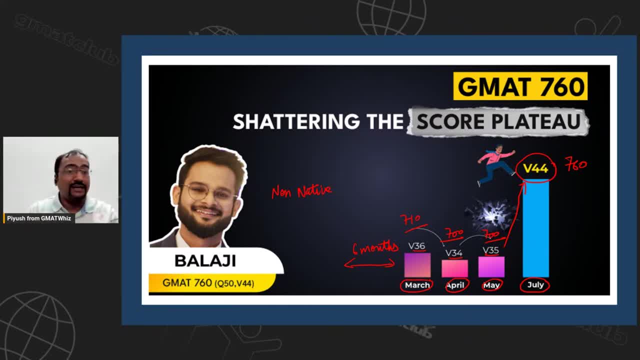 a sentence correction question, he will see. if it is a very long sentence he might think of the meaning. If it is a very short question, he will do the splits. So there was no consistency in the approach And there were other things also which were a bit of a problem in CR. basically there, 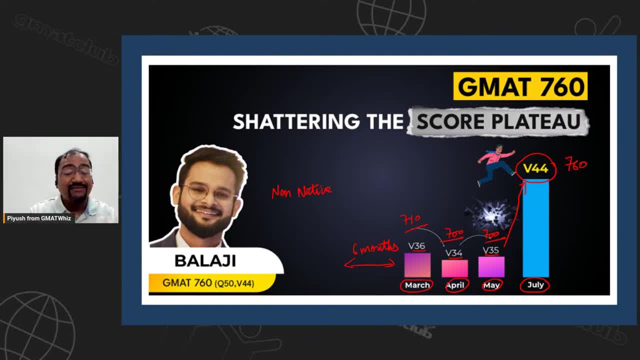 were more problems in his case, So obviously there were areas which he was not aware of he did not know how to tackle. But a study guide like Sunita ma'am- in this case with him he took the tutoring sessions- really helped him trace the way out. 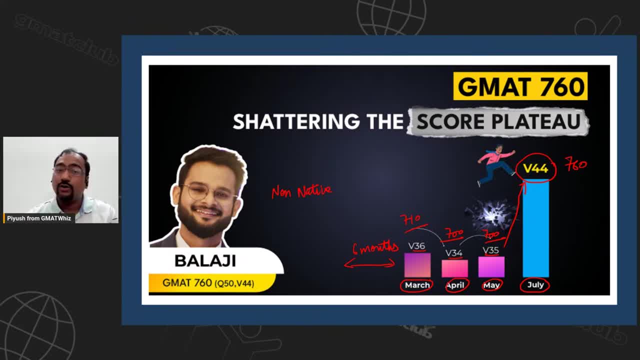 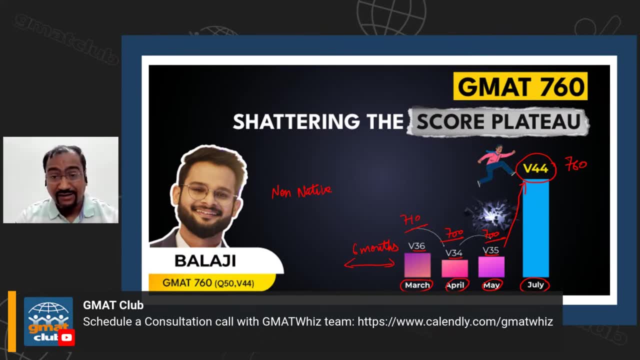 So if you are thinking that you are stuck in a score range, stuck in a score plateau, do reach out to us. we can definitely help you. you can schedule a call on my calendar using this link, basically, and we will definitely help you out and we have helped out many, many 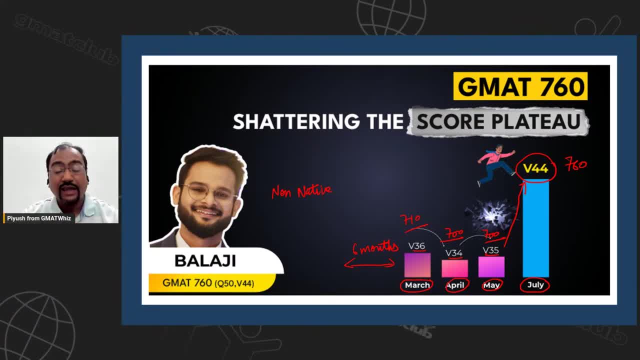 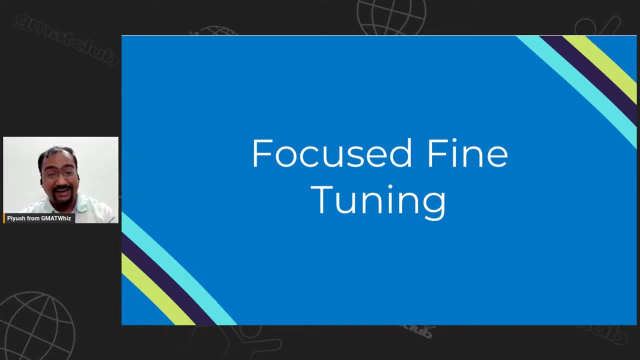 people to improve their scores in 20-30 days also. So make sure that you get a right study guide, a right study guide. The next tip for you to improve your GMAT score is focused fine-tuning. So even if you are practicing- I asked this question, a lot of people said that I practice- 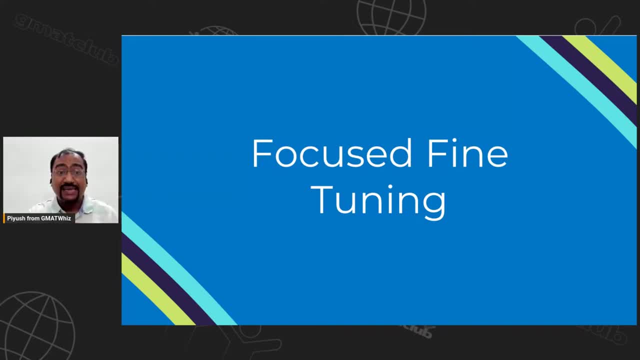 practice, practice. Do the practice in the right way. Some of you were saying error logs help. that's very important. contain an error log. The idea is that when you are doing practicing, you focus on your weak areas, not just doing. 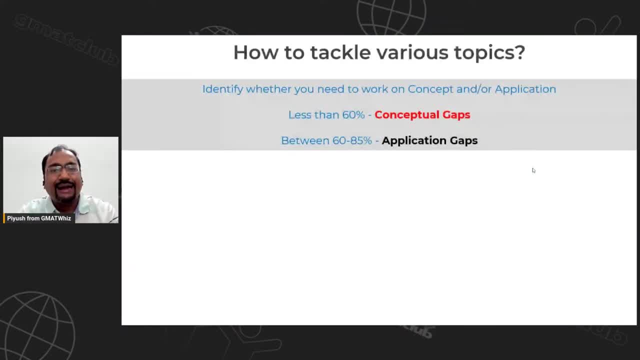 everything. So, when you are working on fine-tuning, identify your weak areas and categorize them into right buckets. So there could be areas in which you are weak because of your conceptual understanding, And then there could be areas in which you are not. 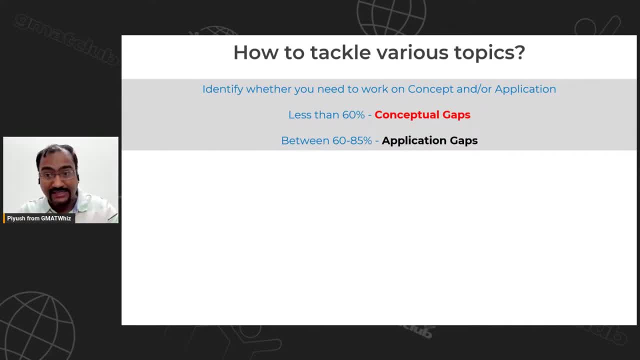 Okay. So there could be areas in which you are weak because of your application, application methods, basically. So I do identify: why are you weak in a particular area? So if your score, one way to look at it is that you can benchmark, basically with respect. 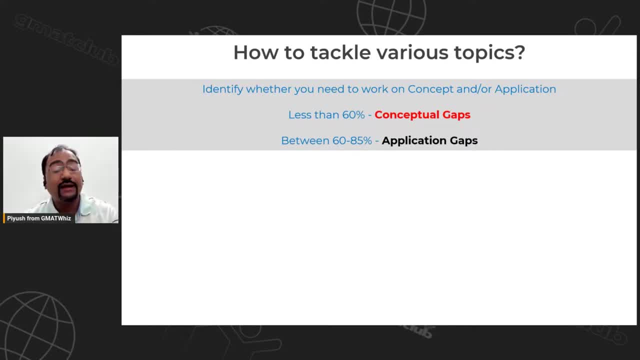 to scores. So if your score is less than 60% in a topic, it's possible that you have conceptual gaps in that topic and that's why your score is weak. On the other hand, if your score is between 60 to 85%, most likely you don't have concepts. 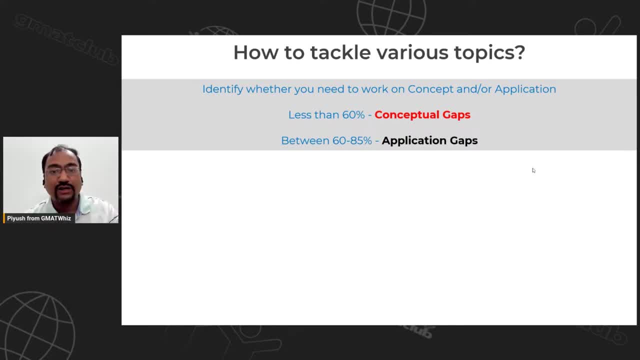 gap. you have application gap, So the areas in which your score is less than 60%: For those areas you need to first work on learning the concepts and the formulas properly. Okay, You need to learn the concepts thoroughly, understand them well, revise them well, because 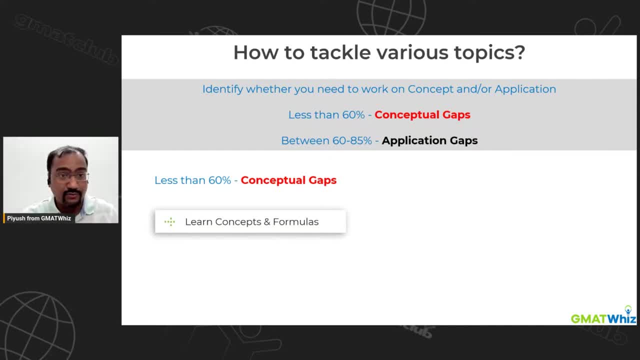 if you have concept gaps and you continue practicing, it's not going to help you improve your score. So learn the formulas again, revise the formulas again, then learn how to solve questions and you can then do 15, 20 questions, Like you will need to do more questions here to improve your understanding. 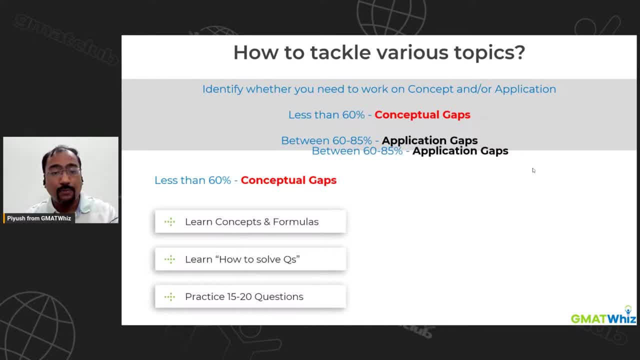 On the other hand, in the areas in which you have application gap, there is no point in doing concepts again Like you'll be wasting time. Okay, So identify the right method, learn how to solve questions in a methodical fashion And, after doing that, practice 10 to 15 questions, and when you're doing this practice, you do. 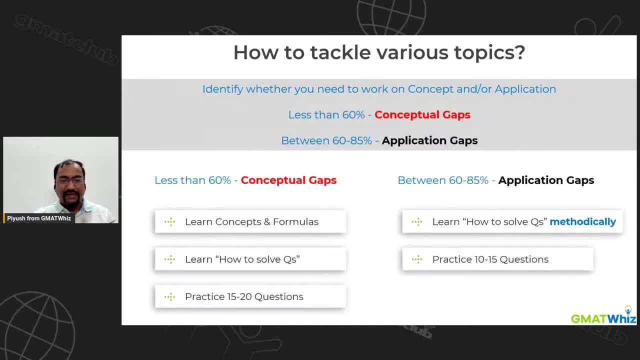 this practice in a systematic fashion, Like, instead of doing all questions at once, do one question at a time and then ensure that you check the solution properly and then only move forward to the next question. Okay, So do one question at a time, check the solution, check whether you stuck to the right method. 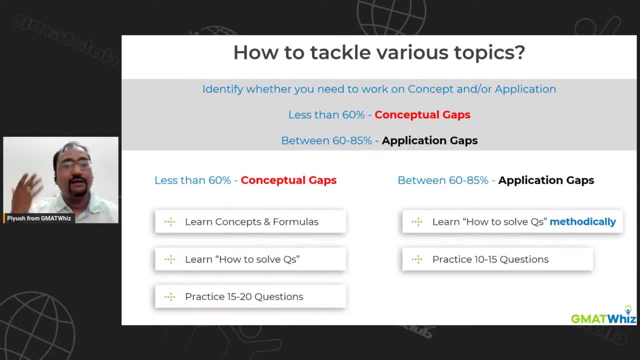 or not. If you did not stick to the right method, Then take up like the differences in your approach. then take up the next question. So at least do 10, 15 questions, one question at a time, and improve your approach over that. 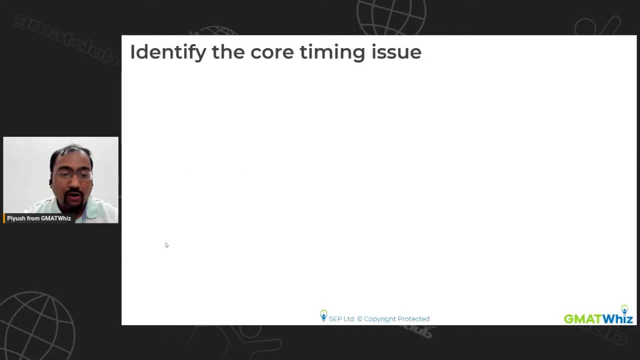 Okay, That's something which is very, very critical for you. Now, also, one more issue in your fine-tuning could be a timing issue. So I talked about two issues: concept and application, but it could also be a timing issue. 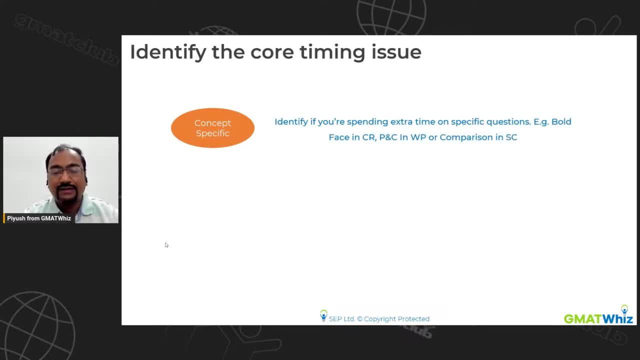 Now identify the core timing issue. Is it because of a concept? Is that like a concept? Is it because of a concept? Is that like in specific type of questions, Let's say critical reasoning in bold-faced questions, you are taking extra time. 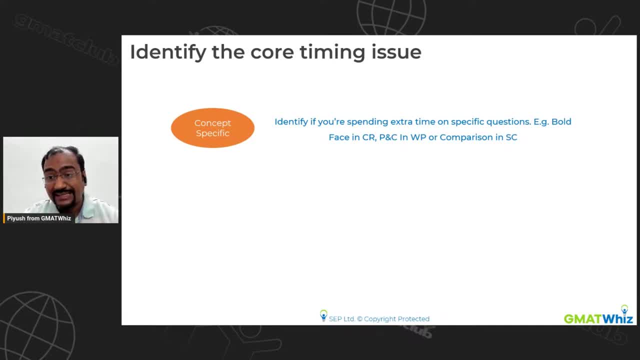 Or it is combination- combination questions in word problems that you're taking extra time. So if it is concept specific timing, working on concepts would help, or is it application related timing issue? Like, if it is application related timing issue, it will happen with the entire module. 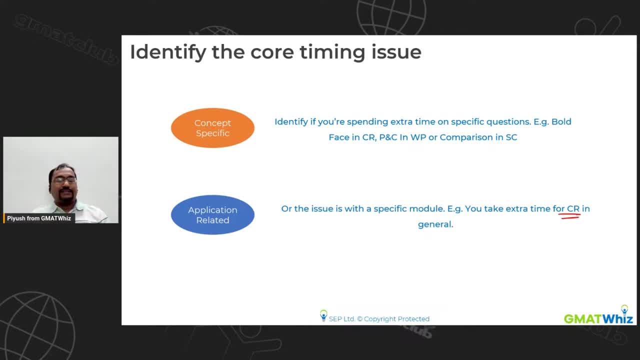 Like, for example, in CR in general, you'll end up taking extra time. Like in most of the topics in CR, you would end up taking extra time. end up taking extra time. if that is the case, you need to change your approach for critical reasons. 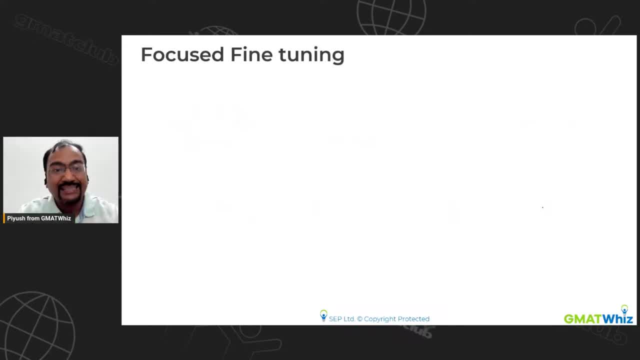 the approach that you're following is not working out for you. okay, that is very, very important. so what i'm talking about is do focused fine tuning and when you're doing focused fine tuning, devote 70 percent of your time on your weak areas only, so if you're doing, let's say, 10, 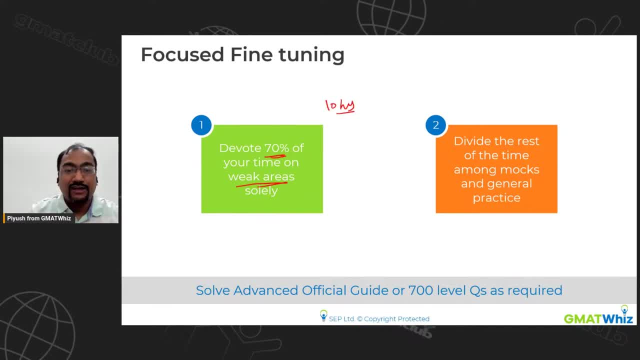 hours of preparation. don't just take sectional tests for content verbal in those 10 hours. that's a very wrong thing to do. out of this 10 hours, seven hours of effort. you should focus solely on your weak areas. let's say you've identified: boldface is a problem, pnc is a problem, and let's 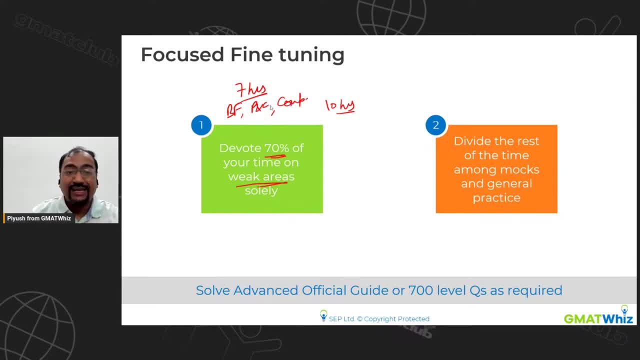 say, comparison is a problem in uh, in, these three are your weak areas. spend seven hours on those out of the time. the rest of the time, the three hours which are left with you, that you focus on general practice, okay, and also solve advanced official guide question or 700 double questions. 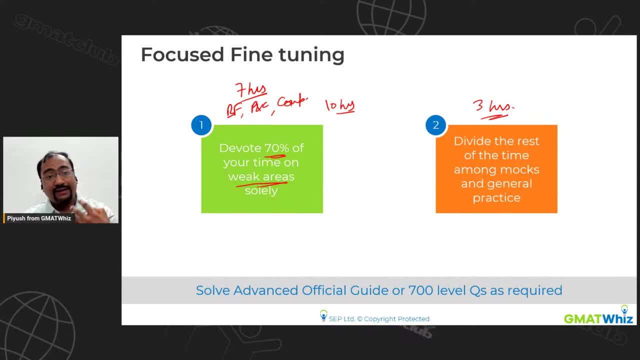 as required. obviously, if you are very weak in a particular topic in in that case, if you you just jump to 700 level questions right away, it won't make sense. you have to first work on easy and medium questions, as i was telling you at the beginning of the session. also. 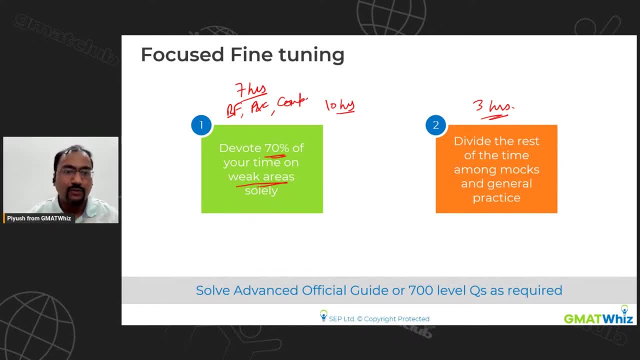 and if you are comfortable with easy and medium questions, then obviously you can jump to the 700 level questions and you can start doing the advanced official. okay, and if you have any questions, guys, till this point, feel free to ask me. i'm more than happy to take up your questions. 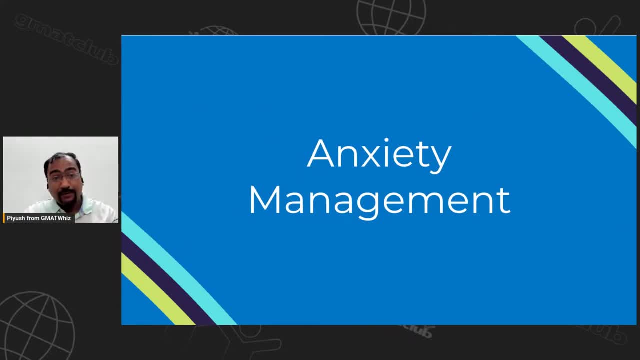 uh, please share your thoughts, okay. the next thing which is very important for you to improve your score is the test day delivery. you have to ensure that you deliver on the day of the test and for that anxiety management is very important, and i tell this to a lot of people that gmat is not. 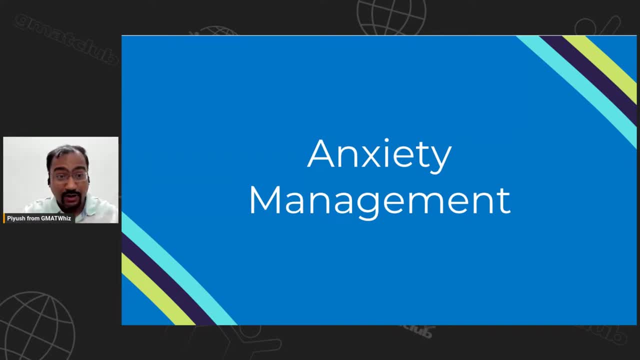 just the test of your capability or your potential of getting content verbal questions right. it's also the test of your anxiety management. people who can stay calm under pressure situations can actually manage to get a good score on gmail. now, how do you improve your anxiety and like? 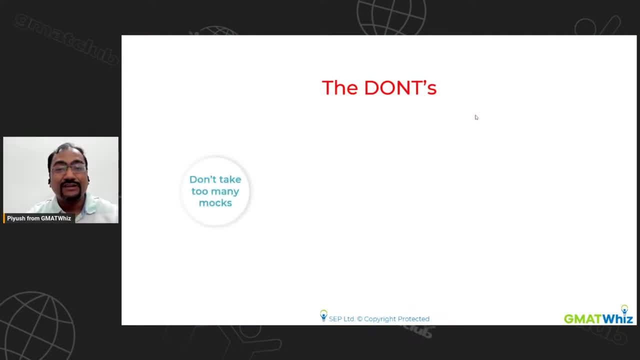 take care of your anxiety rather not improve your anxiety. so one thing is that certain things you should not do, don't take too many marks. i've seen people taking up 15, 20, 30, in fact 50 marks on g for gmat. don't do that. gmat is an adaptive test. just taking more marks is not. 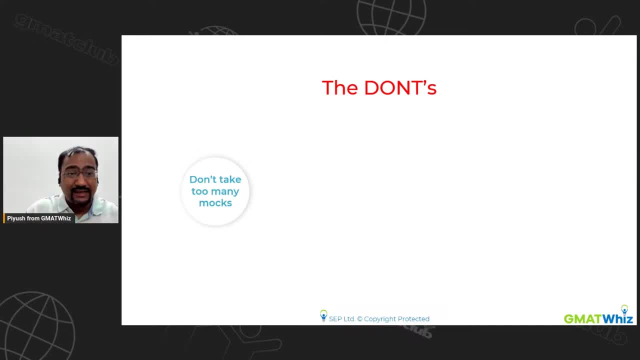 going to help you. you need to work on your weak areas first. even if you have two or three weak areas, or like like in a particular module- let's say in sentence collection- you have two, three weak areas, you will end up scoring low. so instead of using the marks to identify your weaknesses, 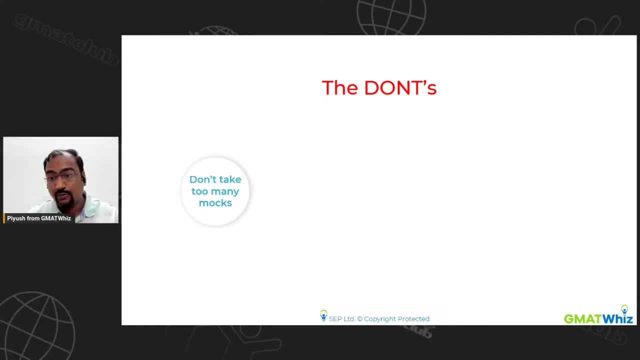 use practice tests, small tests. work on them first. don't take too many more, basically okay. then don't keep a target number of questions for a day. another big mistake which a lot of people do is that they target that okay every day. i need to do 30 questions now, if you. 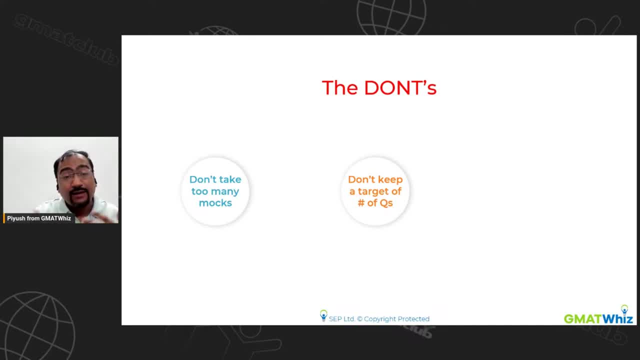 want to keep a target, take it a small tag, take it as a small target or spend more time on solution review part. if you keep a target only of number of questions, your focus will be only on solving more questions and, uh, on days when you're not having enough focus or attention, you will still. 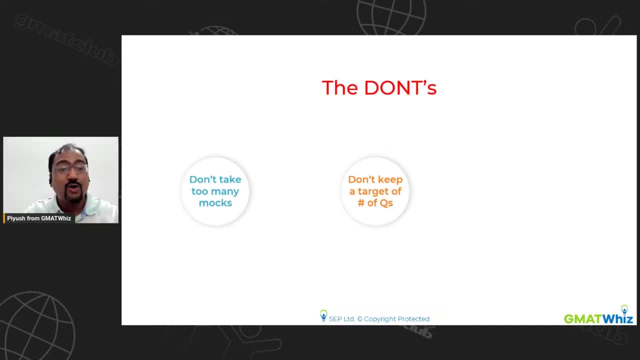 go ahead with solving more questions, get a poor score. your anxiety will only increase because of, and don't increase, your study time. that's another mistake which people do. when they think that okay they are becoming, they are coming close to the test day, they start putting in more effort. 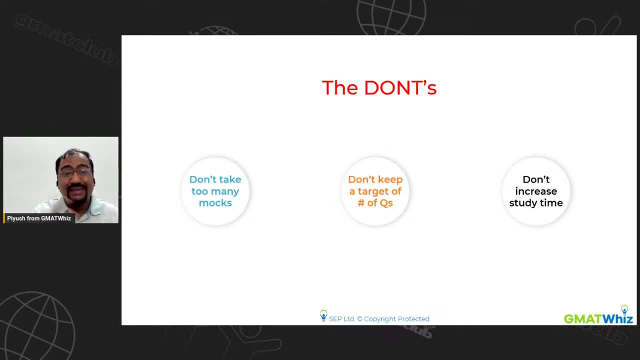 in many cases that becomes counterproductive. so don't increase your study point time till the point that you're not even able to sleep properly. don't make that. make sure you give yourself enough rest before the test, and that's very, very critical. i always recommend the last two days before the test you should ideally not study at all. okay, the do's. 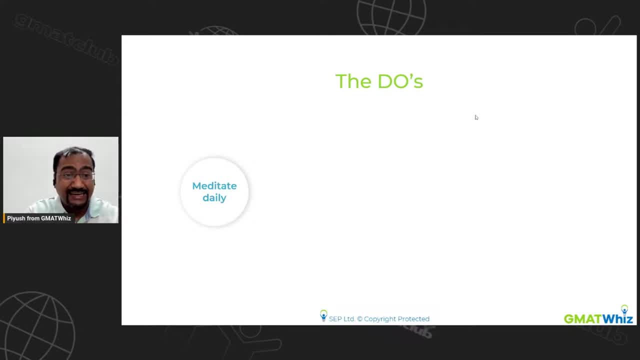 daily, at least if you are. your test is in the next 10 days. you need to do that. ideally, you should start meditating earlier, at least in in that case, if you have a like in general cases, if you have anxiety issues in your previous tests also, then this meditation should happen much more. 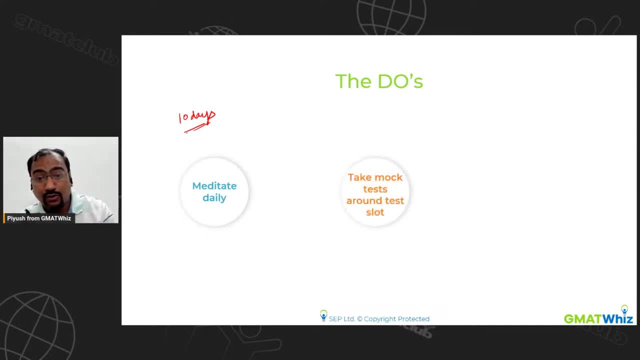 earlier, meditate daily. that's very important. they don't uh take mock tests around the test slot. so if you, let's say, have a test slot in the afternoon, then you take the marks only around the afternoon. make sure that you're comfortable during that time. you have the maximum level of attention. 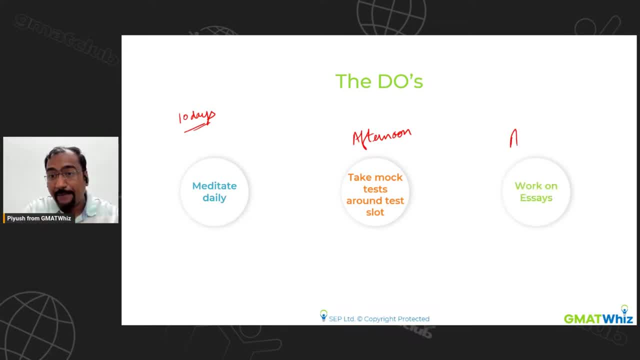 at that particular time and also start working your application. start working on your essays, because when you start working on your essays you know that you are moving forward. otherwise sometimes you feel stuck with gmat, that gmat itself is not happening. when will i get time for my application? so if you start working on your applications, you will feel much more uh. 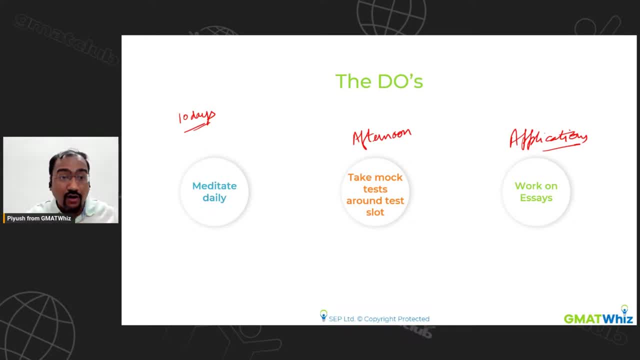 like confident. you will feel much more involved. you will feel motivated to get gmat out of the way as well. so start working on your application alongside. don't delay it unnecessarily. so that's how you can manage your anxiety, and that's all that i wanted to talk. 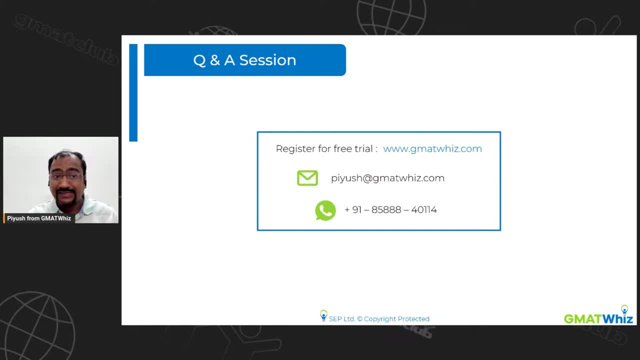 about in the session. i've tried to bring up very important points around six different tips that i have talked about. those of you who joined the session late do watch the recording. you will be able to understand a lot about gmat. so if you have any questions now, i'm opening the session for. 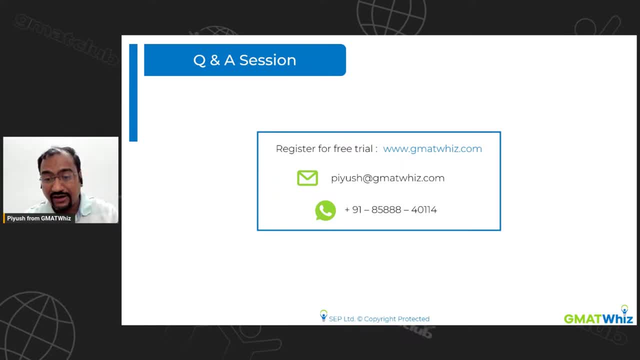 open ended query. now. if you have any questions whatsoever, feel free to ask me. right now. i've also shared uh my contact number, which is my whatsapp number, over here. so if you can, if you want to connect with me on whatsapp, you can drop me a text, but the better way would be to schedule a call on my calendar. if 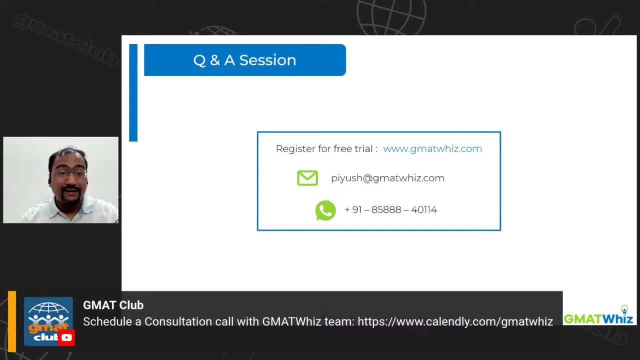 you want to connect with me. i'm sharing the link for the same over here and you can also reach out to me on my email. and if you really like this session, do give it a like, do give it a thumbs up. as i said, i have a target of 50 likes. let's see if you can get 50 likes to this session and 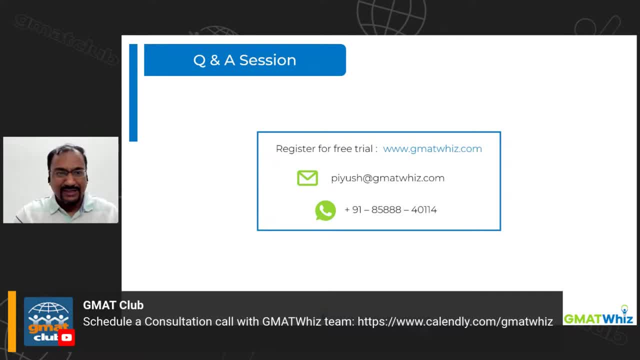 if you do, uh, you'll see me very, very soon again. i'm doing this session for after almost a month and a half, so i'll be coming back again, and next time probably. a lot of people are asking about gmat focus. gmat focus. i'm planning to do another session on gmat focus study strategy as well. 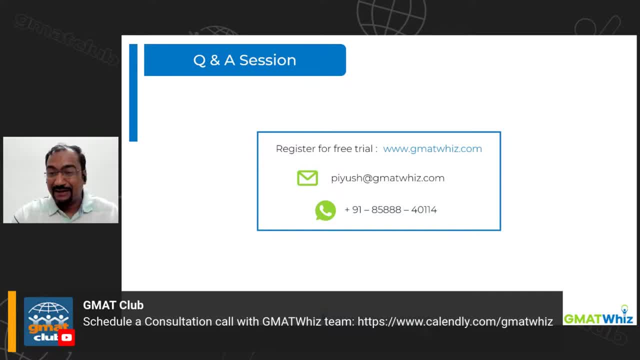 so, uh, let's get more likes on this and i'll be back with gmat focus study strategy session as well. okay, mofasil has a question. he says i feel nervous with large verbal questions. again, understand it this way: if it is a large verbal question. 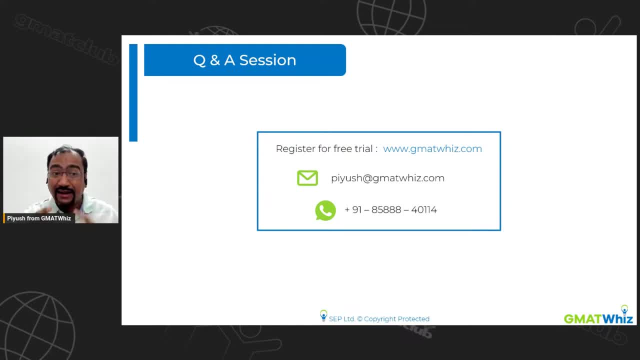 you are not the only one getting it. there are other people also who are hitting it, and gmat has experimental questions also, so they have tested the difficulty level of the question after doing a lot of experiments. so when you are actually getting a large question, just don't. 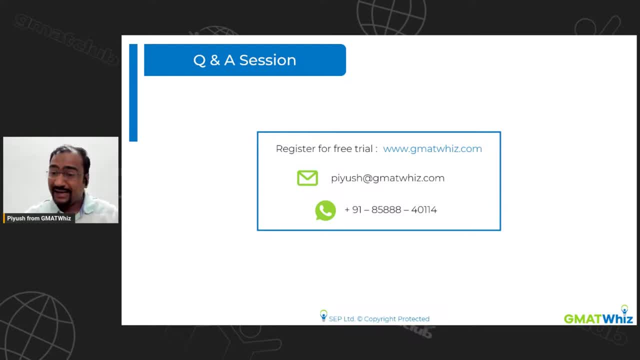 panic because of that. it could be an easy question also, and if it is not an easy question, it's a hard question. you should actually feel more happy. i feel happy when i get a hard question. can anyone tell why? why i feel happy when i get a hard question? any idea, mofasil. 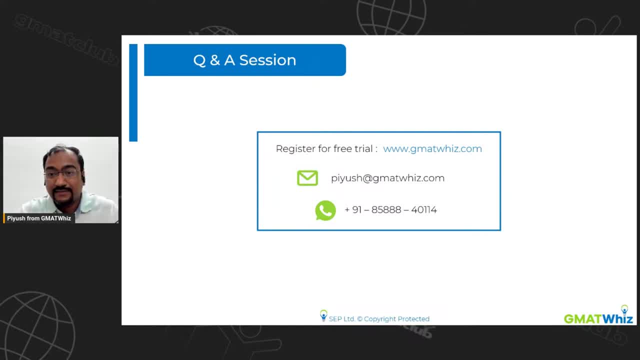 why should i be happy if i get a hard question? any ideas and thoughts? anyone else else has any questions? please feel free to share it over here. happy to take your questions up. guys have any idea why you should feel happy when you get hard questions. really want to hear your thoughts here why you should feel happy when you get hard questions. 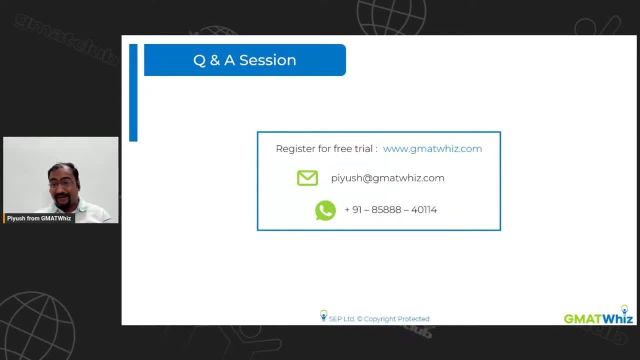 why you should feel happy when you get questions because your score is in high level. your score is in upper level because you're performing well. it's not just for learning opportunity community see, understand it this way. i'm taking a test to get a high score on gmat, right. 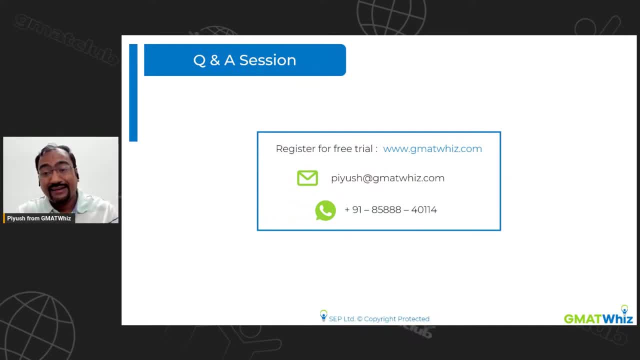 if i'm not getting hard questions, i'm probably not getting the high score. hard questions mean i'm actually going in the right direction, so that's something which is very important for you to understand. okay, so please don't make this mistake: hard questions. if it is a hard question, you should feel happy. 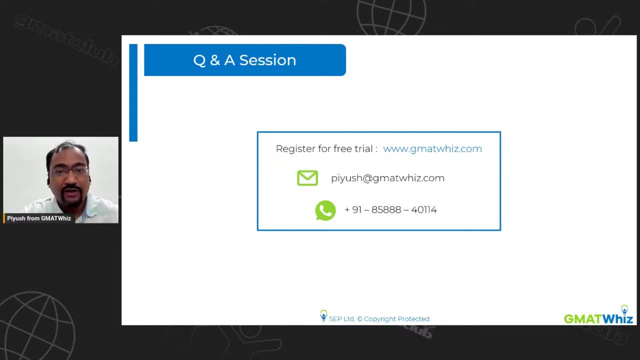 okay, uh don't let's say: should i opt for focus edition? see, there is a. there is a reason why, like at gmat means we are recommending that you should not uh go for the gmat focus edition if you are looking at this year intake and there is a proper rationale for that. so i'm just going to. 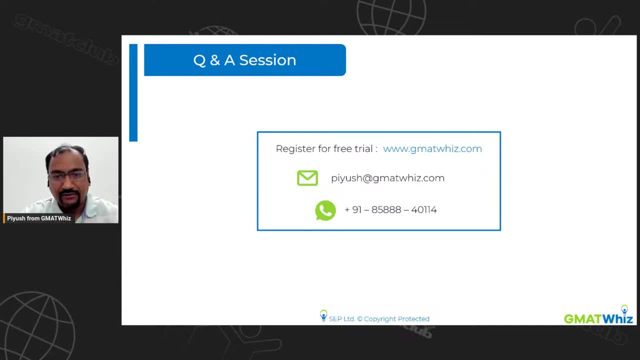 share the webinar that i have conducted on the same and that way you will be able to uh basically get a better understanding of it. so i have actually covered a lot of comparison. i have done a very uh good comparisons video uh between the gmat current and gmat focus so you can go through. 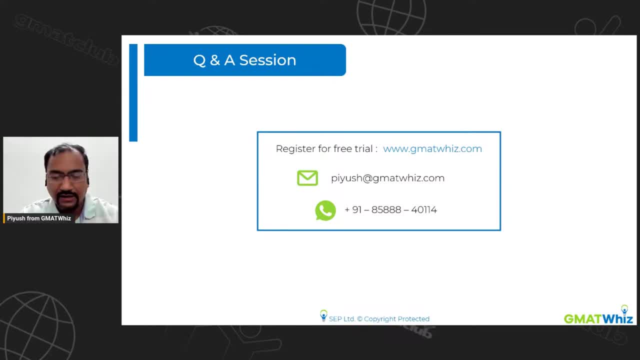 this video should you go for. let me just type the link so you can go through this video to understand this better and if you have any questions, feel free to connect with me again. uh, on the email id that i've shared and the contact number that i shared. so this is the video that you can watch. 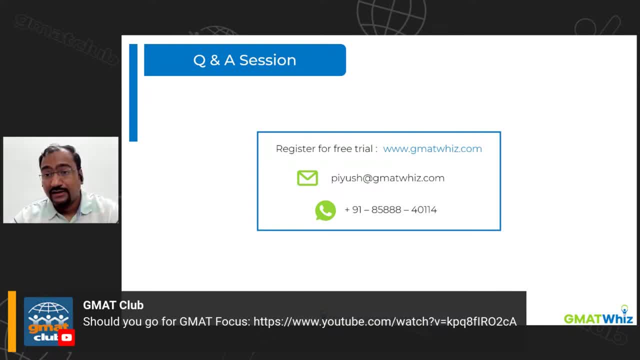 to understand whether you should go for the gmat. focus on that. so you should go for it in certain cases. in certain cases you should not. okay, gargi is the point that he says. i've been giving quant sectional marks recently, but each time i'm getting the same score, i'm not able to cross that mark. but when i try to solve the same 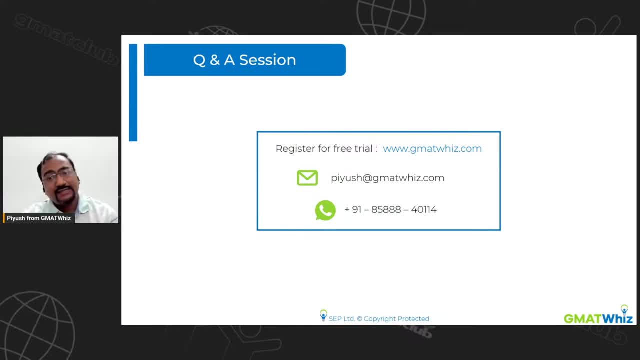 questions later i'm able to solve. so, gargi again. there could be multiple reasons why this could be happening. one reason about the most probable reason is that you are pushing yourself too hard. when you're taking your mark right, you're probably uh like, uh overthinking, or you are. 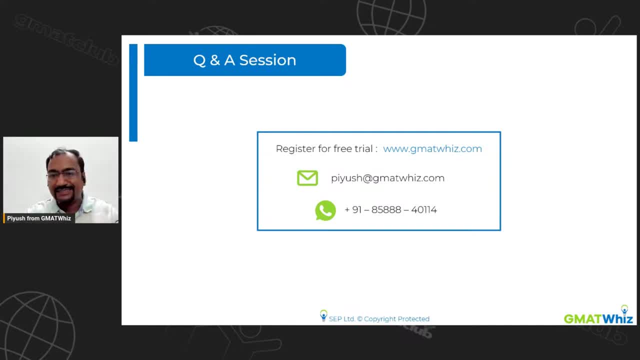 let's say, not overthinking technically, but you are rushing through the questions, then you're not reading the complete questions then, or you're rushing into solving the question. you're reading the questions then, but without thinking about the steps that you need to take, you're just jumping. 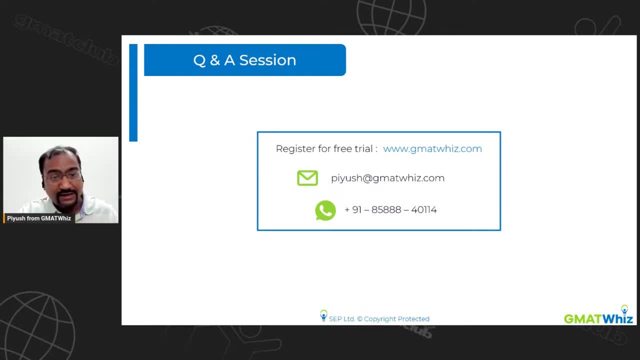 into solving the question, and that's when you end up taking more time. so that could be one reason. second reason could be that you're probably not practicing under the time environment. your methods are not sufficient to get you to solve those questions in that time situation. so you 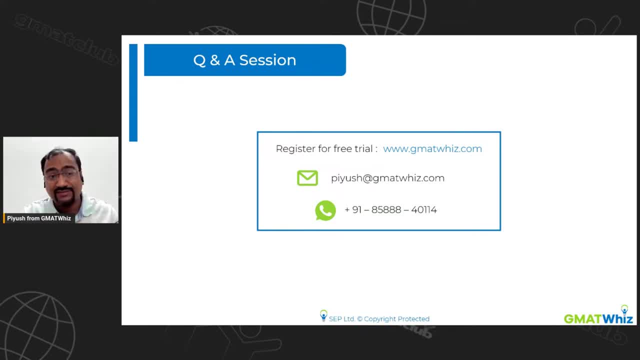 might have to look at improving your method. so it's most likely one of these two things which i can think of. probably, so work on this, and that should really help you, okay, so thank you so much, guys. i don't see any other questions for now, but if you have any questions, 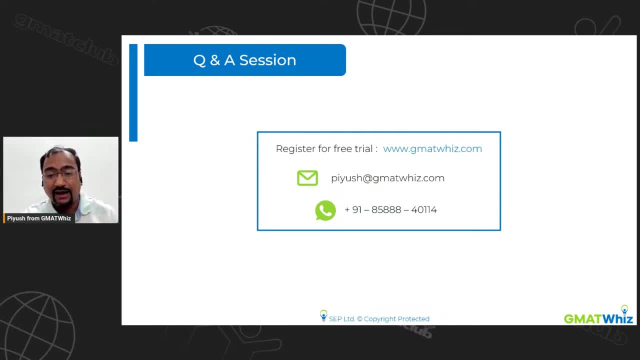 guys for me, feel free to reach out to me. i've shared my uh contact details on the screen. you can check out. uh the uh like my calendar. also, book a slot on my calendar. most likely not find a slot for tomorrow because my slots generally get occupied for one or two days in advance, but